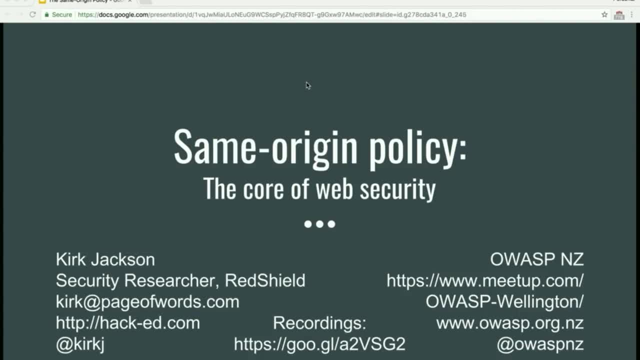 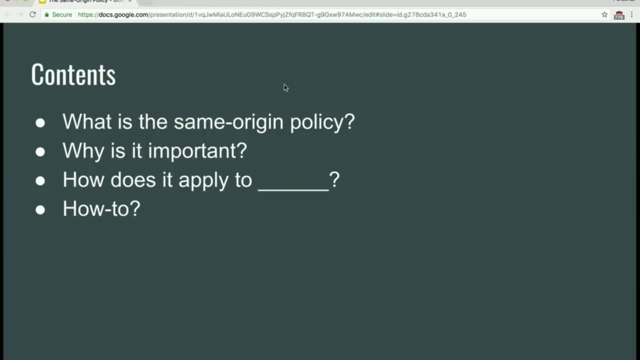 But hopefully this will kind of bring it all together in a cohesive format for you. So this is what we're going to cover: What the same origin policy is. Why is it important to web security? How does the same origin policy apply to blah? 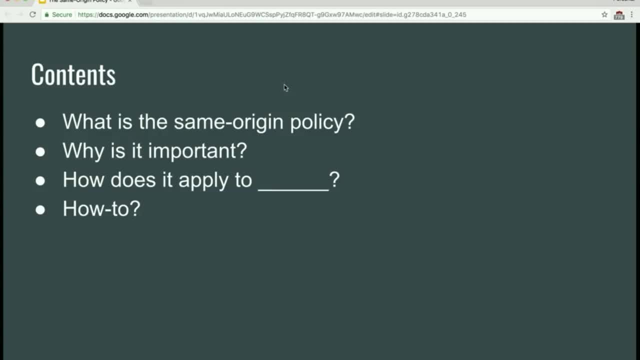 Where blah is one of the many web policies, What type of technologies that you'll use And how do you get around the same origin policy, or how do you do things around the same origin policy, Maybe to embrace and extend the restrictions? But first, of course, before we talk about the same origin policy, we need to talk about what is an origin. 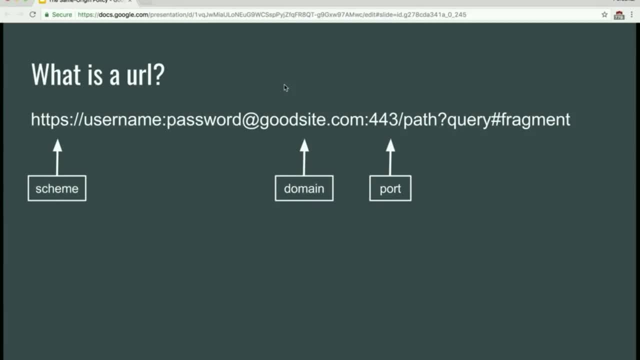 And you've probably seen one of these before. It's a URL. It has some pretty familiar parts that you'll be used to. There's the scheme at the beginning: HTTP or HTTPS Or possibly even FTP or Gopher. You often don't see a username colon, password in URLs these days. 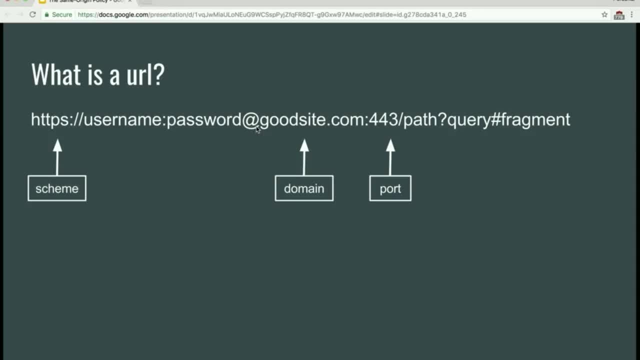 But they used to be used more often- Then an at sign and then the site's domain, A port. If it's HTTPS, you don't need to put it, It defaults to 443.. Or if it's HTTP, it defaults to 80.. 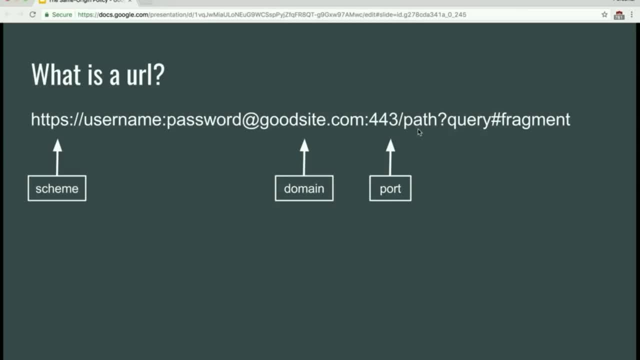 And then there's the rest of the URL, So the path, the query string and any fragment on the end. Now an origin looks at just three of these parts: The scheme, the domain and the port, And together that tuple makes up the origin. 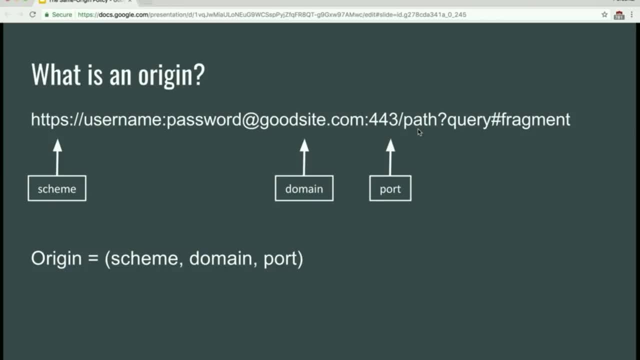 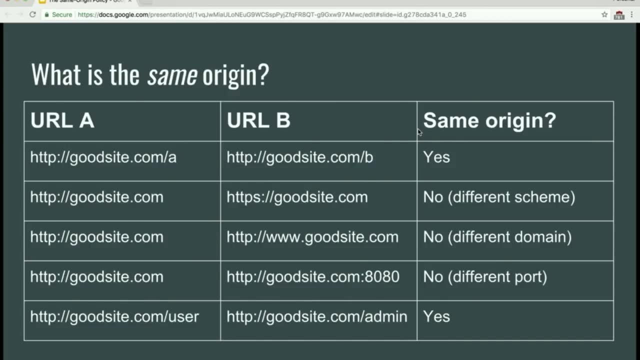 So if two web pages have the same scheme, domain and port, then they're both the same origin. So just to illustrate that in a tabular form, let's look at your pairs of URLs and see if they're in the same origin or not. 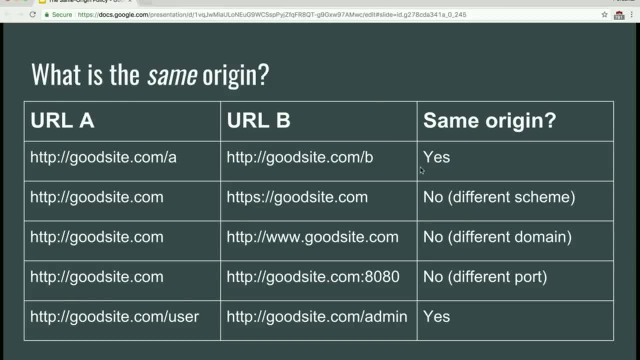 So the first row, those two are in the same origin because they have the same scheme, HTTP, The same domain, GoodSitecom. The port number is 80 for HTTP, so that's implied. So therefore they are the same origin. 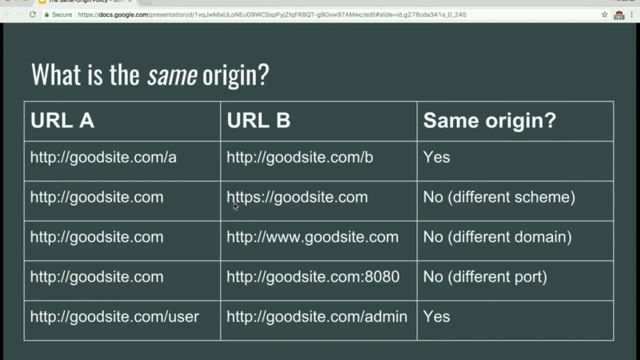 Now, the next two are not the same origin because one is HTTP and the other is HTTPS, And likewise row three. they're not the same origin because the domain name is subtly different: One is GoodSitecom and the other is wwwGoodSitecom. 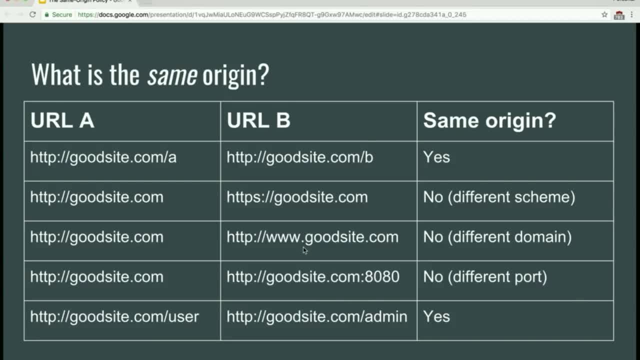 Row four is another example of two URLs that are not the same origin, even though they might appear that, because the second one uses a different port: port 8080.. And lastly, another example of two URLs that are the same origin because they have the same scheme, the same domain name and port. 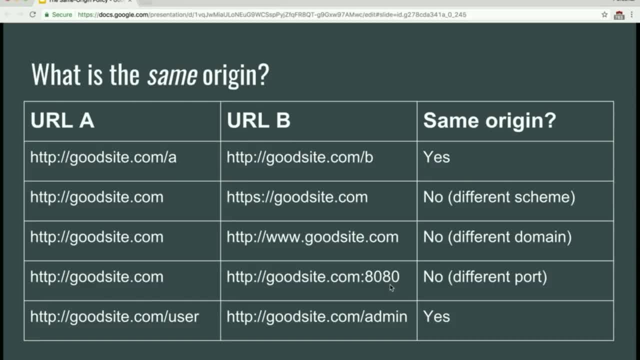 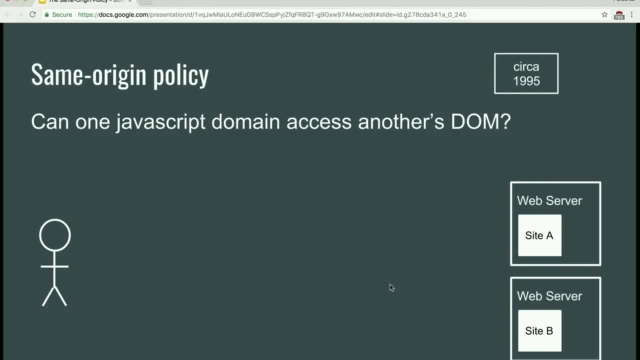 The only thing that's different is the path on the end of the URL. So now we understand what an origin is. let's talk about the same origin, The same origin policy, And to understand this we have to go back back way, way back to 1995,. 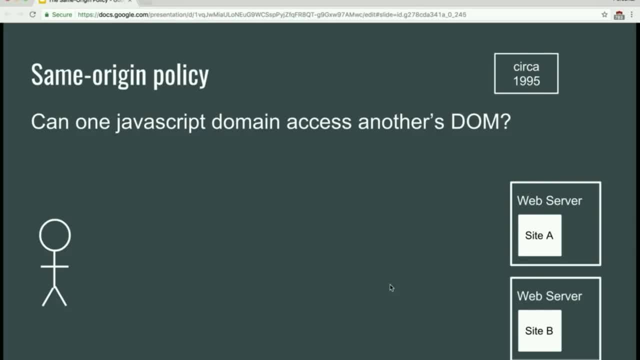 when Netscape was inventing cookies and forms and JavaScript and embedding them in one of the early web browsers, They came up with this concept of a policy that specifies whether one JavaScript domain can access the document object model of another JavaScript domain. So to put this in terms, 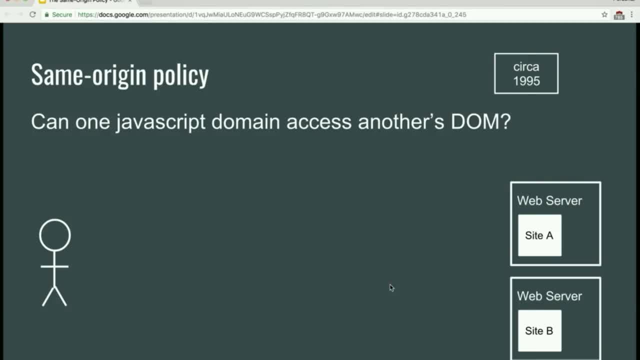 we understand one website running in a browser whether it can access the data of another website running in the browser, And let's look at that in a pictorial sense. So we'll display the browser as a giant box. So the user is using their browser. 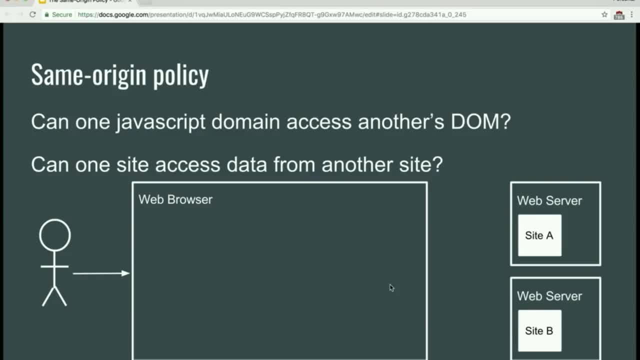 and then the browser is going to be talking to web servers somewhere out on the internet. So when the user enters a URL to go to site A inside their web browser, a context is created to run site A's JavaScript. It has access to the DOM of site A. 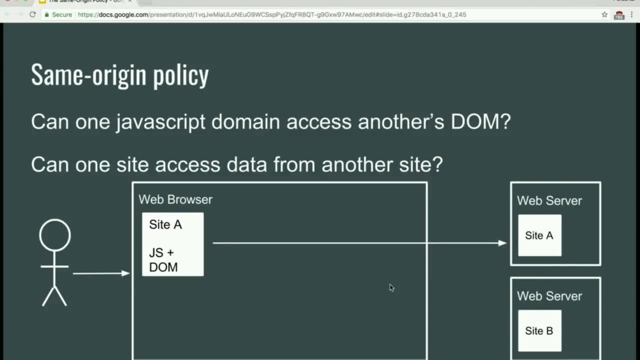 and usually it'll display the HTML or display the web page in a frame or in a window or in a tab. If they go to another website in another tab, a new context is created in their browser for site B, which is loading the files off the site B web server. 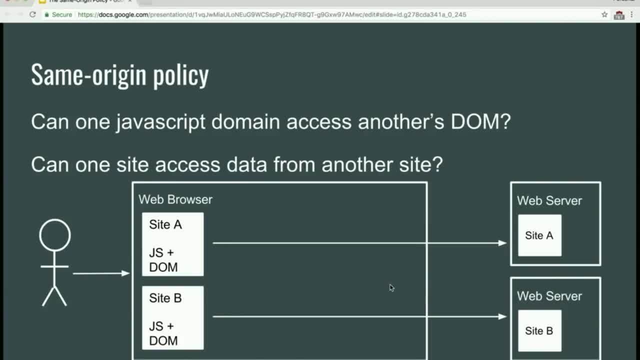 And that has its own JavaScript, its own DOM and its own context, and it's separate from site A's context. And the crux of same origin policy is: can site A- that's running in your browser- access the data of site B, also running in your browser? 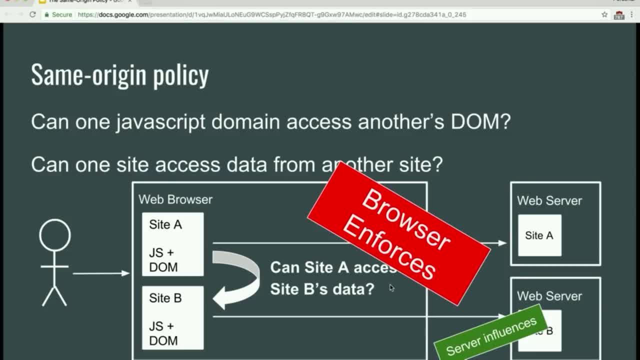 So the interesting thing about this is that the web browser enforces the same origin policy around whether one site can access another, And it's not actually the same as the web server's job to enforce this. It's the web browser. The web browser is the one that's running websites. 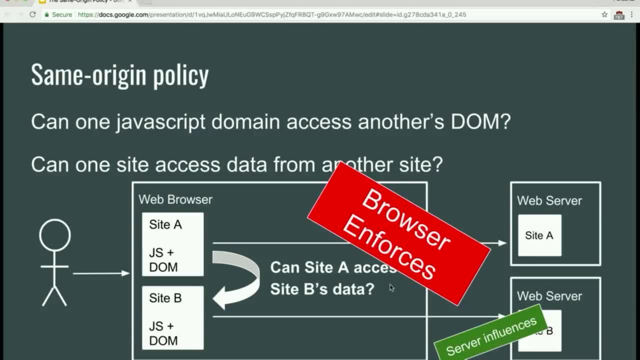 in different contexts on the user's machine and isolating them from one another and protecting them from one another. So it's the web browser that lets you load internet banking in one tab and Facebook in another, And the web browser is what stops Facebook from accessing the data in your internet banking. 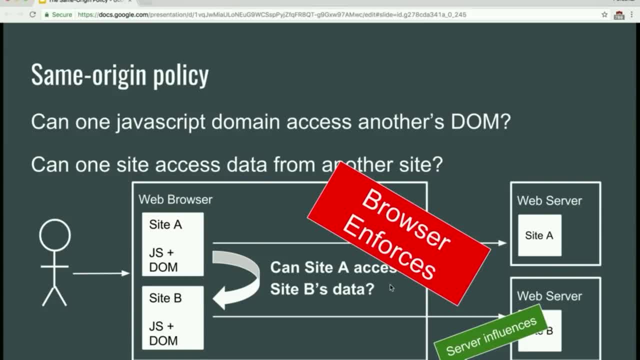 and transferring funds. So I guess that's a core thing to understand- is that the browser enforces the same origin policy and restricts access from one site to another. Now your web server can influence this. We'll talk a few ways about how you can do that. 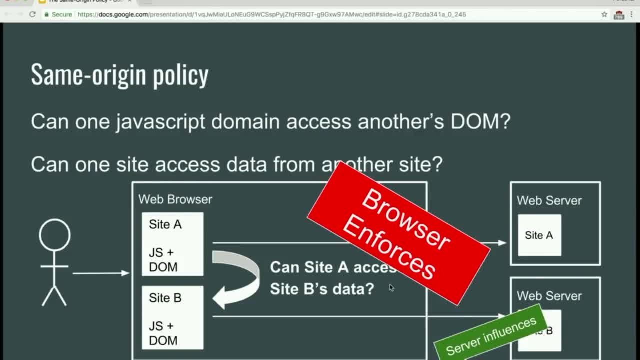 through the course of this talk, But really it's the browser that enforces these rules, And we'll also come back and talk about what happens if it's not a browser that's accessing your web server. What if it's a mobile client or your site is an API of some sort? 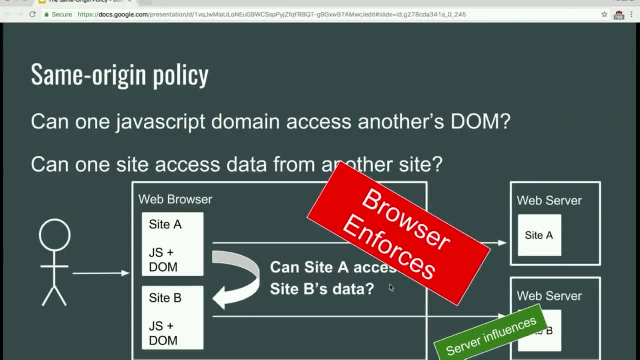 and people are just calling it from a Perl script. Does the same origin policy apply then? And no, it doesn't. If someone writes a Perl script, they can come up with whatever rules they want. They can access whatever data they want, as long as your web server returns it to them. 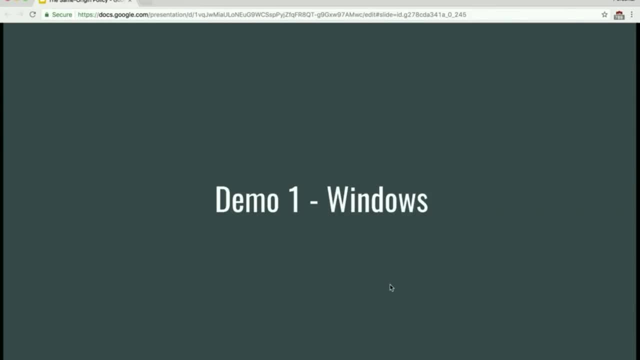 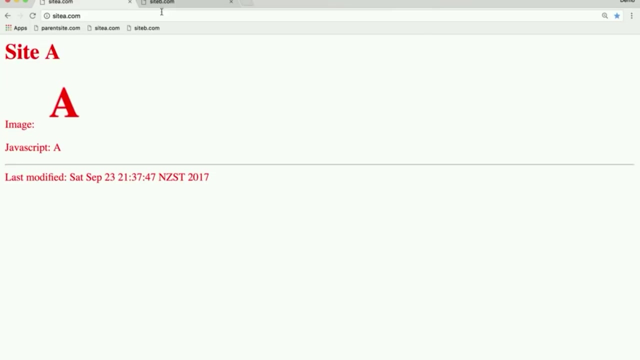 they can do anything they want with it. So our first demo is going to look at what Windows can do to each other. So to show you this first, I'll introduce our demo sites Now. they're very, very good looking. We've got siteacom and sitebcom. 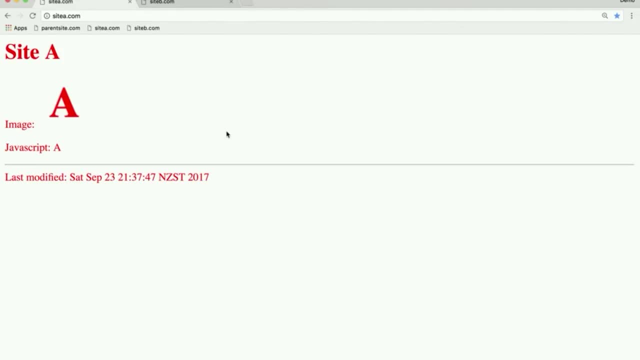 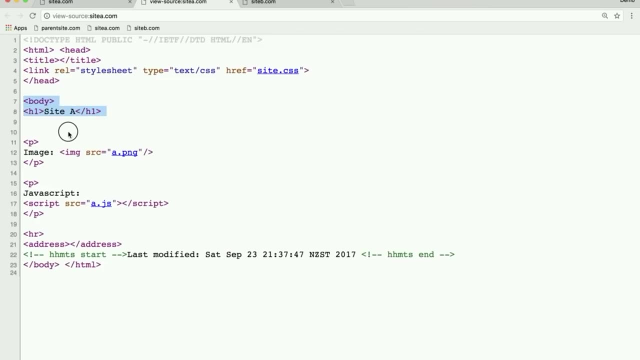 You'll notice they're different colours to make them stand out from each other. Site A is red, site B is blue. If you want to look at the source of the site, it's pretty simple. There's some HTML printing out site A. 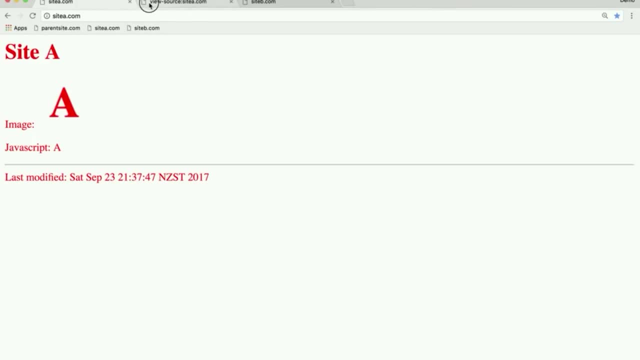 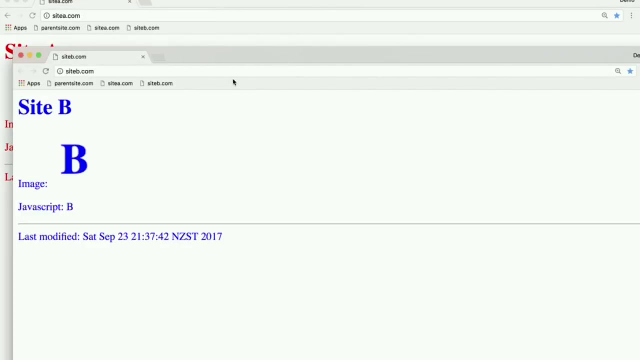 There's an image which displays in A And there's some JavaScript being loaded And it looks like the JavaScript is also printing out in A. So what do we mean by Windows? Well, here we've got two different tabs in our browser, effectively two windows. 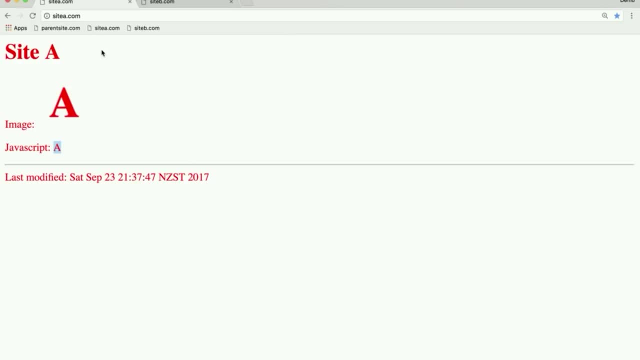 And, as we know, they're running different instances, different contexts for those two different websites. When we look at our website, we can inspect the DOM in Chrome's developer tools and we can do in the console anything that the JavaScript can do on this site. So this is a good way to kind of 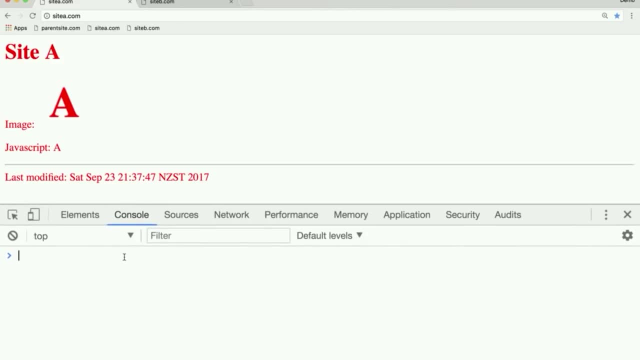 prototype and figure out. would JavaScript be able to do that when it's running on this site? So first let's look at the document in the current window And you can see HTML in that document. So you can do documentlocation, you can change the URL. 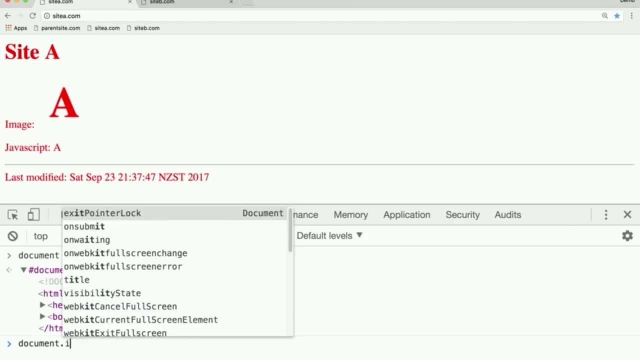 you can look at items within the document, you can change the document altogether, And there's also a window object, and the window has a bunch of different properties on it that affect the frame of the site itself. So the first thing we want to do is 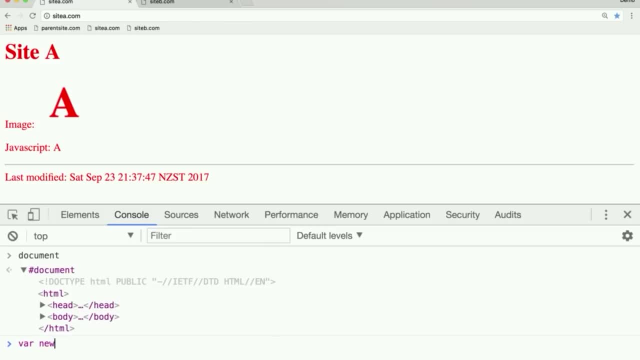 let's open a new window. So this is pretty standard boilerplate code that you've probably done before. And let's from site A. let's open another window with site A in it. We're going to call the next window, write, which is the second parameter. 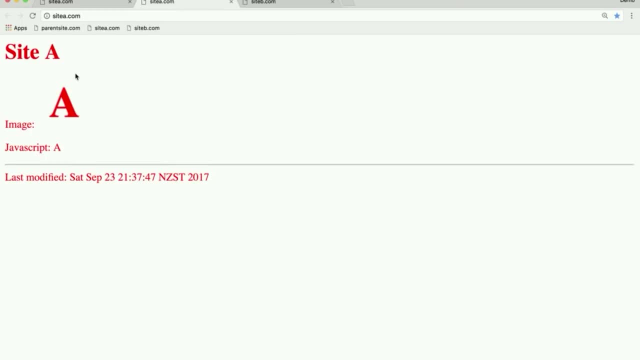 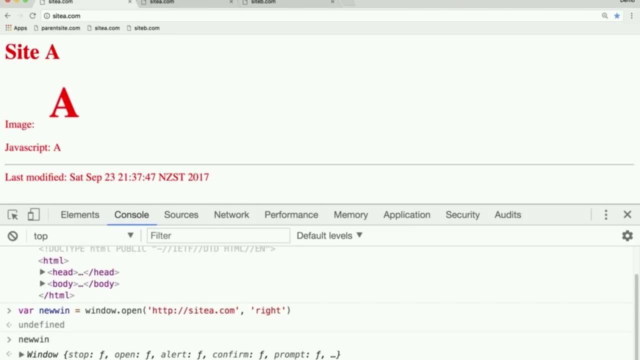 And you see that the browser just opened up a new window. This window's also got site A in it, And if we come back to our first window, our variable is now defined with a reference to the new window that we've created. Now it's interesting. there's no way. 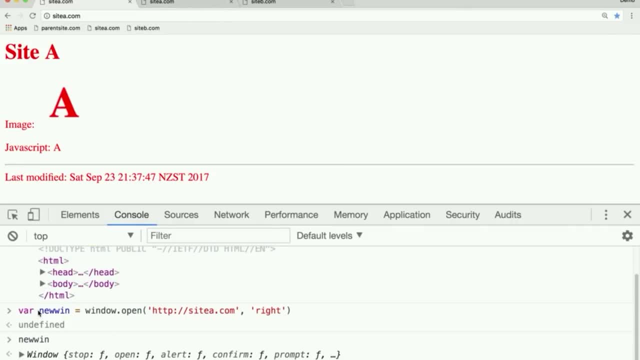 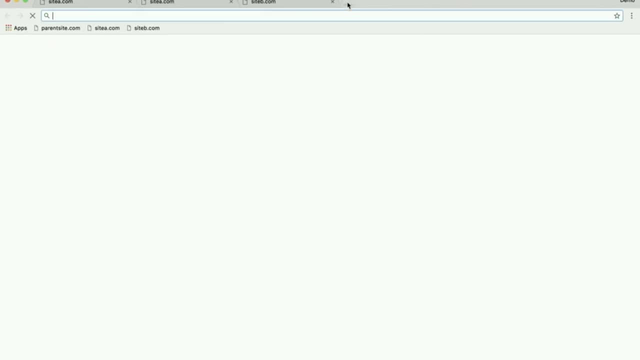 to actually access another window from JavaScript unless you open it and you have a reference to it or one of the other ways to get a reference to it. If there's a window over here with site A in it, the code in the first tab can't access that. 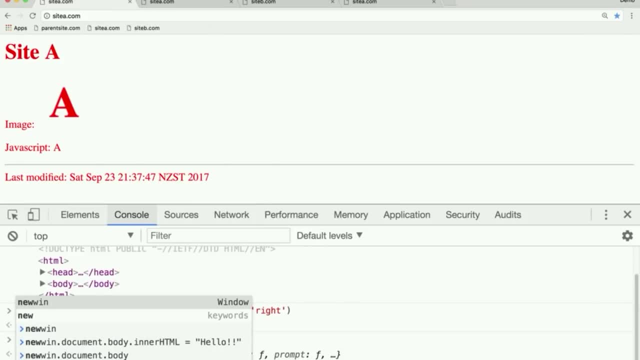 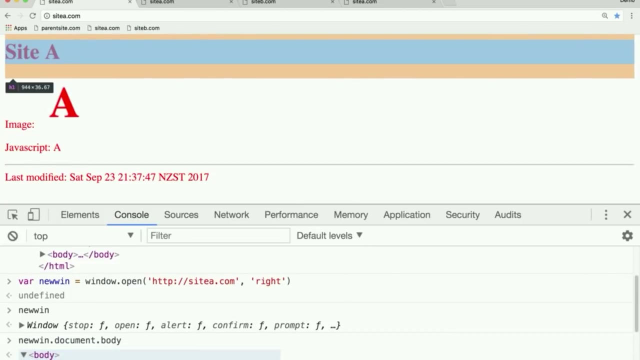 because it has no reference. Now we can look at the body of the second window. So we can look at the new one document body and we'll see that JavaScript in the first window can access the HTML in the second window and look at its internals. 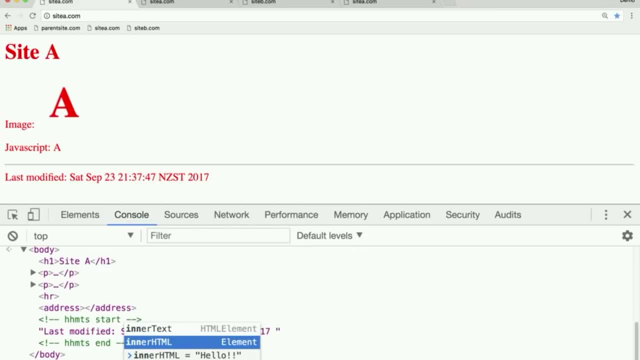 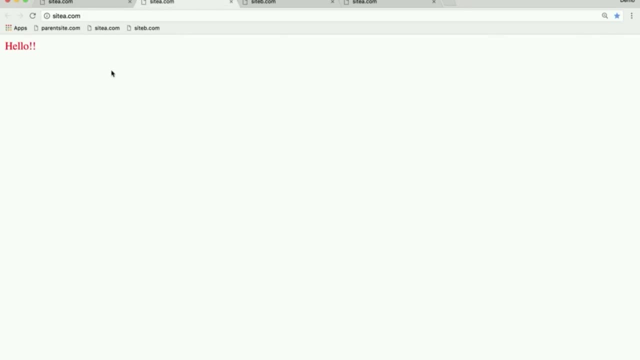 What if we decided we wanted to change that HTML? Well, we can just set it to something and because we've got a reference to that second window, our window is allowed to change the HTML. Now, would that work if it wasn't site A that we opened? 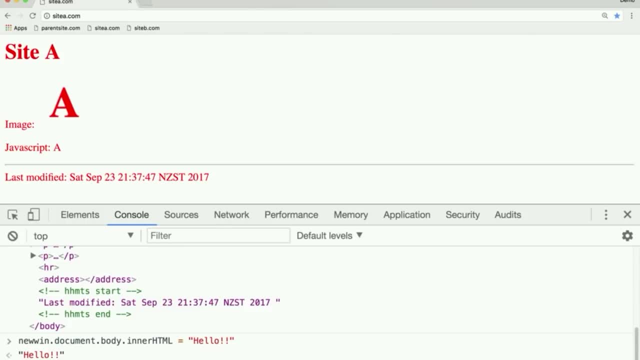 but it was site B that we opened. So let's go back to our window opening code. So we're in site A in this left hand frame and now we're opening a new window with site B. So we still have a reference to the new window. 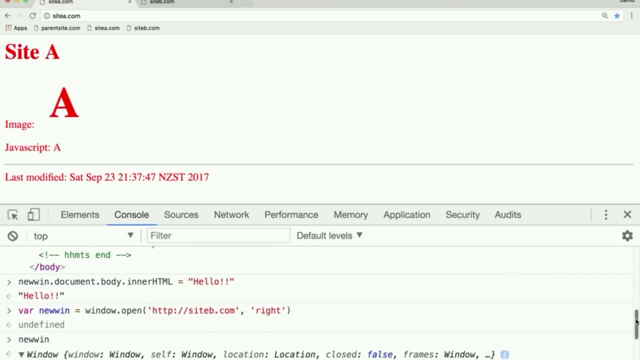 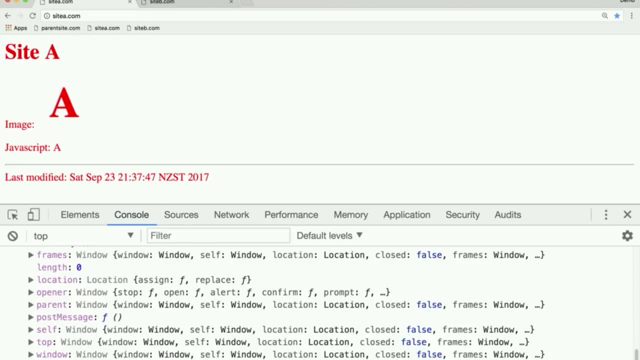 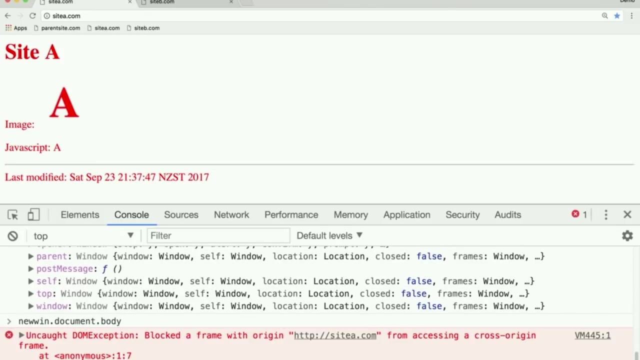 but when we look at it what we can see is a little bit more restricted. So before we were able to go newwinddocumentbody to look at the body of the page in the new window. now site A is not able to look at the body of the new window. 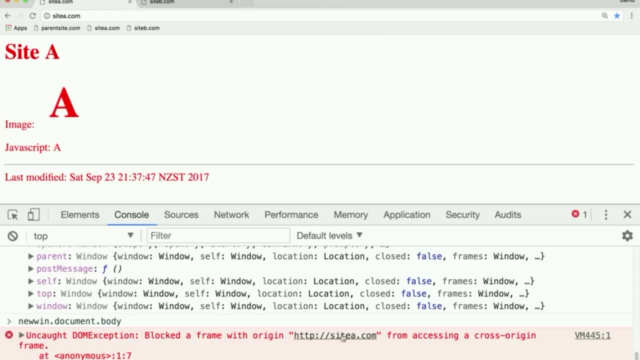 We've been blocked from accessing a cross origin frame and the browser's giving a nice message in the console saying that the current site is siteAcom and it's crying to access a cross origin frame and it's not allowed to. So this is the same origin policy at work. 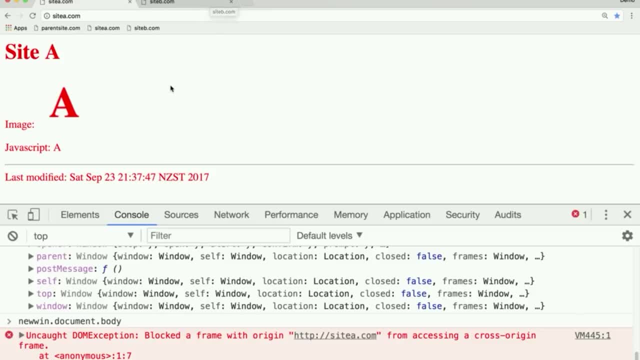 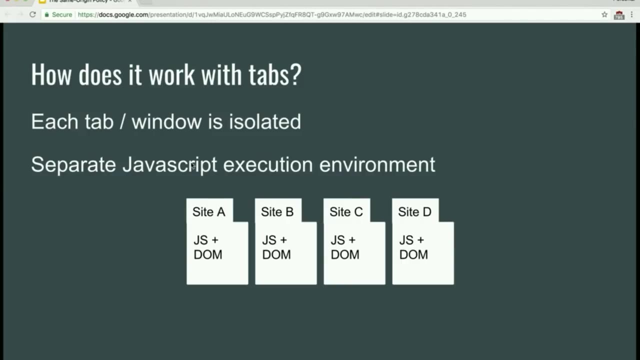 The same origin policy is enforcing that siteAcom is only able to access the content of other pages if they are in the same origin as site A. So how does it work with tabs? Well, each tab in window is isolated, so each tab has a separate. 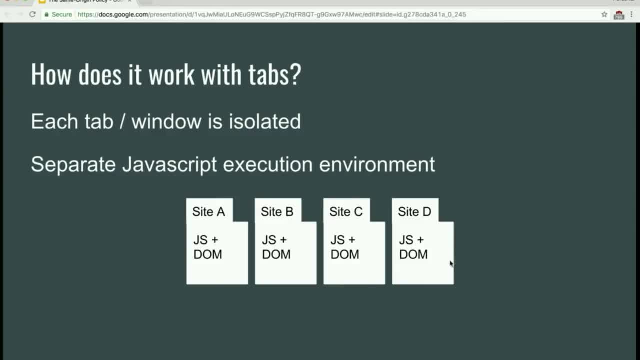 JavaScript environment. it has a separate DOM and they're all running independently. But if two tabs are in the same site, if they have the same origin, they may be able to access the data in each other. This is obviously not what you want if you've got a super secure site. 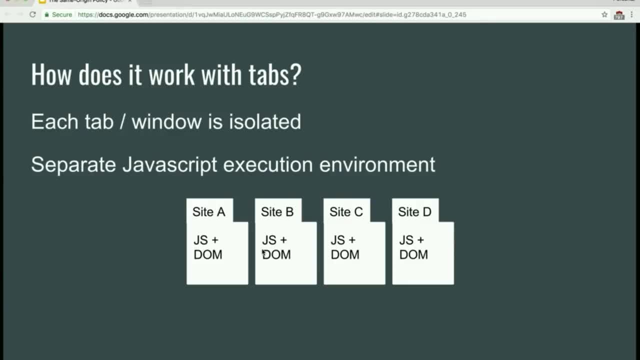 you don't want other tabs in the user's browser being able to access your data, And that's what the same origin policy stops. Just for the syntax of how it works: when you open a window, you get a reference and then the window that is opened. 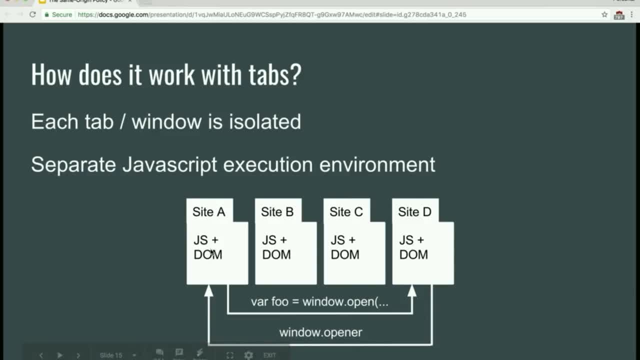 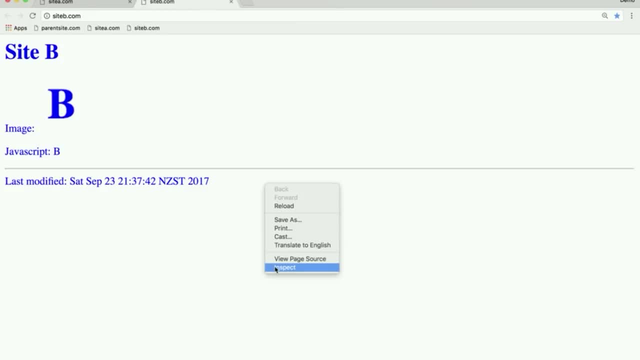 has a windowopener which has a reference back to the window that opened it. So if we go back to our example, siteB was the one that was opened, right? If we look at windowopener, there is a reference back to the original window that called 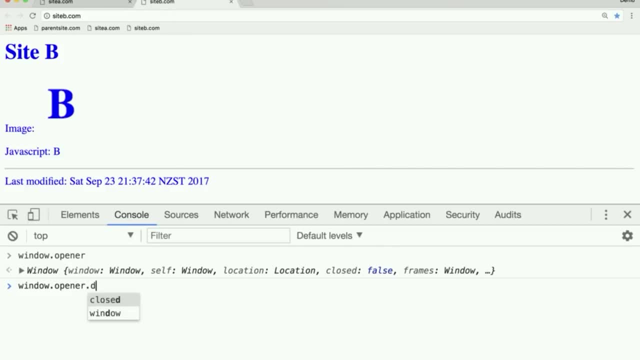 windowopen to open siteB. Now we can't look at the documentbody because we're siteB and that's siteA, so the origins are restricted. but we can do funny stuff, like change the location of the site that opened us, and so let's. 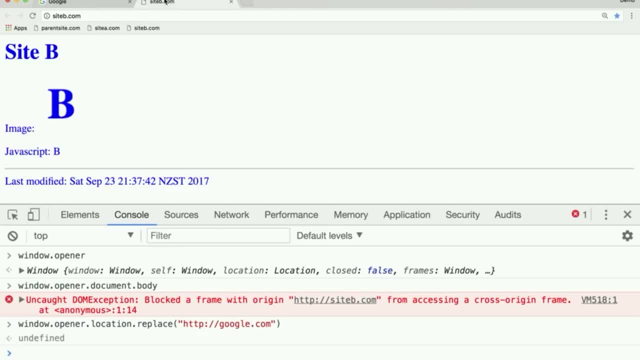 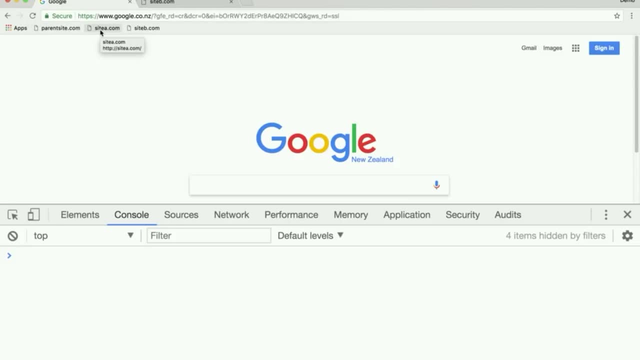 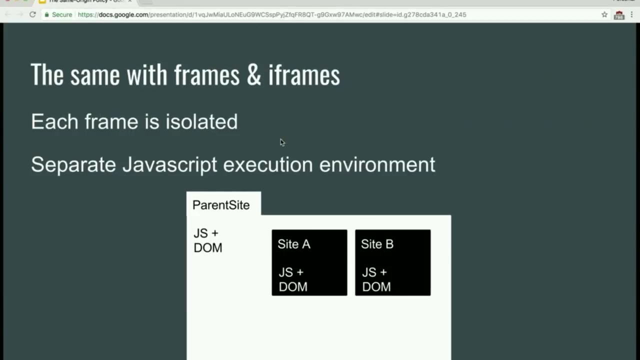 change it to Google and, crazily enough, siteB can actually change the original site that opened it to Google, and so we'll talk about the kinds of attacks that that allows later on and why that is. Frames and iframes are exactly the same, so each frame is isolated. 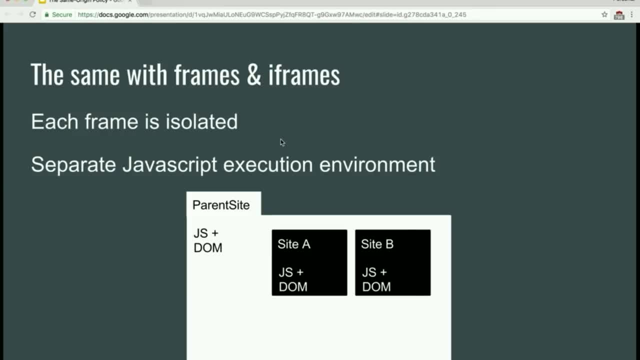 in the same way that each tab is. They have a separate JavaScript execution environment, a separate DOM, and the parent site that contains the frames only has access to the child sites if they are the same origin. The parent site can refer to child's frames by using windowframes. 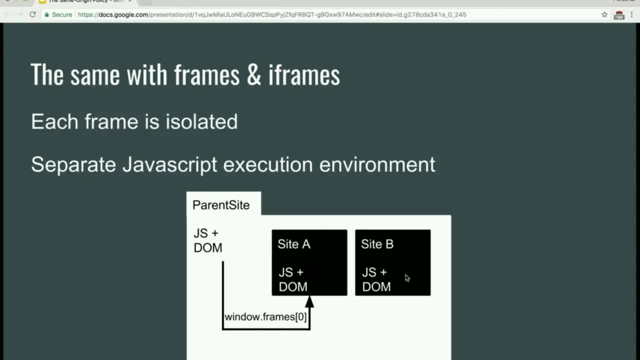 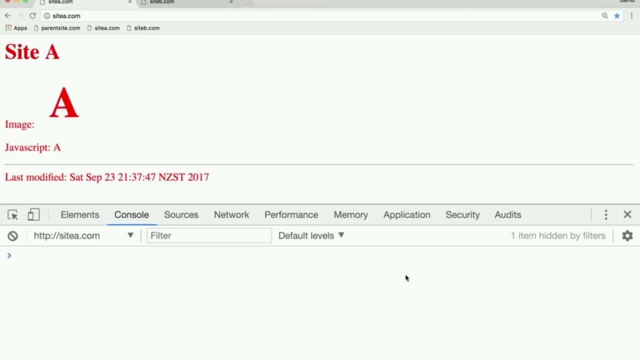 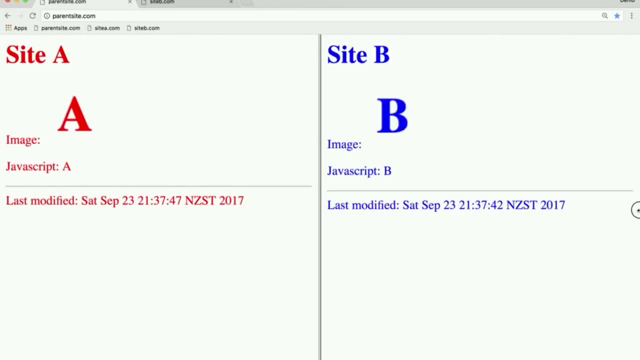 and then indexing into them or by using their name, and the child frame can refer back to its parent by using windowparent. So let's look at a demo with some frames. So here's parentsitecom, and now you probably haven't seen a site like this for a while. 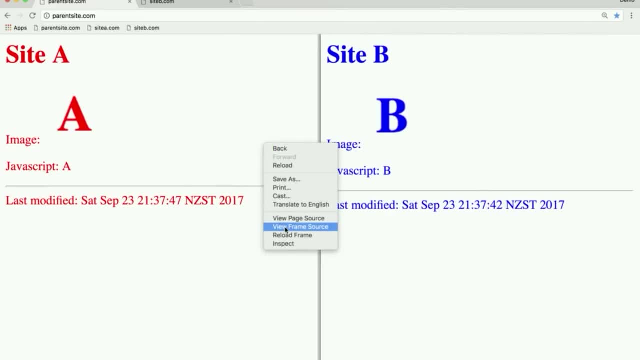 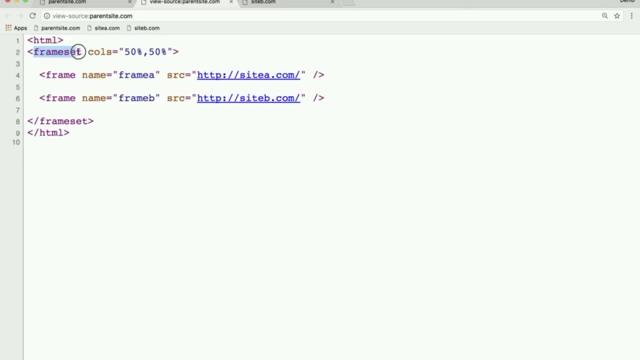 Whoa, Check it out, Crazy Oops. So we want to look at the source of the parent site. It uses an antiquated thing called a frameset and two individual frames inside it. Now, this is basically the same as iframes, which you probably have seen more of. 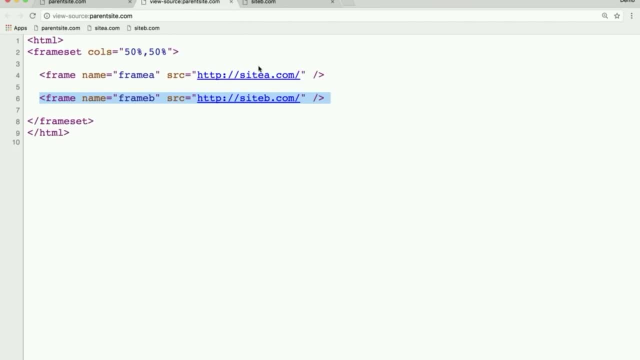 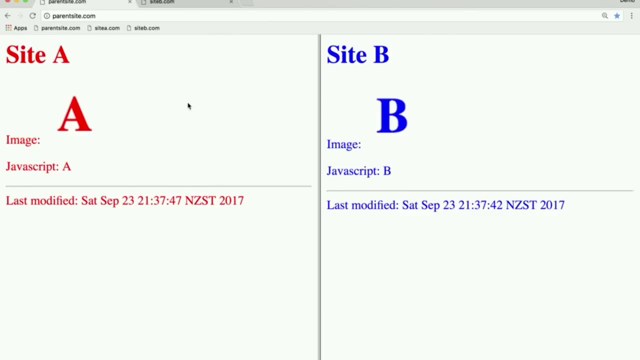 and what this means is parentsitecom has two smaller windows inside it, One with site A and the other with site B, So let's try and see what parentsite can actually do to the inner sites. So when we go to the console we can run. 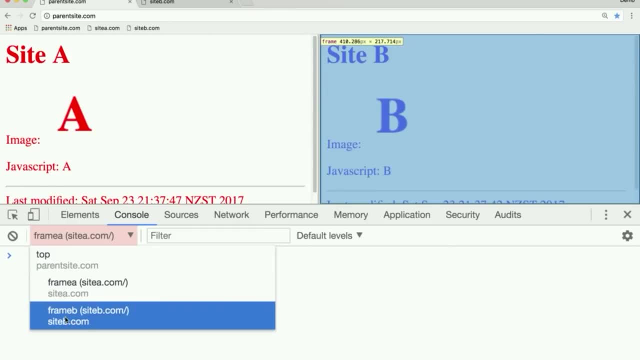 JavaScript in the context of the parentsite or one of the child frames inside that site. So let's do it in the parentsite. Now. the parentsite has two variables to refer to each frame because I gave them names. So frame A is the left. 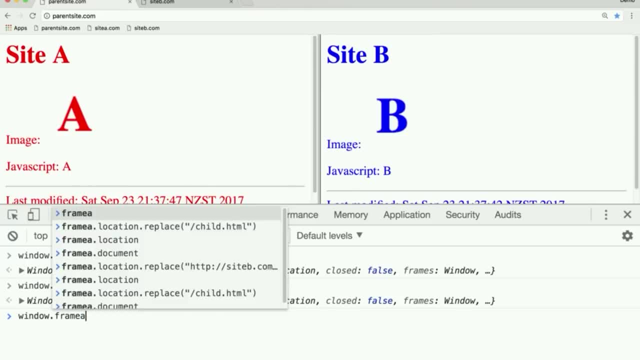 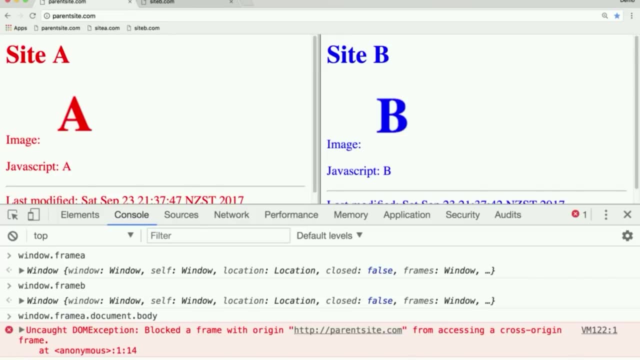 frame, and frame B is the right frame. So if we're looking at frame A, can we see documentbody? No, we can't, because parentsite is a different origin than siteAcom, which is in that left hand frame. It doesn't have access. 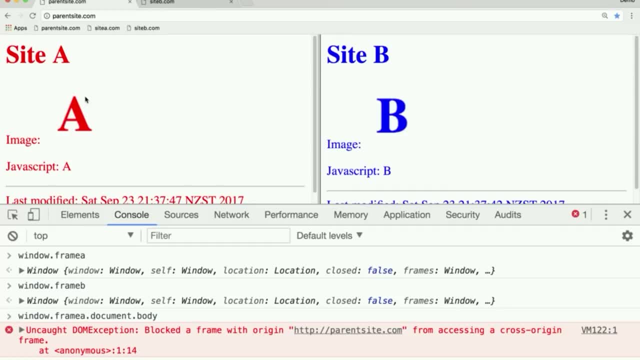 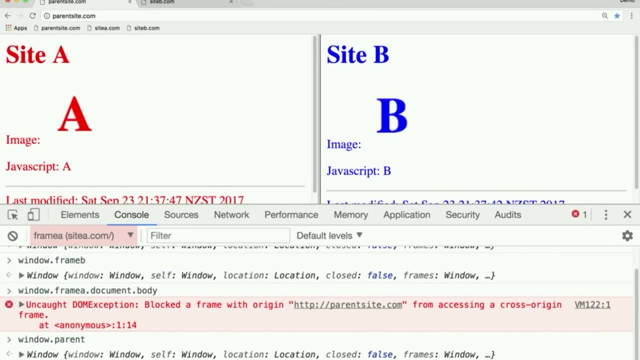 to look at the body. Now, what about if we're inside frame A and we're running JavaScript inside this left hand frame? Can we look at our parent? Well, we can get a reference to it, but can we look at the HTML inside the parent? No, we can't. 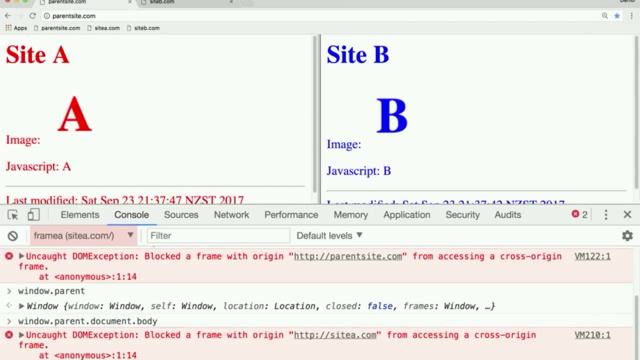 because siteA does not have access to accessparentsitecom. That's a different origin. So what? what siteA can do, I guess, as I showed before, is it can change the location of the parentsite. So imagine that this is a website. 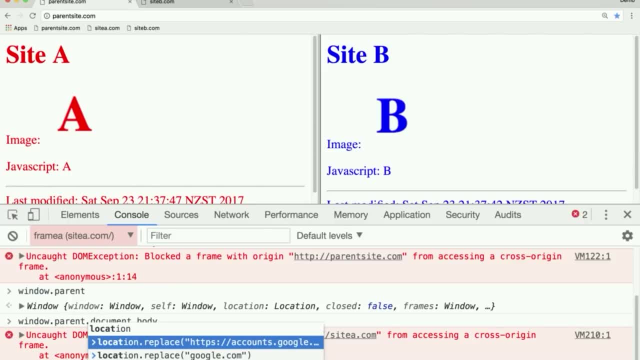 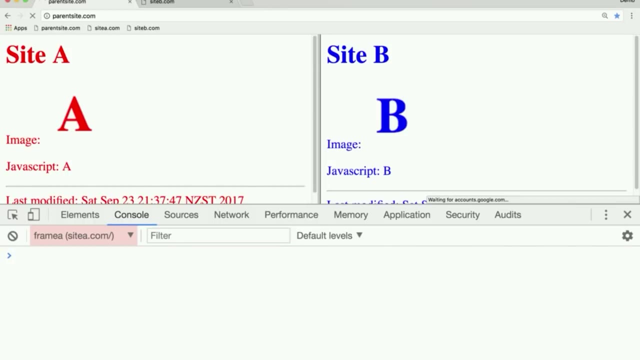 that embeds ads using iframes. It wants to protect parentsitecom wants to be protected from these ads, so it uses iframes to embed the ads. The iframes siteA can actually access windowparent and change its location, maybe to a Google phishing page, and then 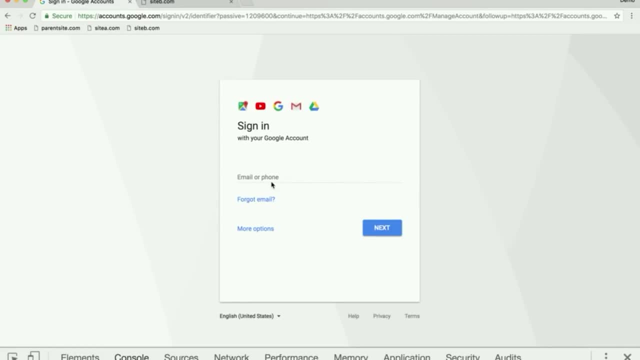 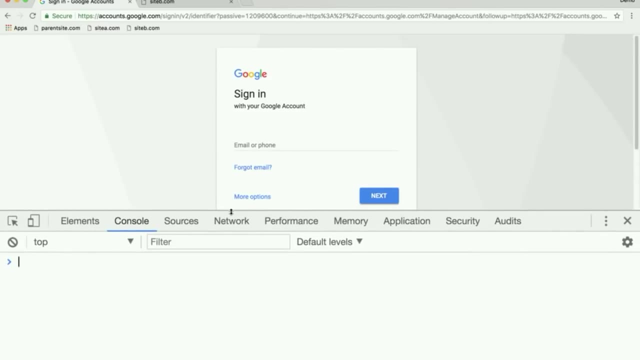 trick the user into logging back in and maybe capture the login or whatever. So it's interesting to note that iframes and frames can affect their parent. they just can't view the data and they're a sandboxed iframes you can use. You can look into further if you want to do this. 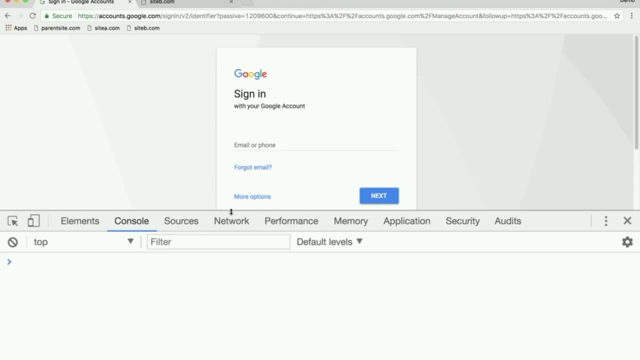 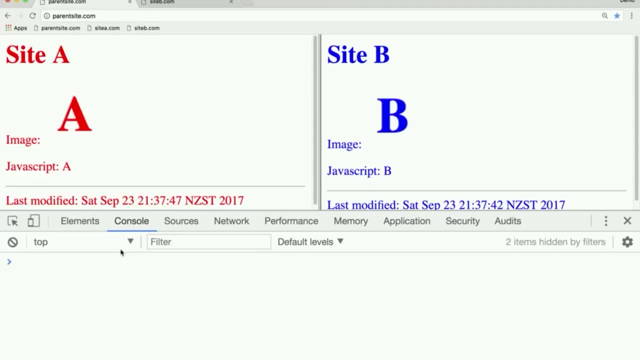 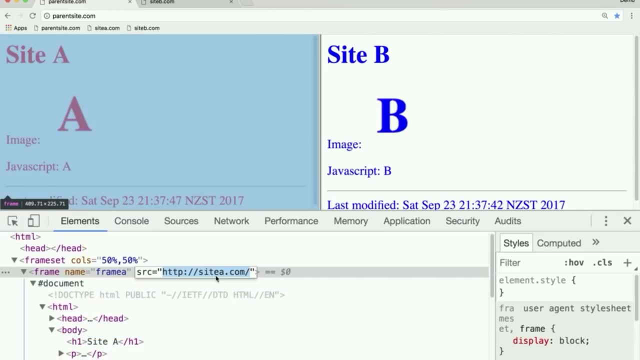 kind of advertisement thing so that you protect the location of documents. Let's go back to our parentsite. Let's change it so that instead of siteA in the iframe it has a subdirectory of parentsitecom. So we've got a page called. 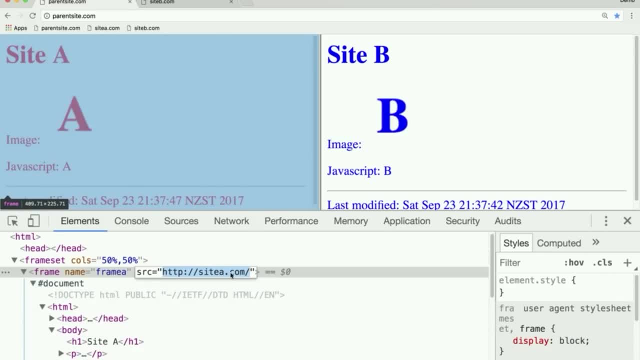 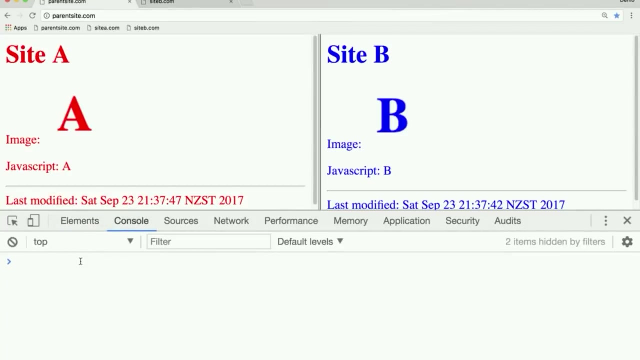 childhtml. Why didn't that work? What's happening? Let's do it in JavaScript. So windowframeA- windowframeA- documentlocation replace child. I don't know why it didn't work when I entered that. Never mind, So our parentsitecom. 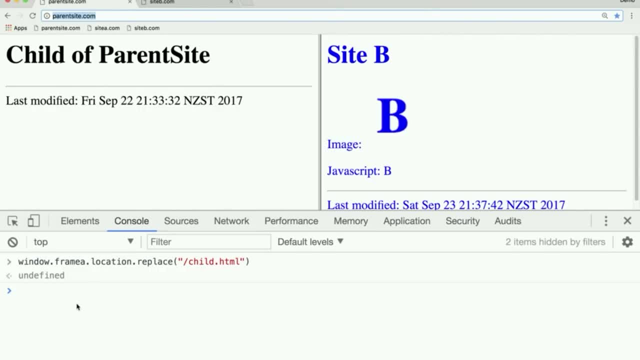 is the wrapper as well as the left hand frame. So from within parentsitecom- and it's JavaScript- I can look at my own HTML and I can look at the HTML of the child frame. So this is kind of what you'd expect. Frames are restricted. 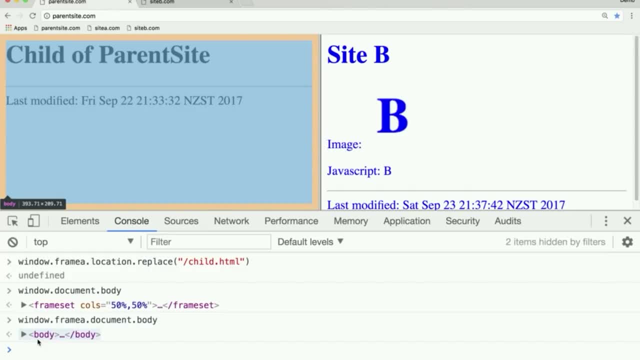 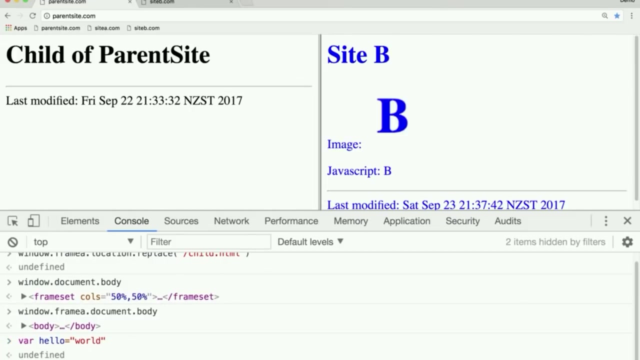 if they're in different origins. but if they're in the same origin, they're able to view each other's data. And one thing the pages can do is they can also make JavaScript variables. So say, I make a hello variable with the value world. 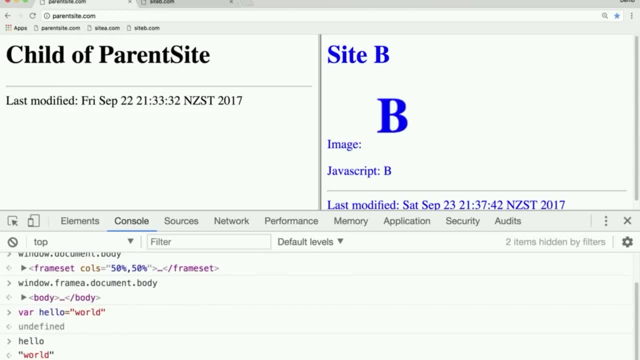 I've made that in the parent frame. So if I print out hello, I get world. If I go into the child frame, because it's the same origin, I don't have my own variable inside my frame, but I can go to my parent frame and look at its. 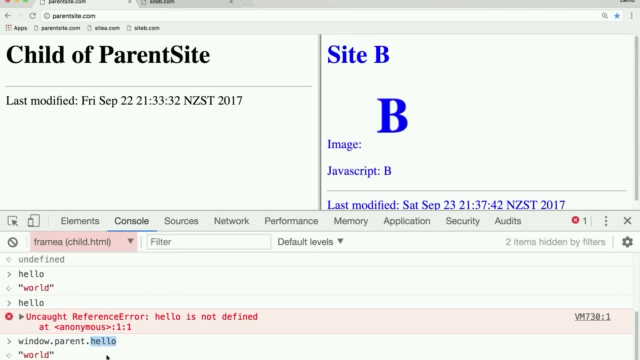 variables in the global scope by referring them to them in JavaScript, And so this is how parent and child frames can talk together. Now, this doesn't work for frames that are on a different origin, So sitebcom over here if it tries to go. 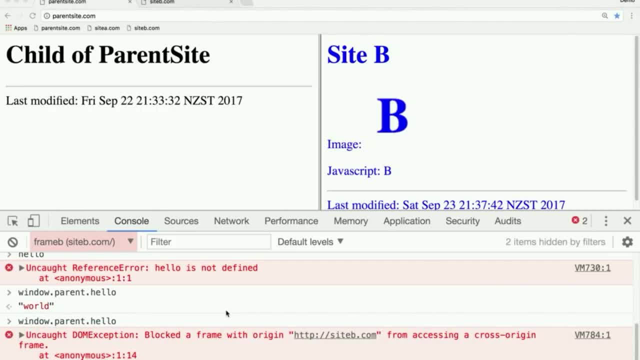 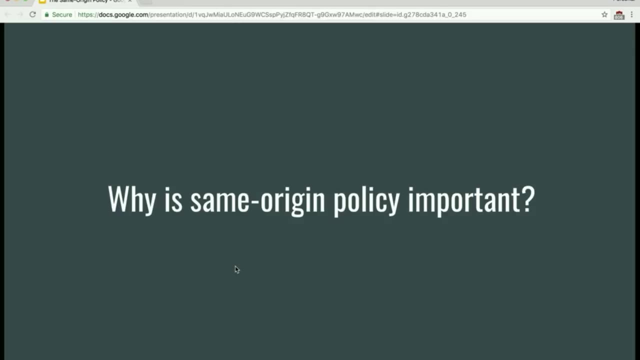 window- parent hello. it gets blocked because siteb is not able to access a cross origin frame in parentsitecom. So why is the same origin policy important? Why are we talking about it? Well, it underpins the security of your web browser. The same origin policy is the basic set. 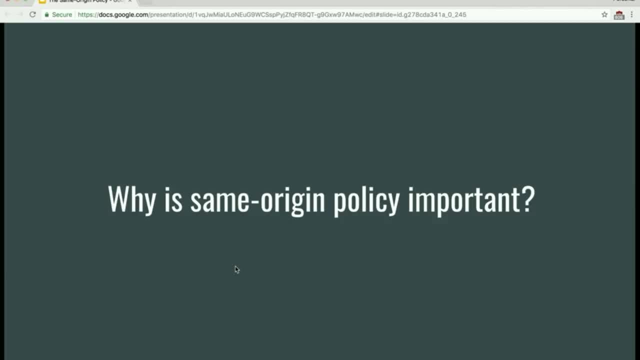 of rules that the browser follows to protect one web page from others in the same browser, And it's a mostly consistent set of rules that applies to most HTML features, especially the most more recently developed ones, where they've tried to be consistent but doesn't apply exactly. 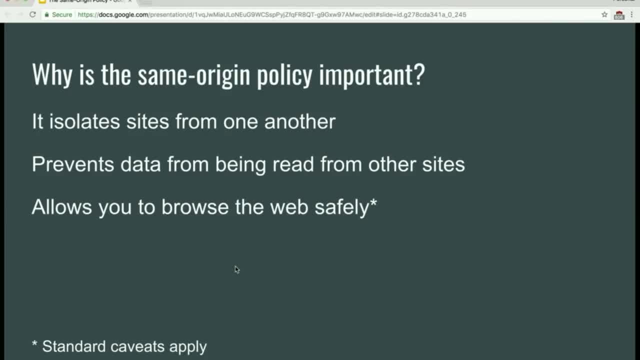 as you'd expect in some of the older features due to historical reasons. So the same origin policy isolates sites from one another and prevents one website running in your browser from being able to read the data of another website running in your browser, And it allows you to browse. 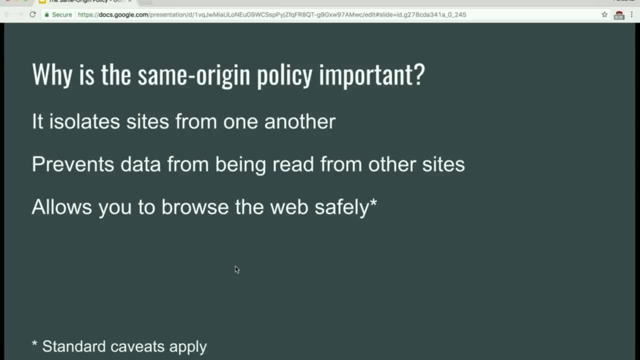 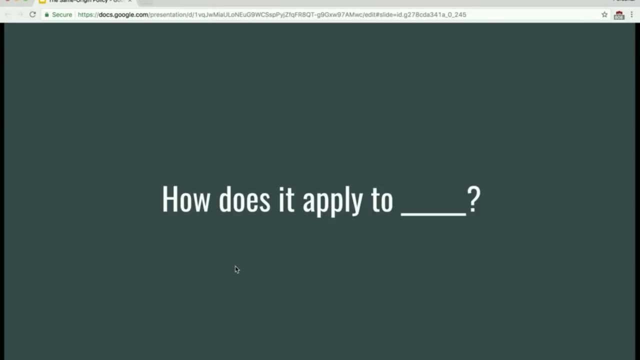 the web safely. So the caveat there is, of course it's dangerous browsing the web and lots of bad things can happen, but the same origin policy protects is what the browser uses. the rule set that it uses to protect one page from another and to make it safe. 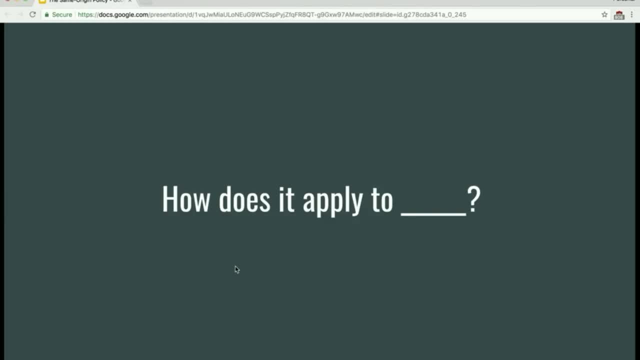 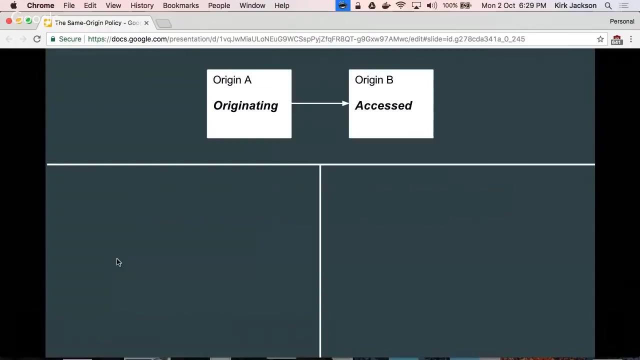 So the next section we're going to look at: how does the same origin policy apply to different technologies that you'll use on a day to day basis when you're developing for the web? So for these examples, there'll be two sites. there'll be an originating site. 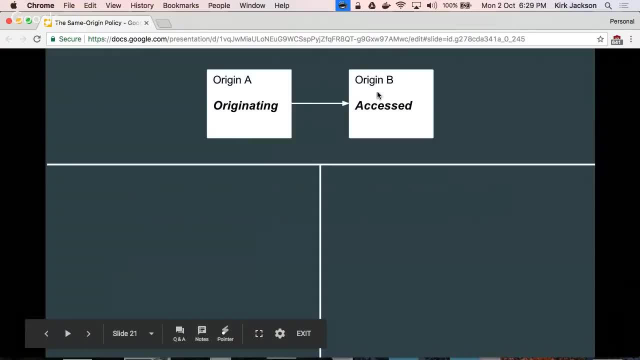 trying to access some resources of a site, a second site, and there's two kinds of scenarios. there's where the web browser- you've got one site in the browser trying to access Javascript variables or DOM and another site in the browser. and the second example is where you've got a site in your web browser. 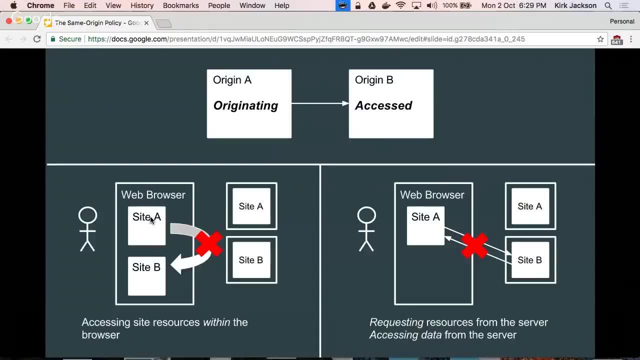 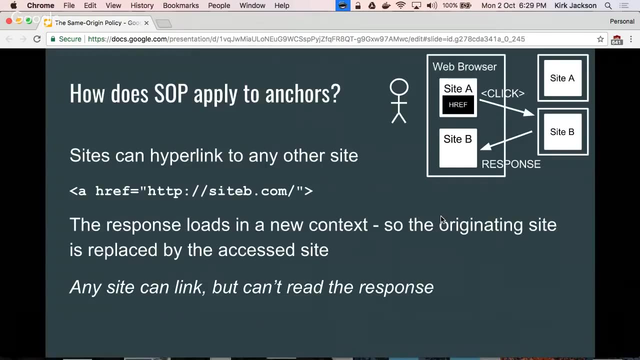 and it's trying to connect to a server and access data from that web server. so left hand side is within the browser from one frame to another, and the right hand side is one's talking to a different server than the one you're loaded from. so the first thing we're going to do 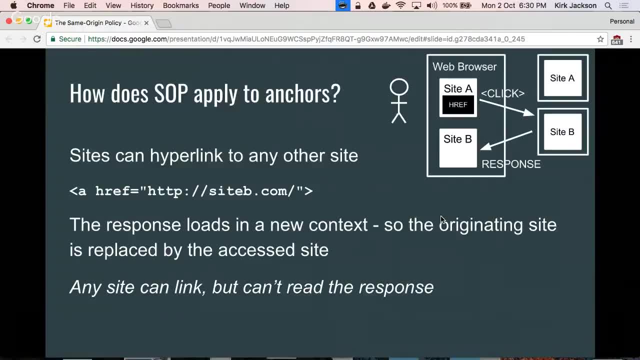 is anchors, hrefs, so this is pretty straight forward. any site can hyperlink to any other site. that's how the internet works. but when you link from one site to another, the response. so if site A has a link to site B, the response loads in the browser. 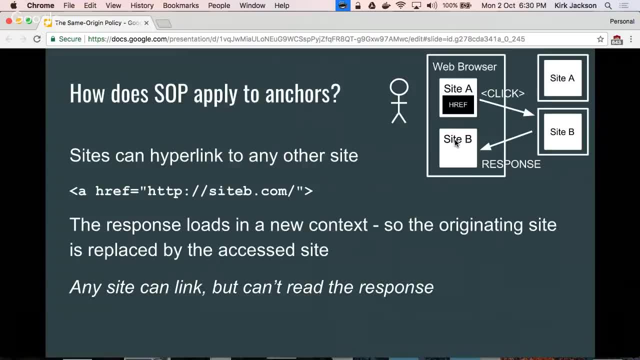 in a new context for site B. there's no leakage between site A and site B there. basically it's replacing the original site. so any site can link to another site but it can't read the response forms. so when you post, site A posts some data to site B, so just to the server. 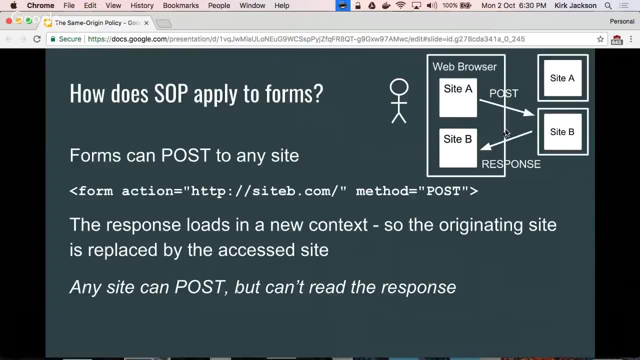 the response of a form is loaded in a separate context. so when the form is submitted the server will return some new HTML. that HTML loads in the browser in a new context. so this means that a site can post to any server that it wants, but it can't read the response. 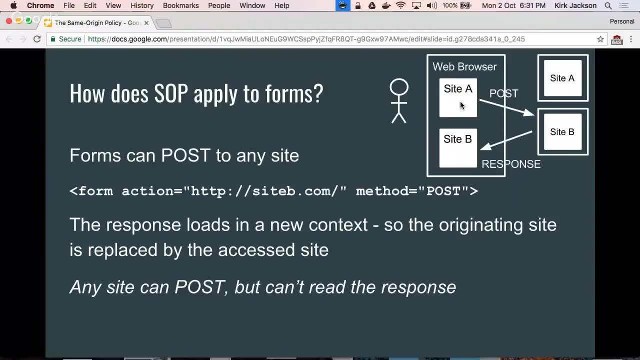 so, for example, if this site A was evil site and it was trying to post a funds transfer form to your online banking, it would be able to send the request from your browser to site B, but it wouldn't be able to read the response to see if that was successful or not. 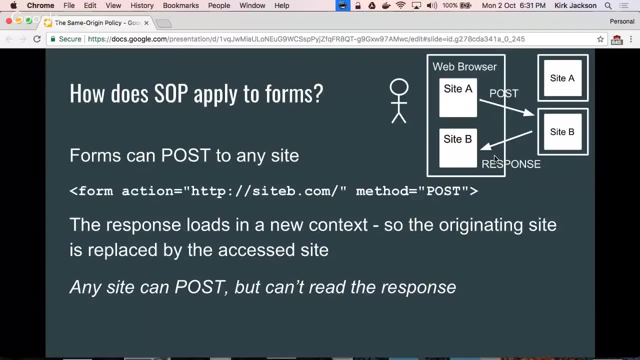 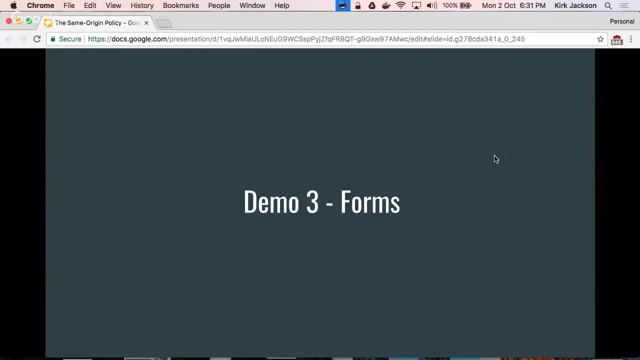 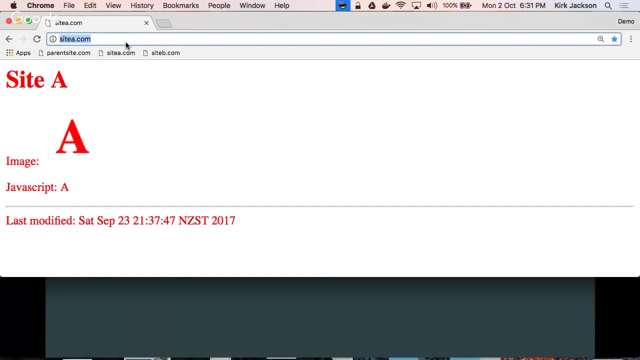 you get no indication of whether that worked properly for regular form posts. ok, so this demo is the thing. you probably have seen forms before. so site A slash form, oops, posthtml. so just to show you what this is, it's a pretty simple form that's posting to site B. 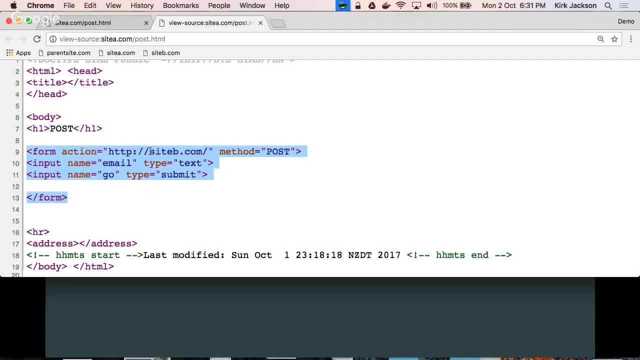 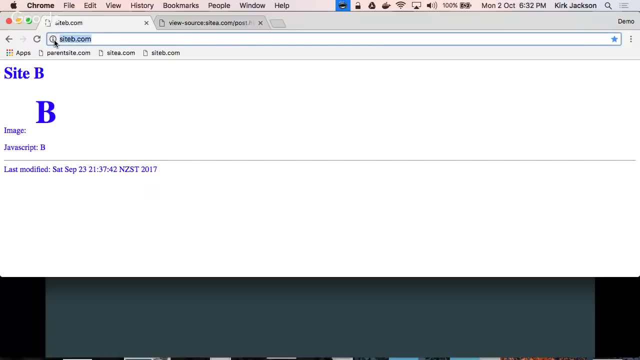 when I enter an email and click go, it's going to send the information to site B and you notice that site A got replaced with site B in the browser. so it's a completely separate context. there's no way that site B can attack site A. there's no way for site A to read the data. 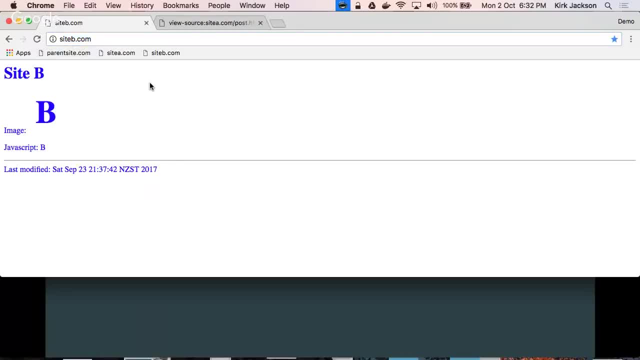 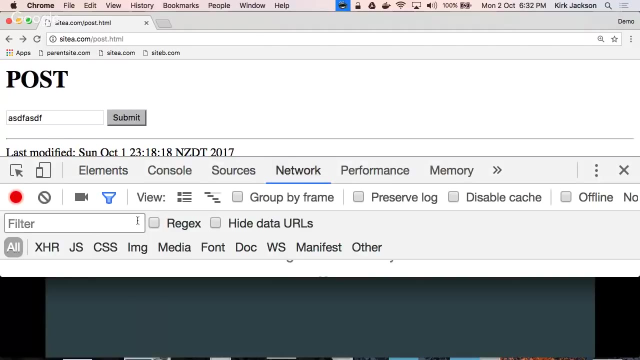 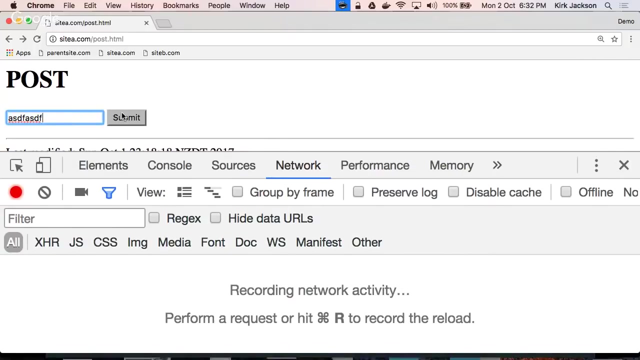 it doesn't even exist in the browser anymore. there's only site B. site B has received the post data, so we could have a look in the dev tools and watch that happening. I'm going to need to increase this a little bit, so when you're on site A and you press submit. 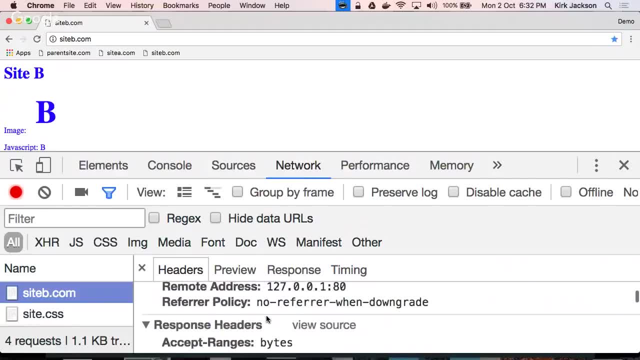 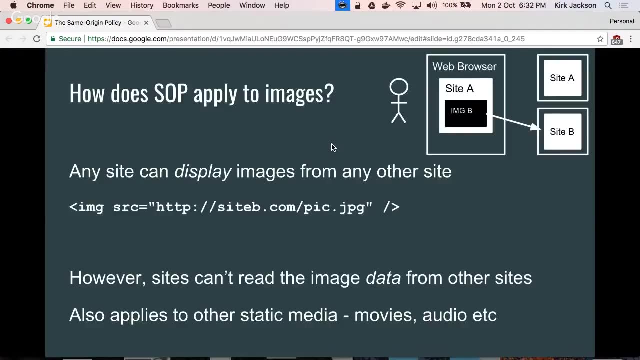 there's been a post to site B and inside the post somewhere will be the email address that I entered: astf, astf. I might need to zoom that a little bit smaller, otherwise it's going to be hard to see. cool, so forms work how you expect. 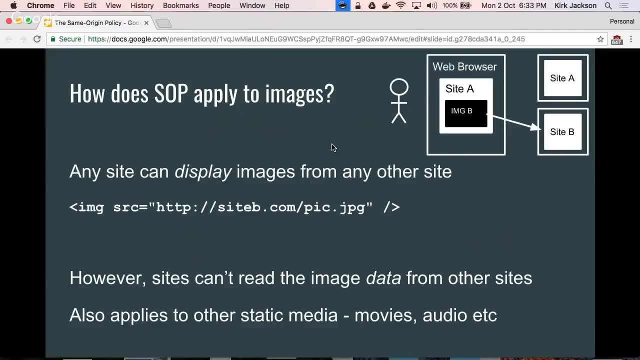 and how you probably use them. so images: another quirk is that any page can embed images from any other page from any other web server on the internet, so we do this all the time. we'll put our images on a CDN or whatever, but site A can't read the image data. 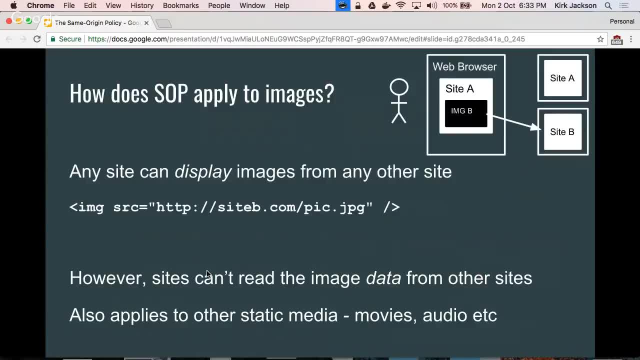 that's embedded within it, and this was historically an issue, because if you're able to access the data inside the image that you're displaying, you might be able to get people's secret images off Facebook or whatever. site A might be able to load something from site B and then look at what got. 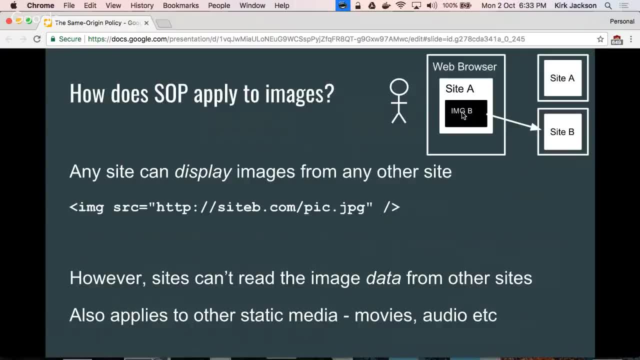 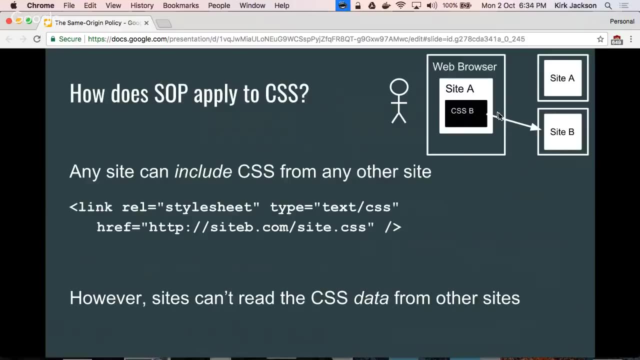 got returned. this is the same for all static content. so movies, audio, everything. you can source them from any URL. cool same with CSS. so you can include CSS from any other site. so site A can load the CSS from site B but it can't look at. 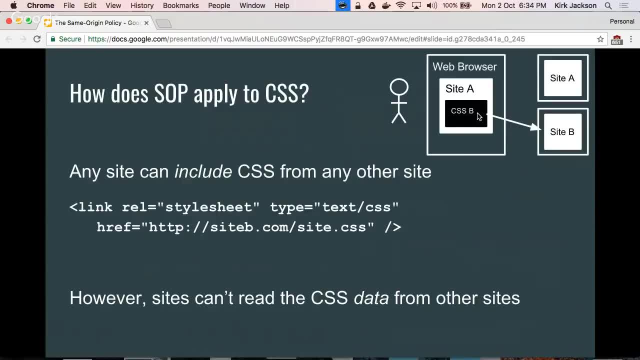 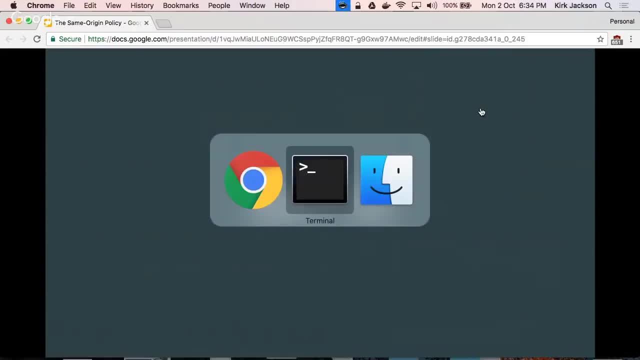 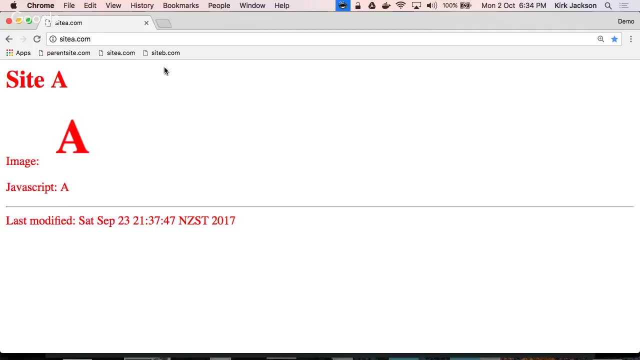 the data that was returned by site B, so the web browser might change its colours and stuff depending on that CSS, but you can't actually look at the CSS itself. I'll show you how that works if I press the right tab key so you'll notice that site A. 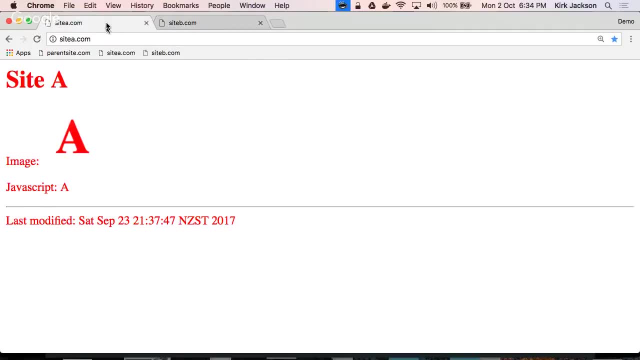 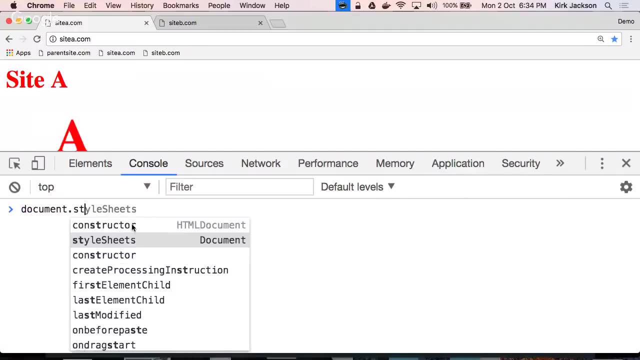 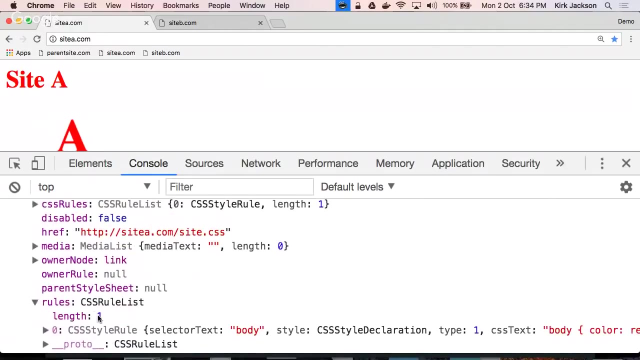 is red and site B is blue- good use of colours. so if JavaScript is running in site A it can go documentstylesheets and look at its own stylesheet. so site A has the stylesheet siteAcom, slash, sitecd and you can look at the rules in here. 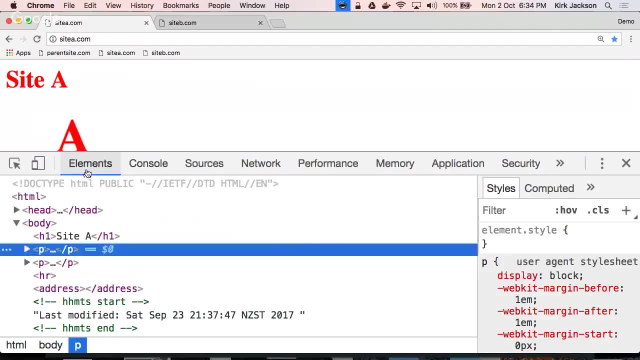 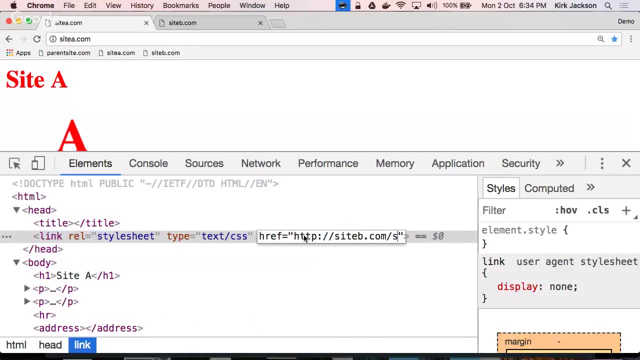 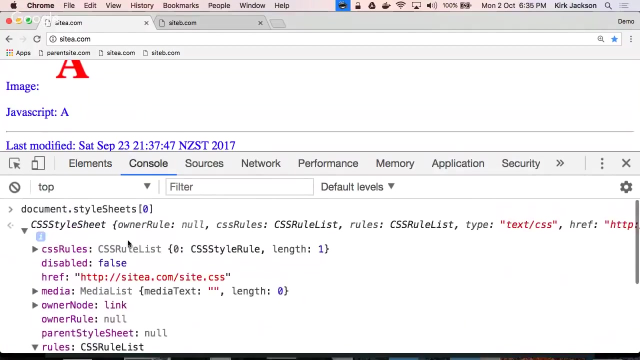 and somewhere in here that its colour is red. but if I change this and change the URL, sitecss thanks. so the text has changed to blue, the image hasn't changed. so now when I try to access the stylesheet from JavaScript, we'll see what happens. we can see the URL of it. 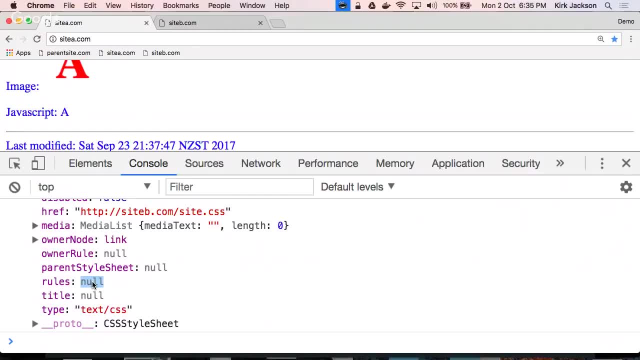 but when we look at the rules, we don't get access to the rules, and so that's just in case site B's stylesheet had some sensitive information in it. basically, the same origin policy applies to that as well. site A can only see the CSS of sites from the same origin. 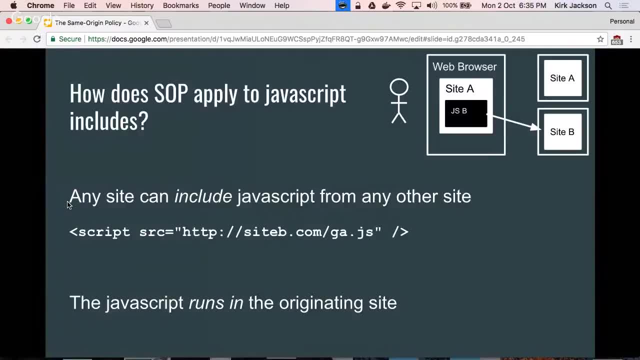 okay, so we're going through some of the normal stuff you will have seen. the simple thing you would have seen is including JavaScript, and you'll know that one website can include JavaScript from any other site, so site A can include JavaScript from site B. you were saying that. 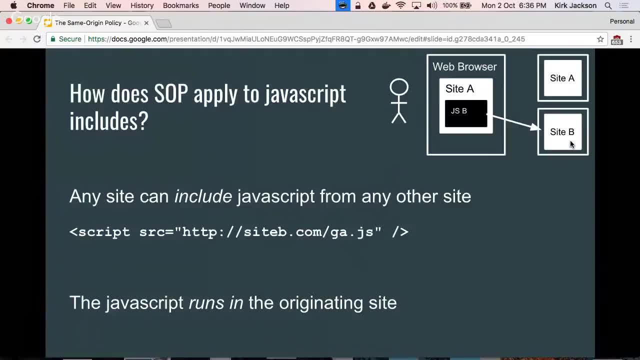 this is controlled by the browser, not from the server side, so if you're using not browser, then you can bypass it. yes, so the question was: are these rules controlled by the browser? which is yes, they are, and the answer is yes. so if you write your own NET code, 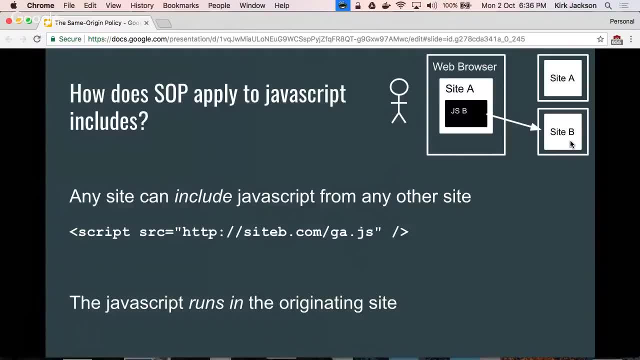 and request a CSS file, you can look at the contents of it. but if JavaScript in a browser tries to do that, it can only look at the contents if it's on the same URL. so JavaScript includes. you can include JavaScript from any other site. the only thing here is: 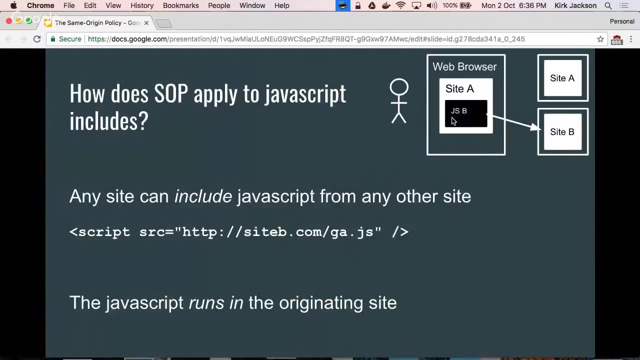 that the JavaScript runs inside site A. so this is kind of alluding to, I guess, cross site scripting, which you might have heard of. I know there's some videos of previous talks about it. site B's JavaScript is going to run in site A and do whatever. 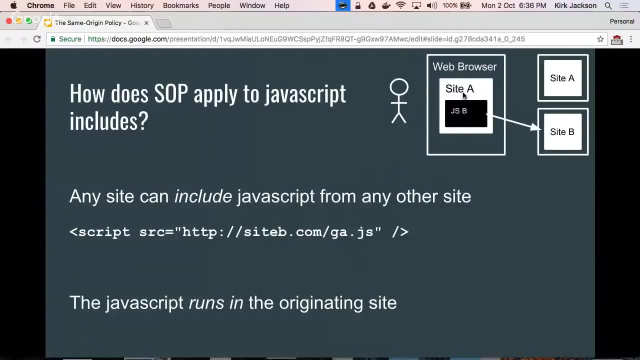 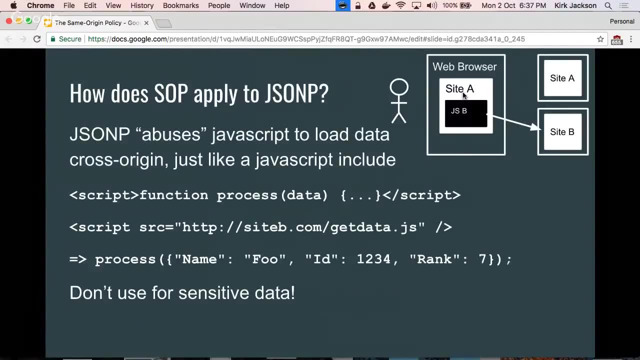 site A whatever site B wanted it to do, which means that if you include site B's JavaScript, it could potentially attack site A. there's a particular abuse of JavaScript called JSONP, where you include an external JavaScript like siteBcom to get data and when that JavaScript runs. 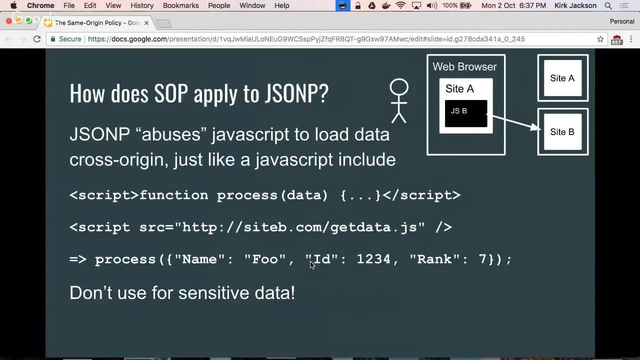 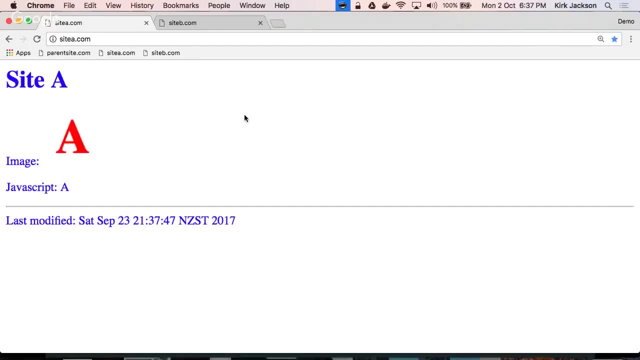 inside your site. it calls a function in your site to pass some data to it. so I'll just show you how these two things work with JavaScript. so let's get site A back to normal. so you'll remember from looking at this site: A includes some JavaScript. 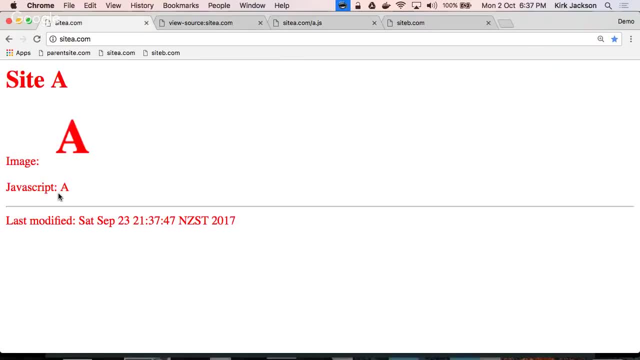 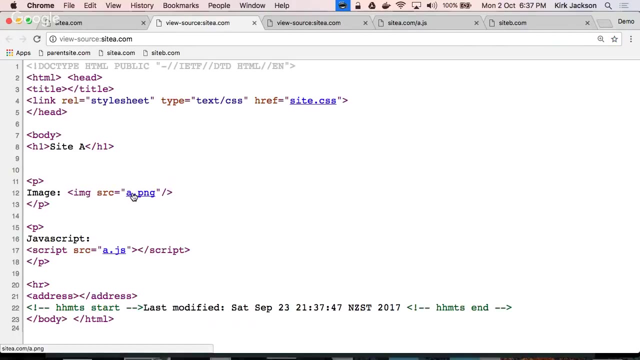 that writes A. I'm pretty good at writing JavaScript. that's the output there, and site B includes some JavaScript that writes B. so if I was to load site A, I could change that script tag to include site B's JavaScript and B would be written in my page. 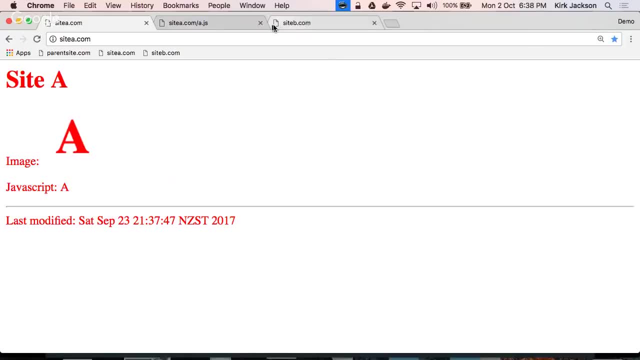 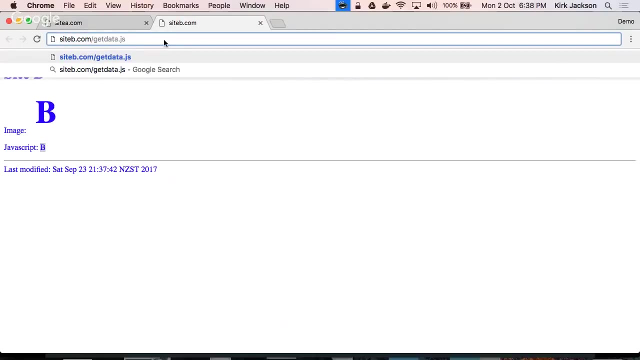 it only runs at load time so I can't just edit it to show you. so, JSONP: I'll just show you how that works because it's one way of sending data from one site to the other. so site B has an endpoint that returns some data from a database. 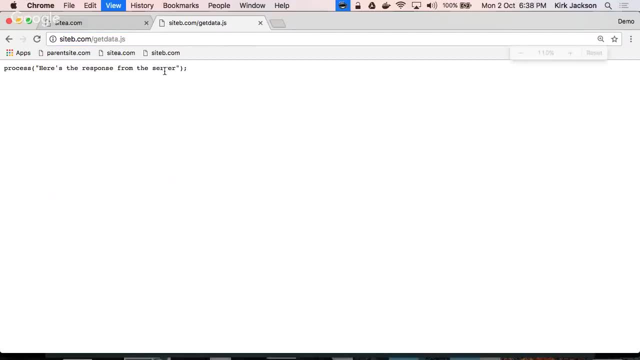 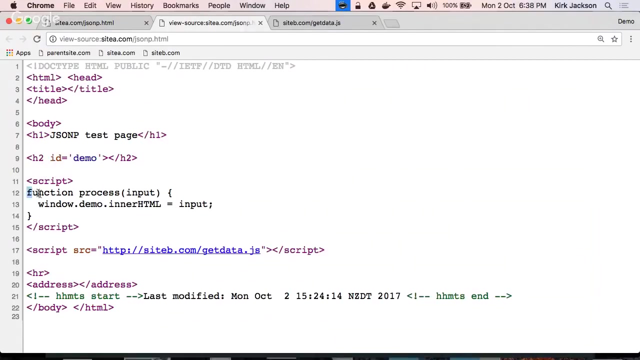 that's the data. here's the response from the server. so site A wants to take the database result from site B and embed it in the current page. so here's a page where I do that. so what's just happened? site A made a function called process. 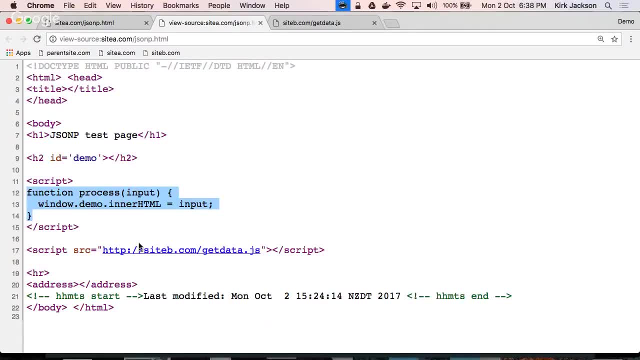 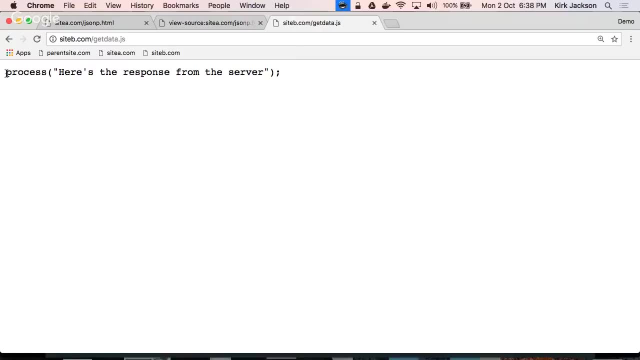 that waits for some input and when that input comes, it writes it to the page and then it includes site B's JavaScript. and if you look over here, site B's JavaScript calls that process function that we created and passes some data to it. so the end result is: 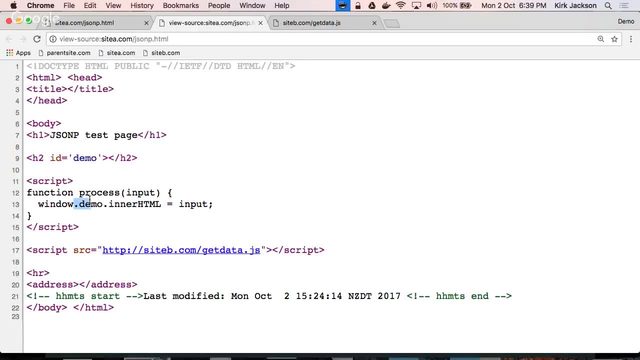 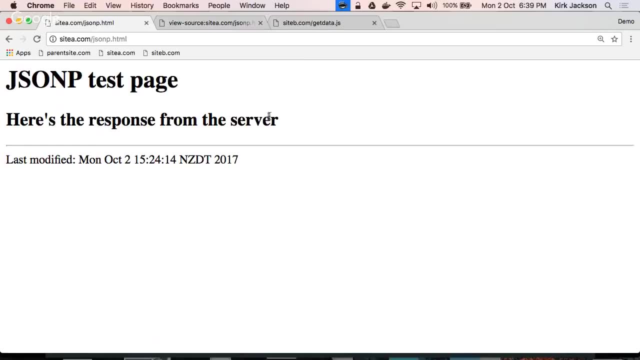 there was an H2 tag that was empty and site B is sending some data to this function, which is getting written to that tag, and that's what you see there. does that make sense how JSONP works? ok, so JSONP is kind of an abuse of JavaScript because 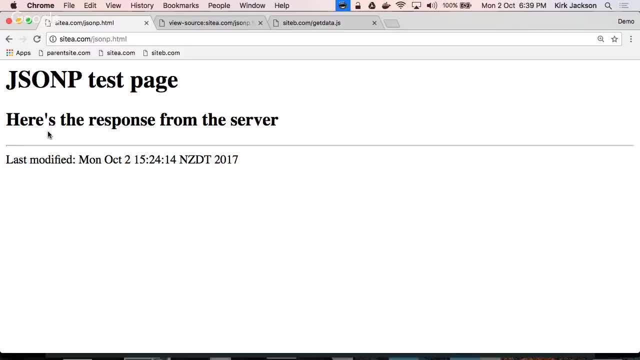 the same origin policy wants to stop you getting data from other servers. but you're allowed to get executables. you're allowed to get JavaScript code and run it. you're just not allowed to query a server for data and look at it. so JSONP turns the JavaScript. 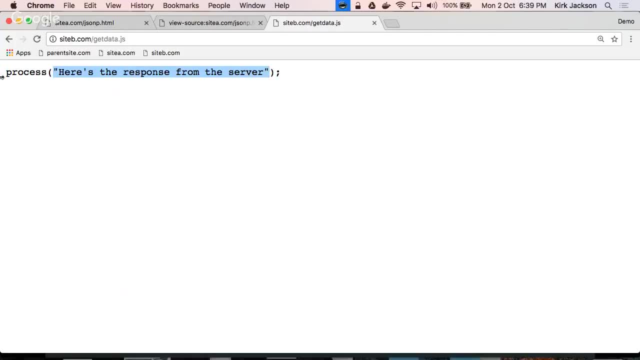 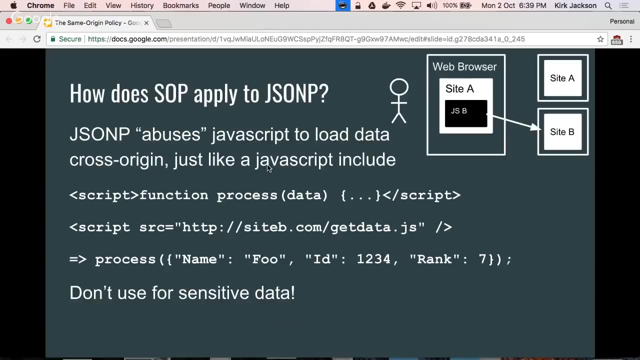 data- which I guess is the bit between the string- into an executable. so your page is running that. ok, I've put here: don't use for sensitive data. I don't think you really need to use JSONP anymore these days, but I've included it for completeness. 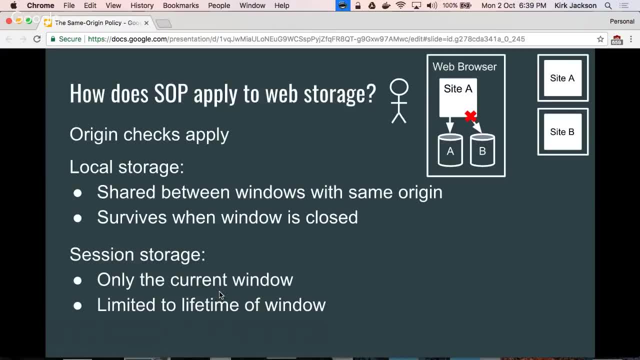 you can dig into why it's a bad idea. so next web technology is web storage. so you might not have seen web storage. it's the ability for JavaScript running inside your site to store data in the browser, and what it lets you do is you have this little database in your browser. 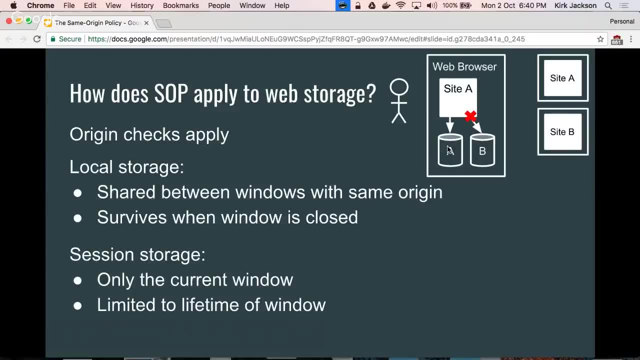 where you can store data for your origin and no other origin can access the data. and there's two types of web storage. there's local storage and session storage. local storage stays forever and is accessible across all the tabs in your browser, and session storage is only the current tab. 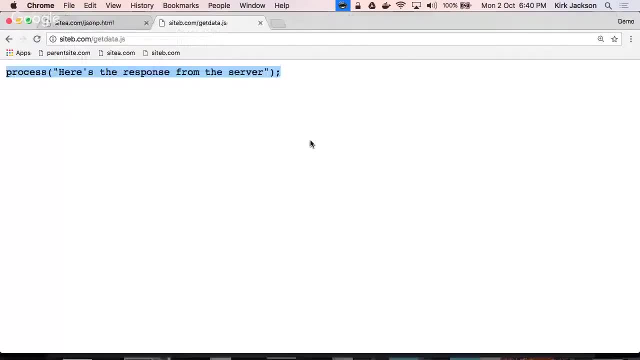 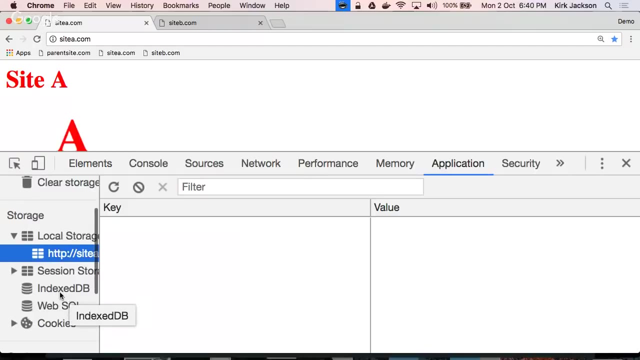 or the current window. so I'll show you how that works so that I remember what the URL was. I think I don't need a URL for this, cool. so if you want to see what web storage looks like, you can go into application and there's two areas. 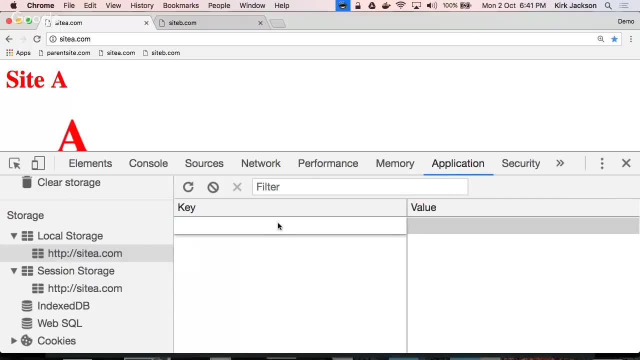 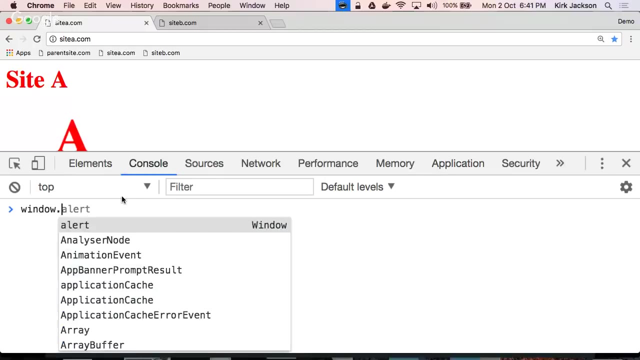 for local storage and session storage and you can stick things in there. so local storage, session storage, so, or you can do it programmatically, which I guess is what you're more likely to do. local storage, call it temp, call it test to get the data out and you can put new data in. 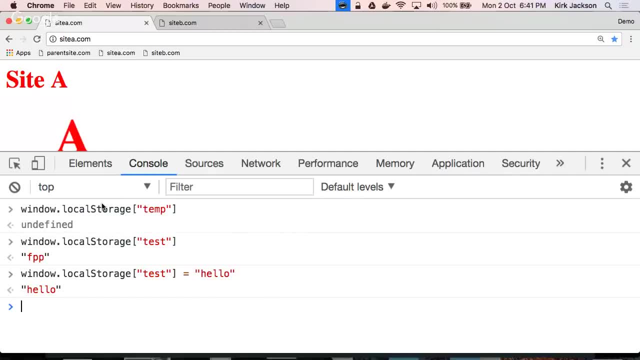 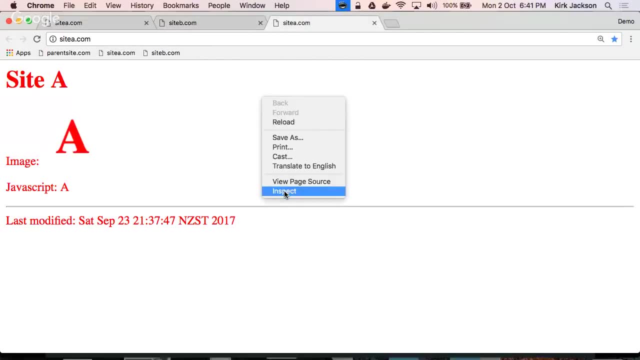 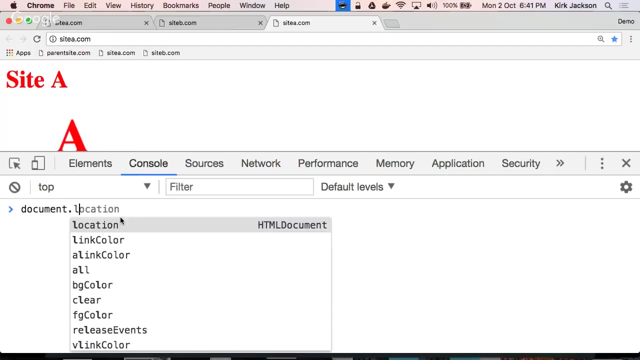 so, as I was saying, local storage can be accessed by multiple tabs. so if site A is open in two tabs, then oops, window dot, local storage. sorry, excuse me while I javascript. you know the second tab can see the storage that was set in the first tab, so we set it in one. 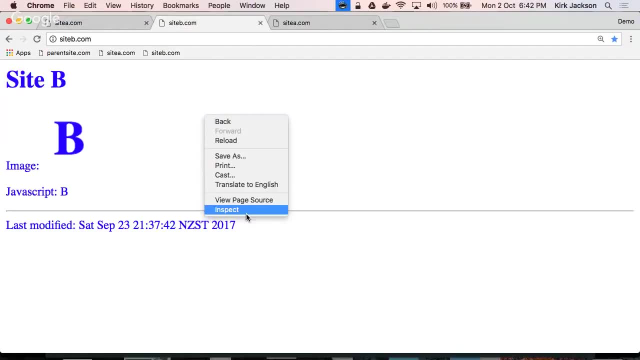 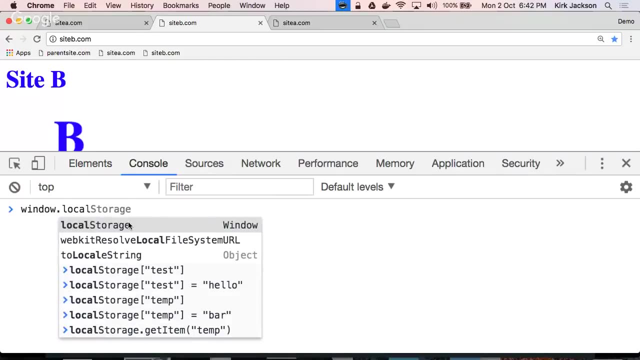 we can see it in another. but if I'm on a different site- site B- I don't have any access to site A's local storage. so if I go window dot local storage test I don't get any data. so basically, web storage follows the same rules and 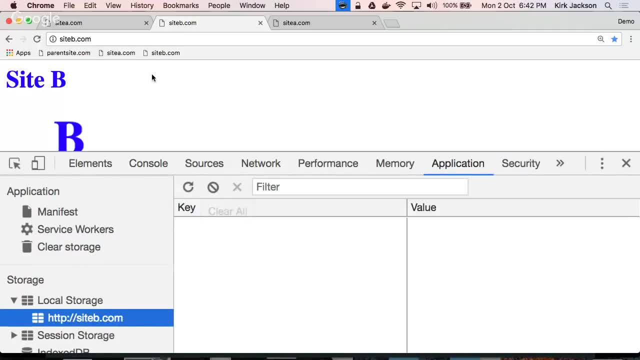 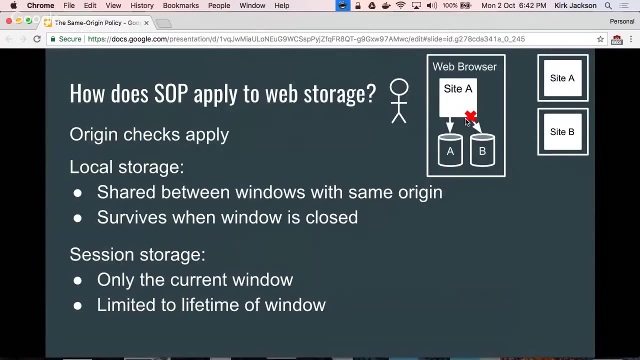 you can see the origins, I guess, and the data that's stored by drilling into the application tab and looking in there. cool, and that's denoted by an x in the picture. you can't access other people's storage, so cookies, cookies are the ugly stepchild. 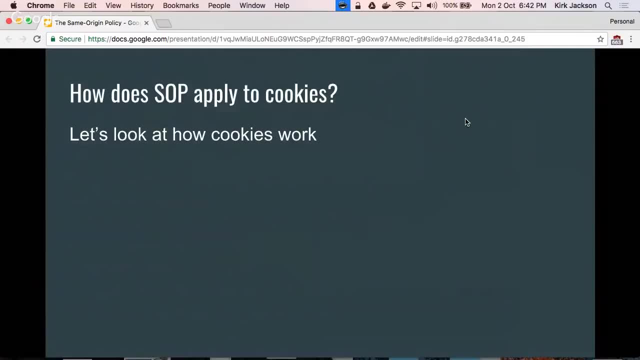 of the web security world, and I think it's because they were designed like first, before Netscape and whoever had their idea around how data from one site could be accessed by another site, and it's different to all the rest. so let's look at how cookies work. 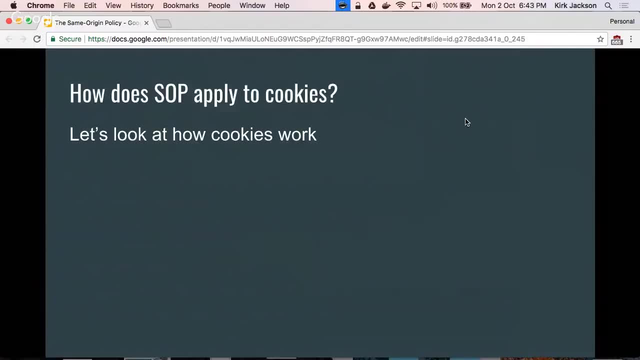 it's probably going to be a refresher and if you want to look at more about cookies and how they work, I recommend checking out Veil's CSRF book from a few months ago. so here's an animation. so a gender neutral stick figure goes to site A dot com. 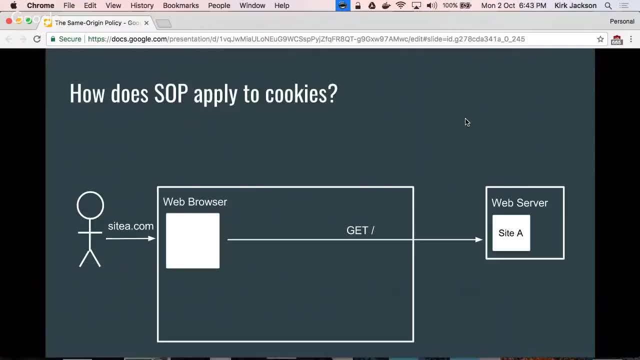 in their browser and the browser requests site A dot com from the web server. site A dot com has returned a cookie, so the browser stores that cookie in a cookie jar specific to site A dot com and returns the rest of the HTML, without the cookie, to the web browser and the web. 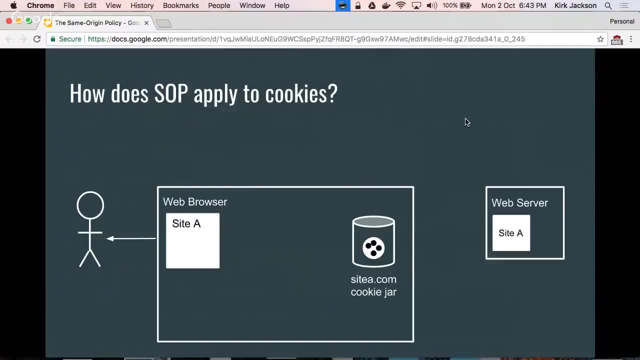 browser makes a context for site A and displays it to the user. if the user gets another page on the same site, the request goes from their browser. it goes through the cookie storage and grabs the cookie on the way, requests the page from the server and the server returns the HTML. 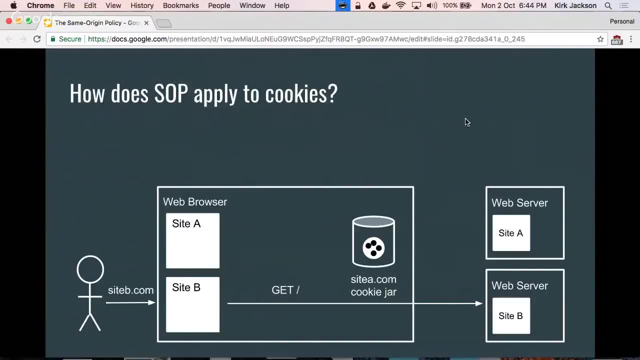 looks like I skipped a step in my animation. so what happens when you open a new tab and you request site B? well, it doesn't have access to site A's cookie jar, so your request to site B just goes straight to the web server and you get some response back. 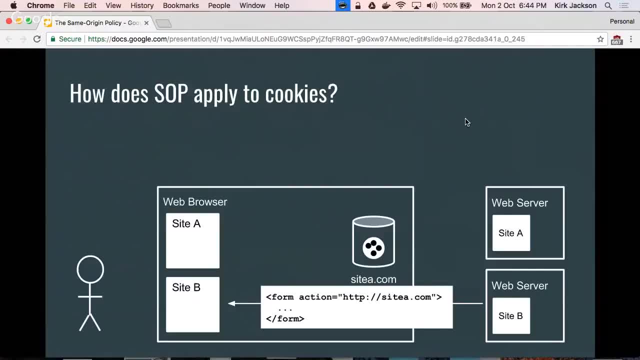 but what if the response is a form which tells the site B in your browser: hey, when you post this data, send it to site A. and this is the cross site request for drew attack. that I'm showing so you can dig into that by watching previous talks what happens. 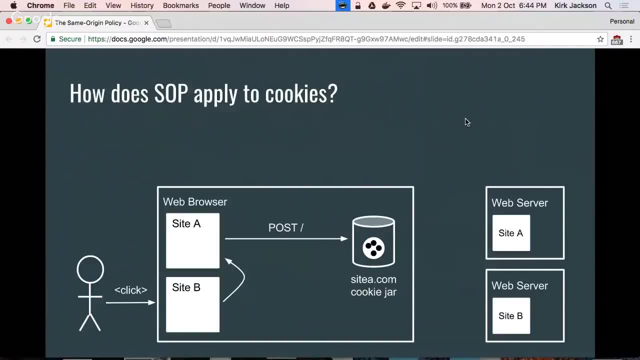 is. there's the form sitting in site B in your web browser. when you click on the submit button, the page is actually going to site A's web server. as the context of site A, it grabs the cookies and it sends the cookies along to the server. so site B is actually able to kind. 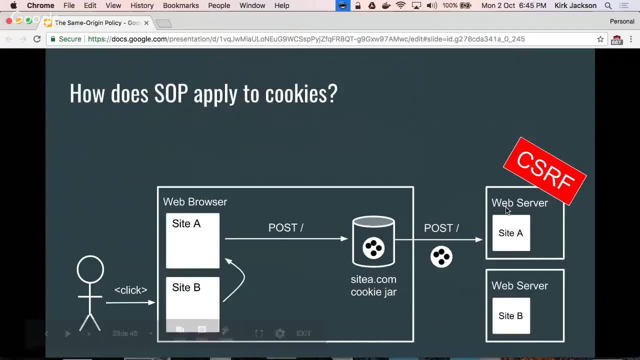 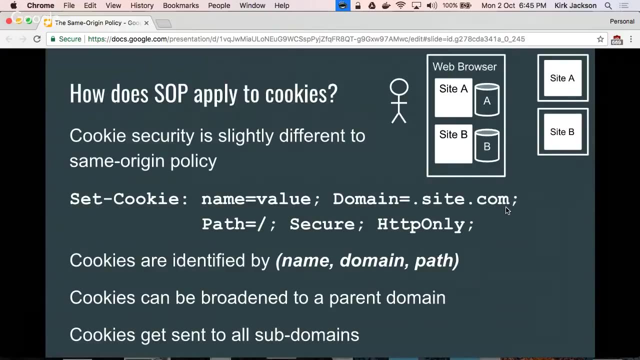 of post to site A with site A's cookies because the browser adds them on automatically so that enables a cross site request for drew attack. so cookie security is slightly different in that there's this latent authenticator, which is a cookie which gets passed along with your requests automatically. 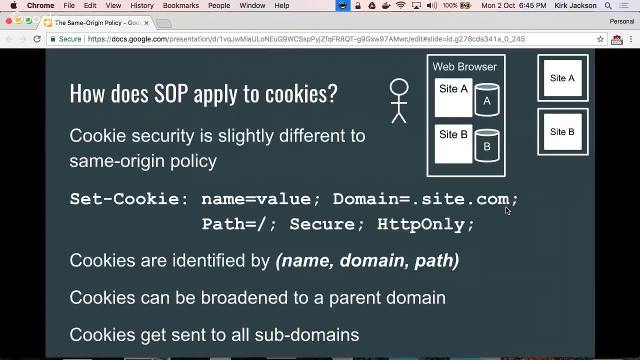 and also the way that they're identified is different. so when cookies are set, they have a name, they have a domain, they have a path and they might have some flags. cookies are actually separated by name, domain and path, which is different than scheme domain and port- that same origin. 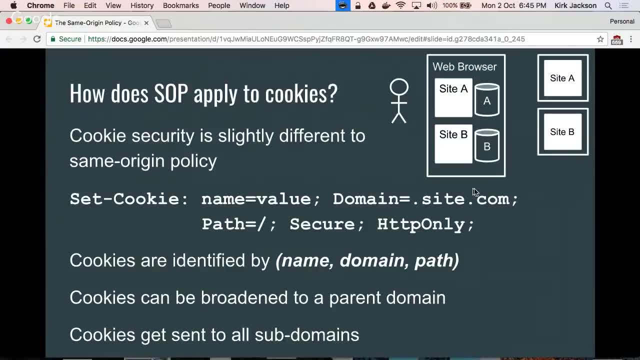 policy has, and so that means that, potentially, HTTP and HTTPS cookies can be accessed by either site, or that sites running on different ports on the same server can access the same cookies. and there's another little trick, which is that you can set a cookie on your subdomain, so if your site is 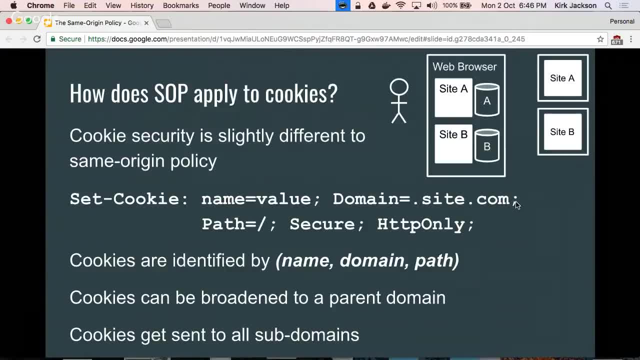 abccom, then you can set a cookie for ccom, and anyone else's site that is xyccom or pqcom will get those cookies cool. so that's kind of how. cookies are a little bit different, but it's the same kind of idea. 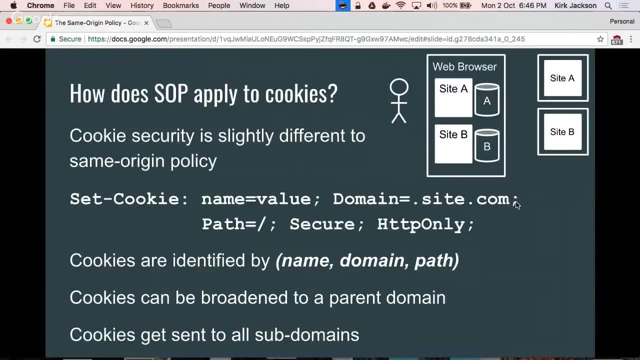 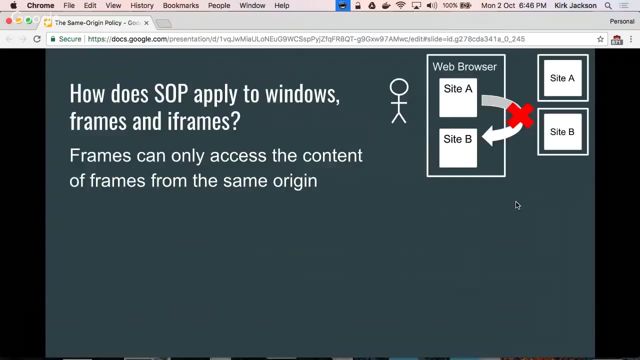 the idea that cookies are restricted to a particular site or family of sites. it's just the complication there is that the rules are slightly different. okay, so how does this apply to windows frames and iframes? how does the same origin policy apply? well, we've already covered this. 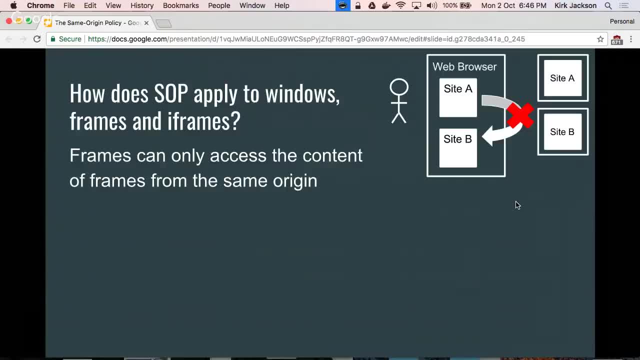 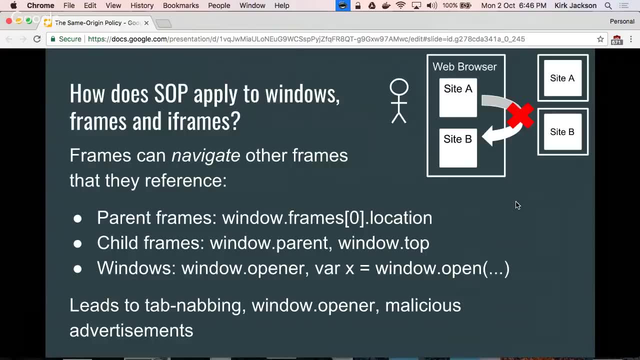 frames can only access the content of frames within the same origin, so when we had the two site a's open in different tabs, they could access each other. you can navigate other frames by changing the location and you can also reference other frames so parents can reference the children. 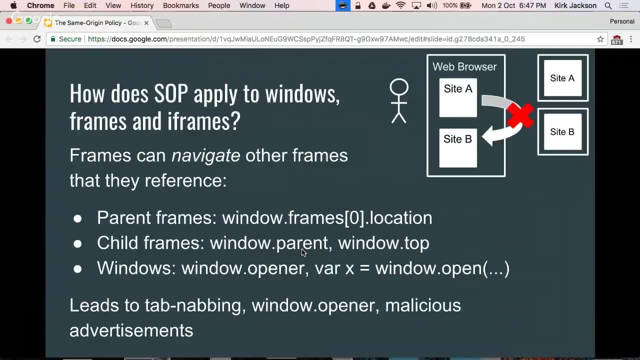 windows can reference the page that opened them, and actually being able to change the location of frames leads to some attacks that you might find out about furthering your journey, like tab nabbing and malicious advertisements that take over your browser and stuff like that. I'll show you briefly one. 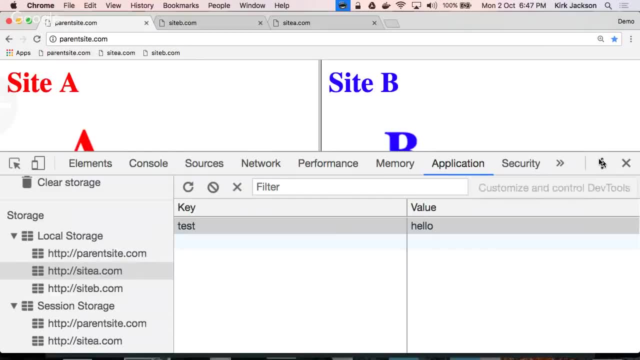 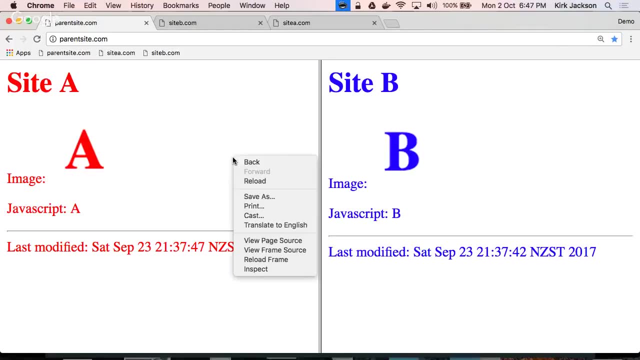 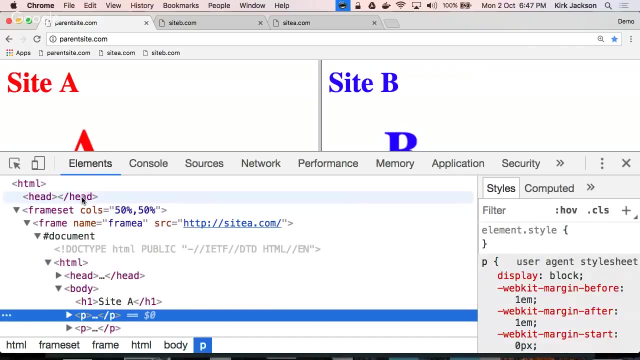 so let's go to our parents site. so say parents site has two iframes, one of them is an advertisement sitting on the right hand side. but say that advertisement is malicious and it wants to take people to a fake google login page. then in that child frame, 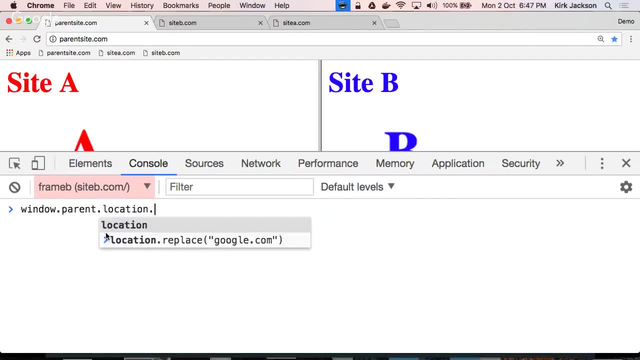 site b, it could go window dot. parent dot, location dot replace and send you to a fake google login page which looks remarkably like the real google login page, and so you might switch to a different tab and then, when you come back, the advertisements changed the parent frame and you'll go. 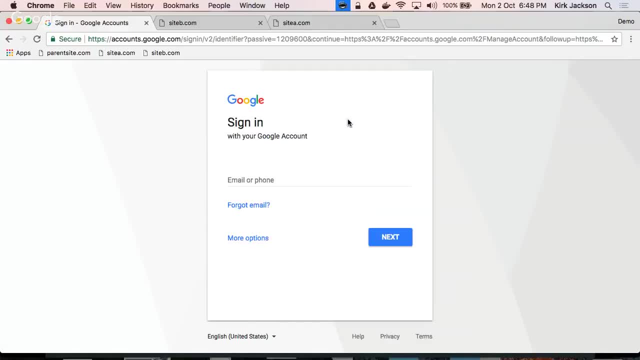 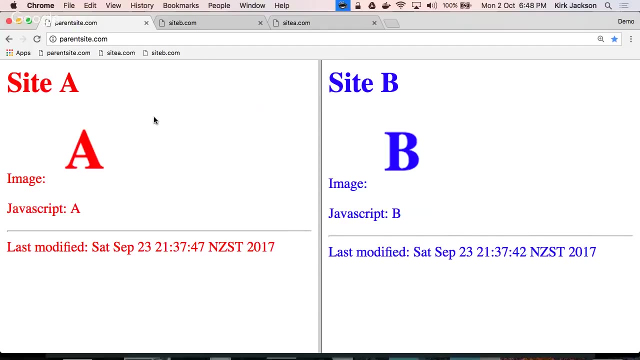 well, that's weird. I'm sure I was logged into google before and you'll log in again, except this might be an attackers website that you're logging into, not the real google site. so that was a tab nabbing attack. another one is abusing window dot opener. so if you follow a link to 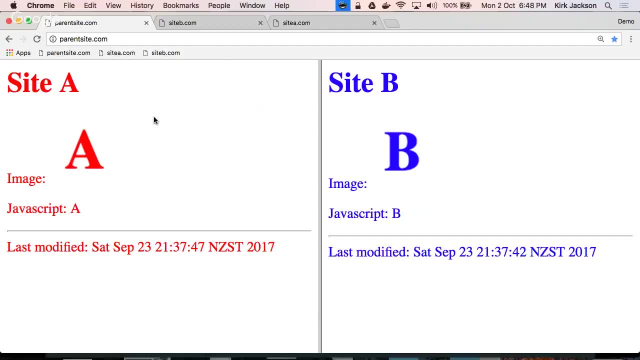 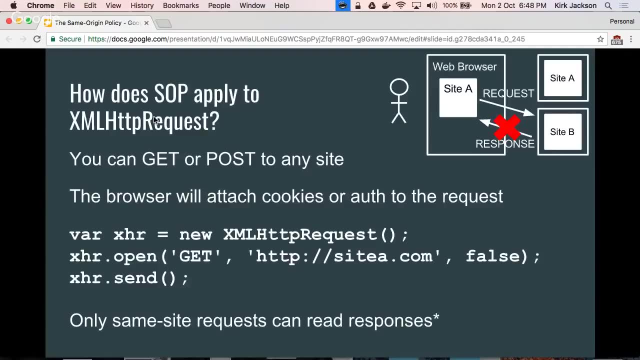 another page. that page can change the location of the person that opened it. so there's a few kind of attacks that you can look out there. okay, so now getting into the interesting bits, where you're using javascript to request data from your server. so the interesting thing about 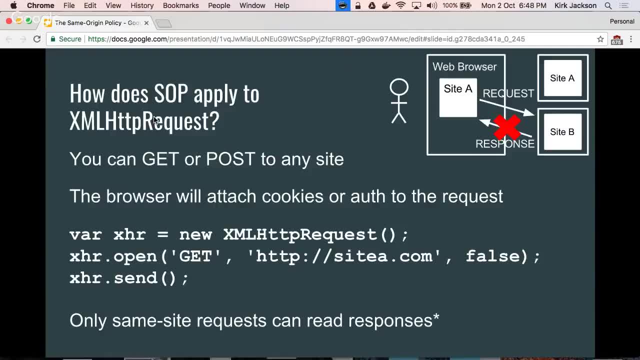 web browsers is they'll let you send data to any website so you can post a form to anywhere on the website. you can send an xml http request to any website. the browser will let your javascript code send data to anything it wants, but it won't let you read the response. 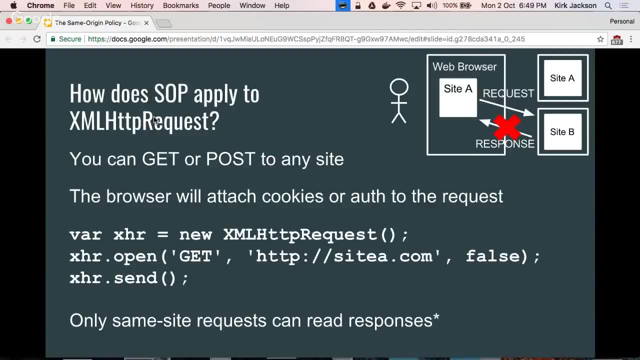 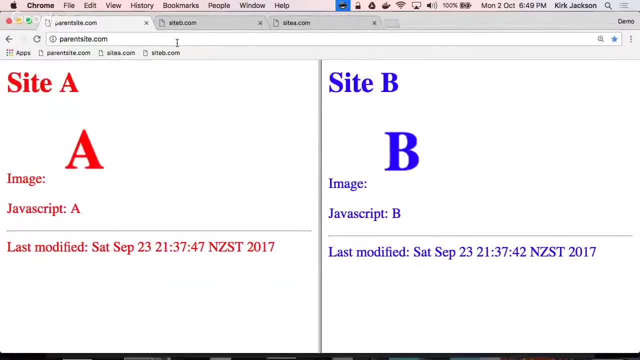 because the response is the sensitive stuff that that server might send back. so that's why there's a big x there. so let's just look at how that works. i think i've got okay. so you've probably done like ajax type stuff before, where you make. 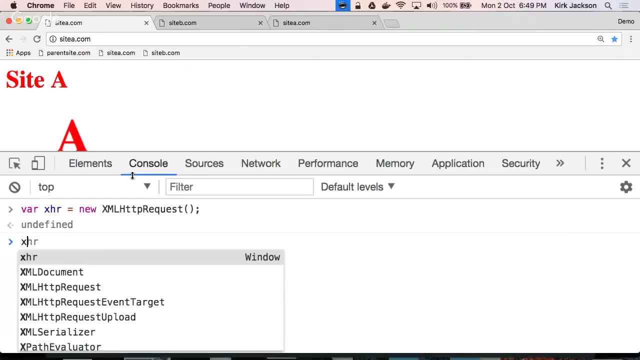 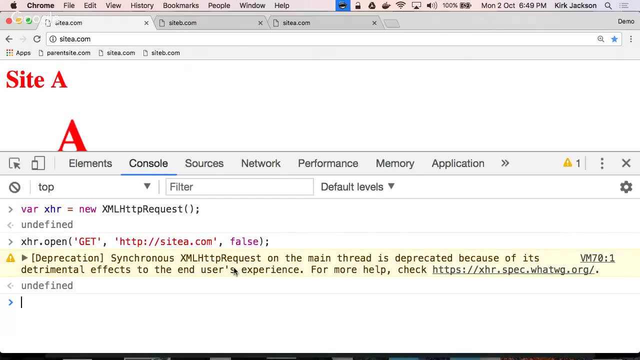 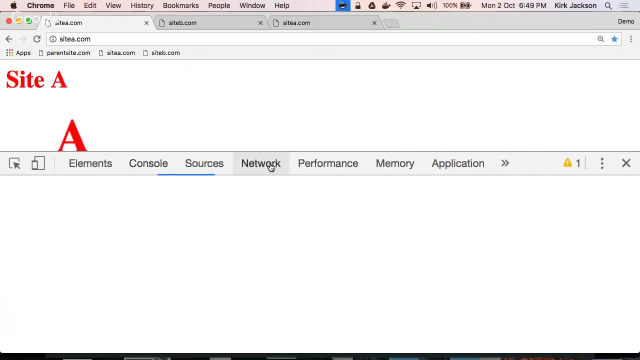 a variable which has an xml http request object and then you see the url that you want to open. so i'm in site a and i'm trying to request site a. i'm using the version, but same thing. so if i send that request, let's see what happens. 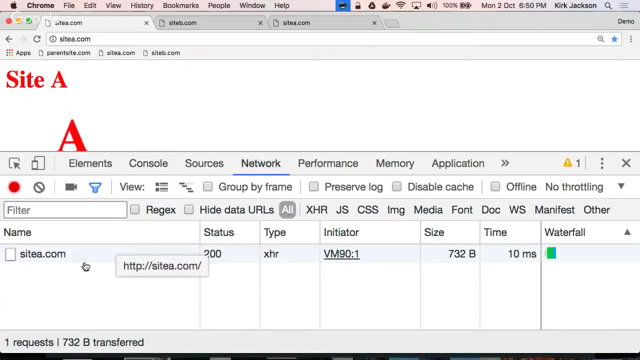 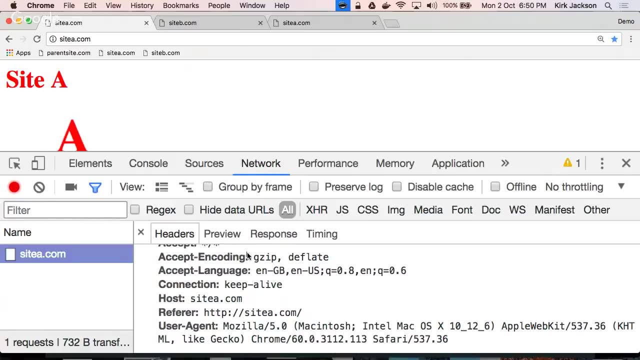 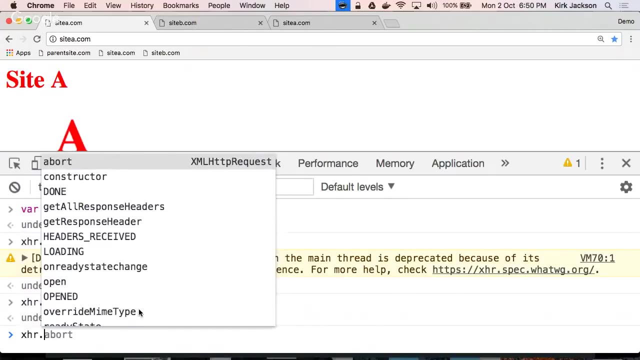 in the network. so site a dot com sent a request to site a dot com which returns some html. that's kind of what you'd expect. maybe you're getting some jc or whatever and from javascript. after i've sent the request, i can read the response and: 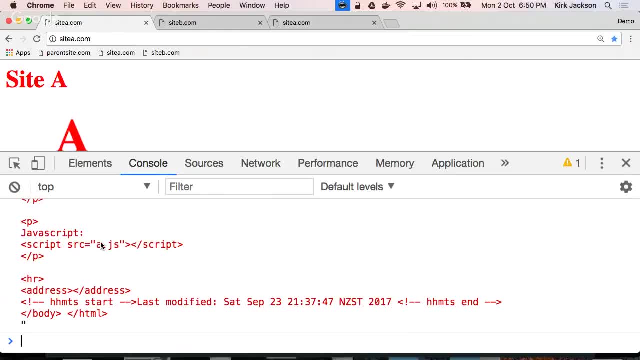 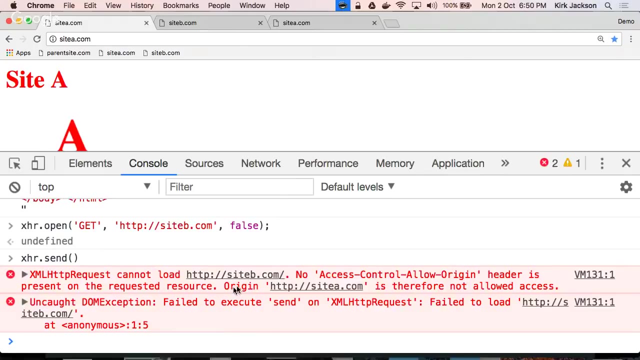 see the data. so that was requesting data from my own site. that's allowed. what if i tried to request data from a different site? so now i'm going to try and get some from site b, which is a different origin and there's an error. so xml http: 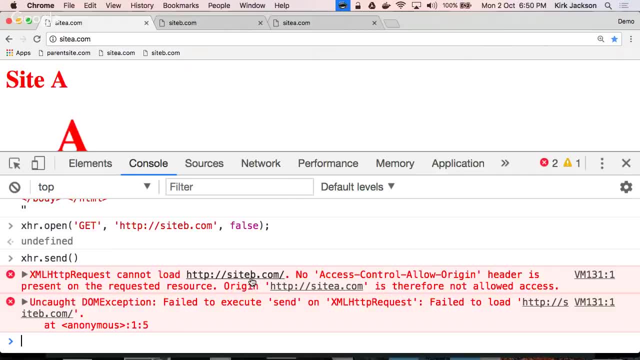 request cannot load site b dot com because it's not allowed access and there's some other errors. talks about access control allow origin, which we'll discuss in a sec. but basically this is same origin policy, saying site a is not allowed the data of site b. this is good. 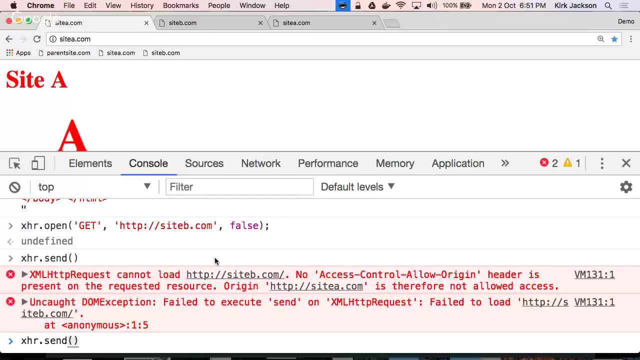 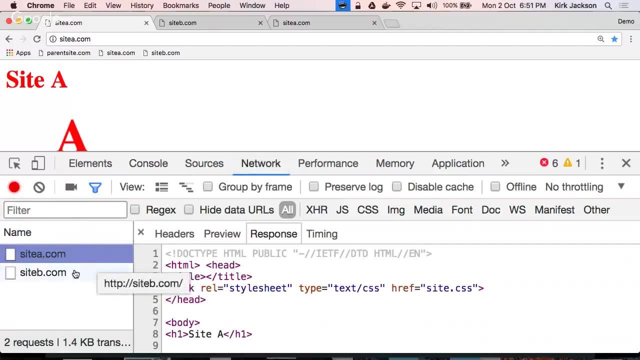 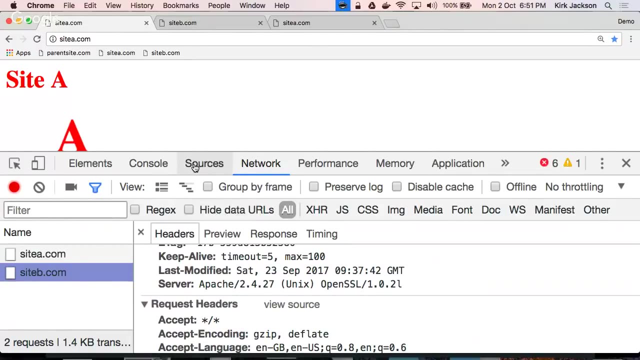 cool. the interesting thing here was: i'm trying to call site b right. the browser, my javascript code, is sending requests to it. um, in the network tab. um, my requests to site b are actually happening. um, and it is actually site a is making a request to site b. 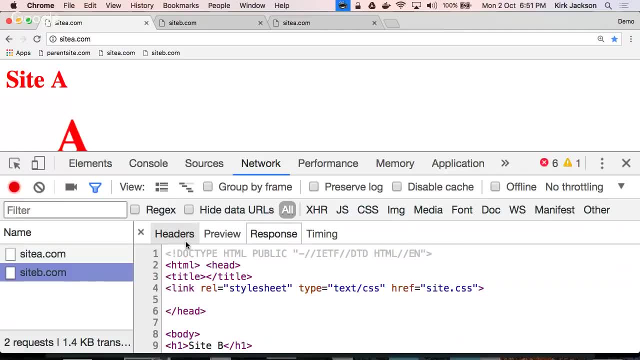 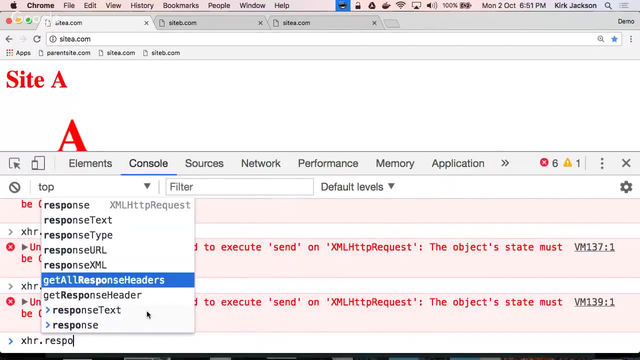 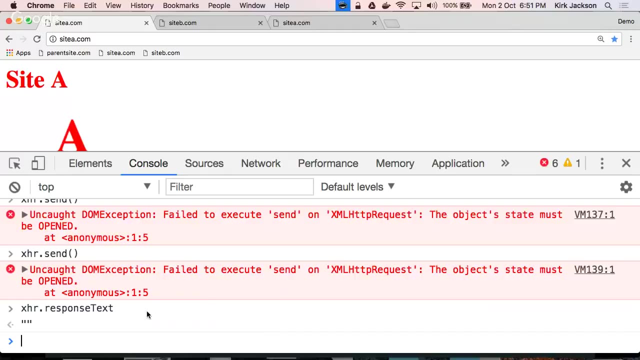 getting a response from site b and then the browser is not letting javascript have the response. so if i try and look at the response, um, where's text there? it's just giving me an empty string and it's giving me an error. so yeah, so it's the. 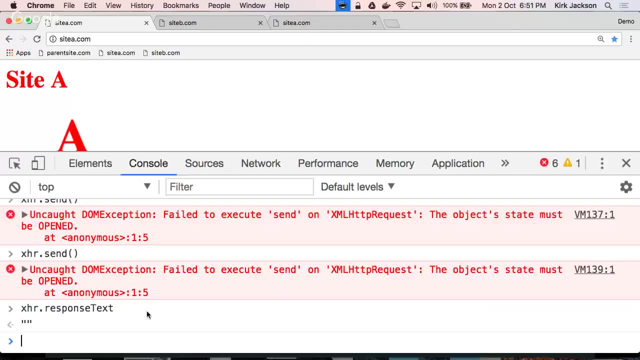 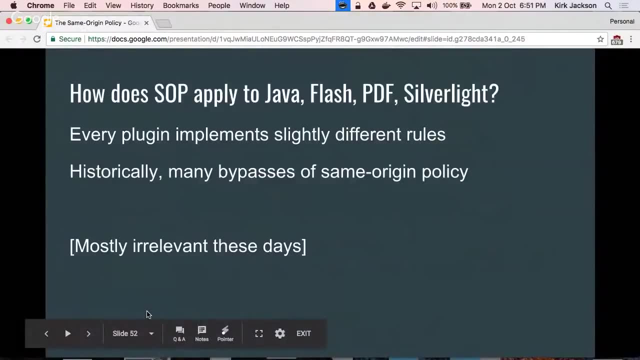 browser. that's enforcing it. it's not stopping the request from going, it's just stopping it from looking at the response. cool, um. so other browser technologies that you don't really see in 2017, um, that are kind of quirky, are java applets, uh, flash. 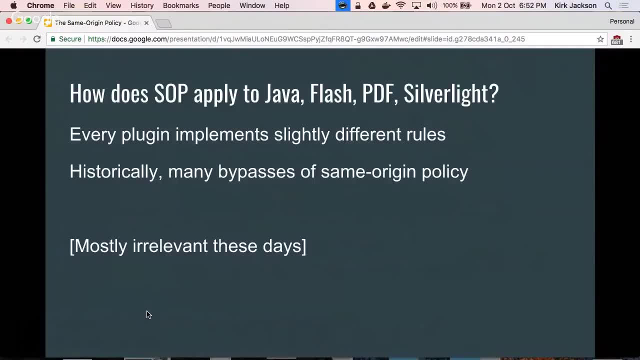 applets. i guess um pdf like acrobat reader, um. inside pdfs javascript can run, so if your pdfs open in the browser it runs in it. um or silverlight, which is also dead. so these all have different rules from the standard html way of defining. 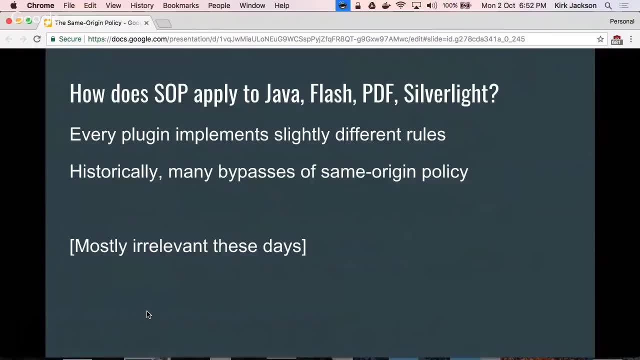 what an origin is and what they can access, um and um. you know, going back through history, there's been lots of kind of attacks: um on one site attacking another by using a malicious java applet or using a malicious flat flash applet, um. but that's mostly irrelevant these days because 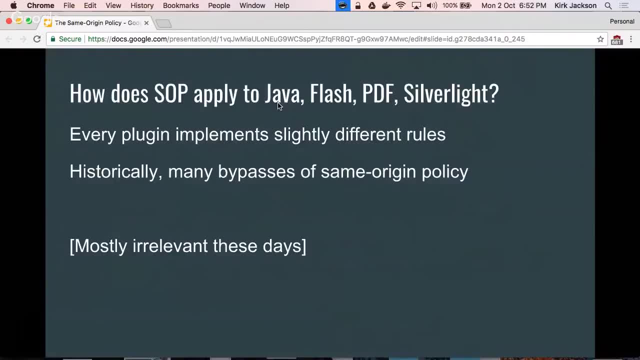 um, both browsers don't support any of these things anymore. um, so i'm not going into it. um, if you do want to get into, uh, the quirks of flash and and java, um, this book, the tangled web, is really good. um, so it's, it's a little bit old, it's from. 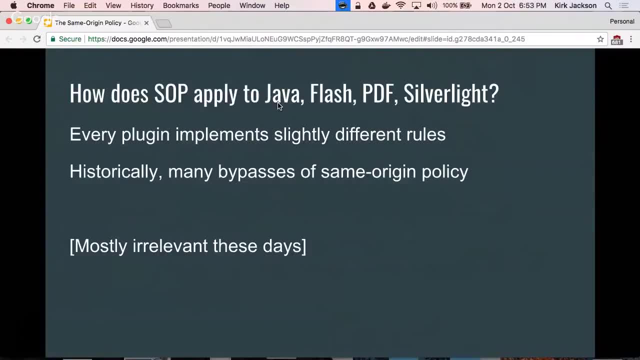 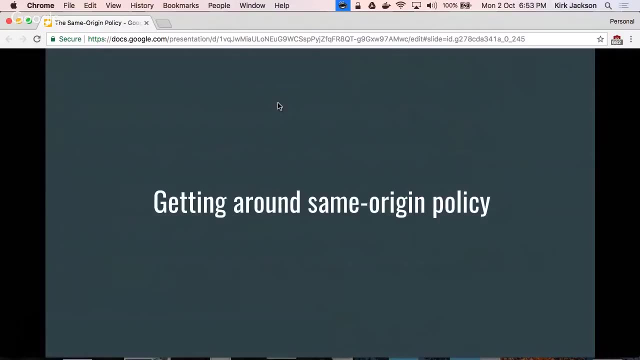 uh, 2012. um, but um, it's a really good reference for how browser security works and you know what weird rules apply to java and flash and and everything else. um and uh, we'll give away one of those at the end of the session. um, so that was a run through a bunch. 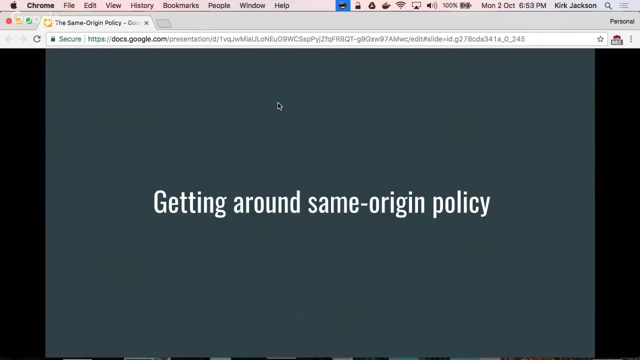 of different technologies and how same origin policy works. um, so how do you get around this? like what happens if you're writing an app where you want two frames to be able to talk to each other or you want to be able to access data from you know? uh? 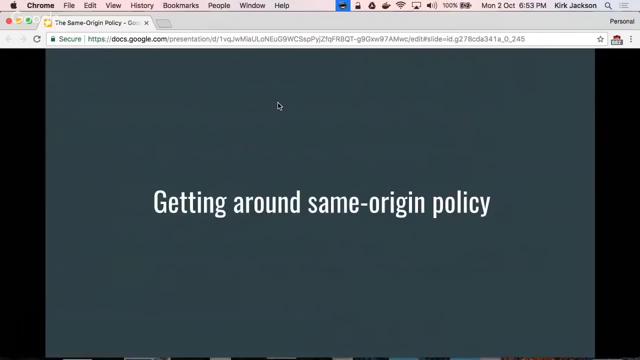 datayoursitecom from. you know websiteyoursitecom. you know you want to share data between different sites. um, the only way we've seen that you can do that is with jason p and i mentioned. that was kind of a hack and kind of ugly. 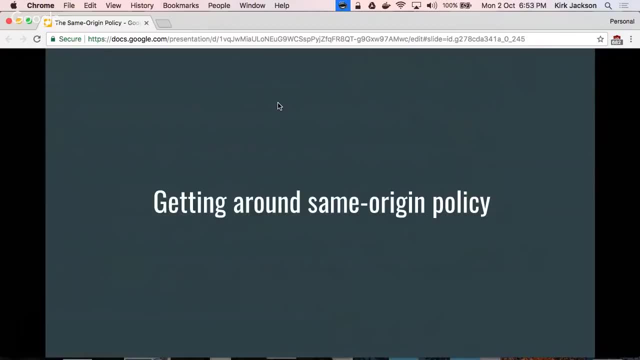 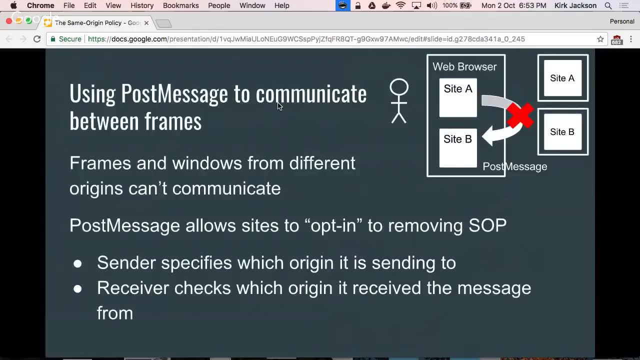 uh, so the web standards bodies have looked kindly upon us, um, and have come up with two different ways of doing this, um, the first is post message and that this technology allows one frame to talk to another frame, so a frame or a window or an iframe to talk to another frame or window. 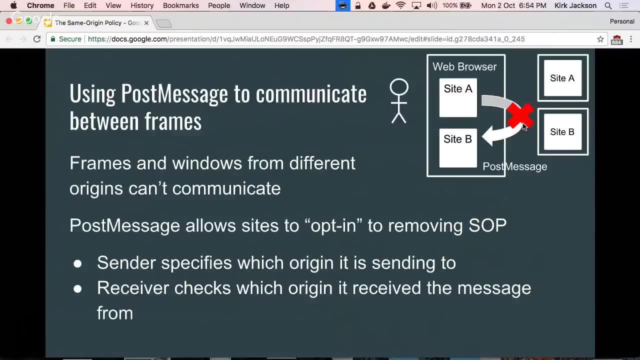 or an iframe. so normally, uh, frames can't talk to each other. we've seen that, um, but if you use this post message api, the red cross goes away and you're left with an awesome arrow with a gradient. um, so sites can opt in to this um api. so 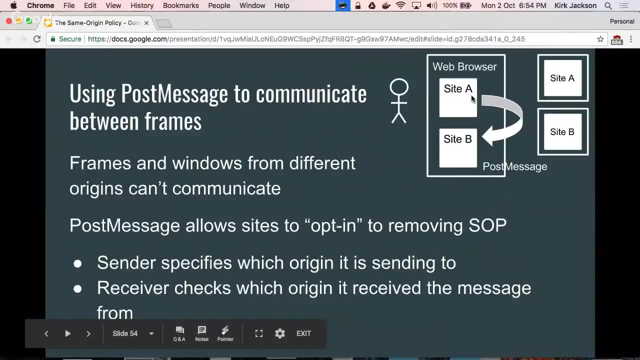 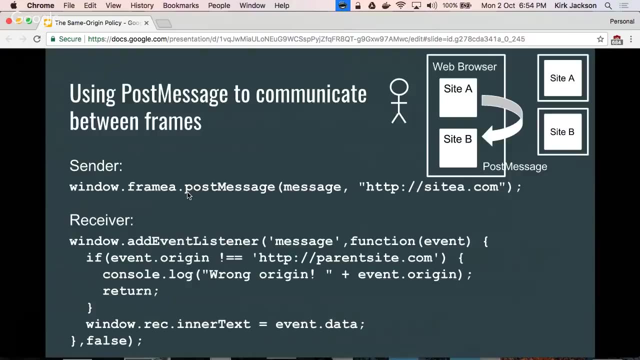 the sender: um. site a sends a message, site b can ignore the message, um, or it can look at the origin to see that it's coming from the right person, the right website, um, and then decide what to do. um. here's some code. i'll show you it again in the browser. 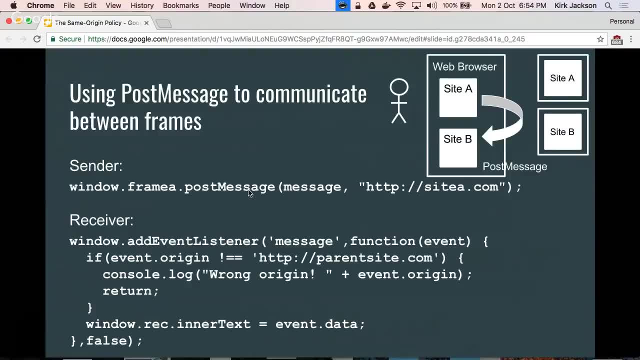 but basically it's: uh, the first site goes post message um with some message text which could be json or whatever um, and specifies um who it wants to send it to, um. so this is what. this is the origin of the other frame. so it's not sending the message to a server. 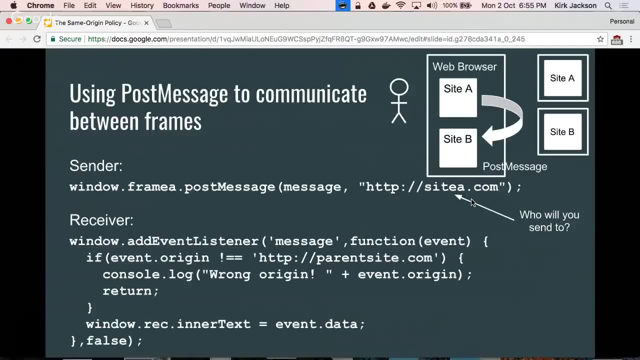 it's sending it from one frame to another, so it's javascript talking to javascript, but it it's saying: i only want to send this message to site a, not to site b or anything else, and then the receiver um adds an event handler to listen for messages that come in, and it: 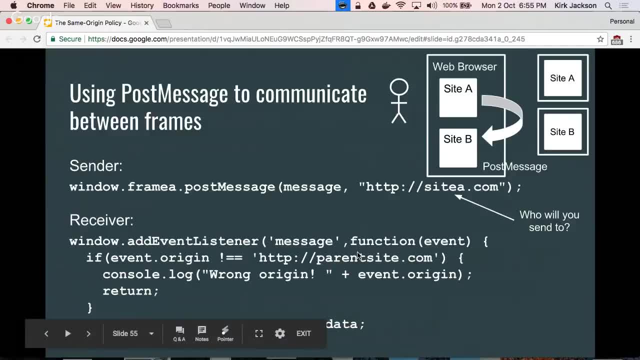 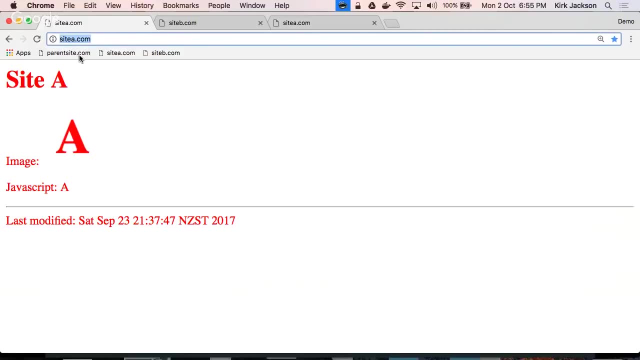 can check that it's receiving the message from the right origin and then do whatever it wants with it. uh, so it opts in by adding the listener and it can do security checks to make sure. uh so have a look at how that works. um, uh, post message. 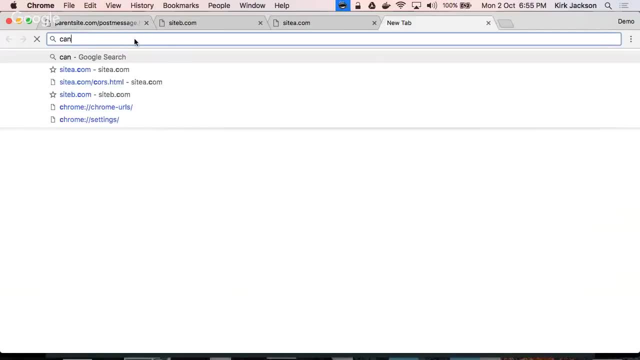 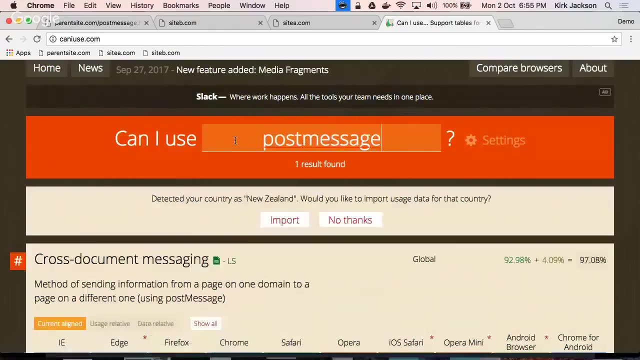 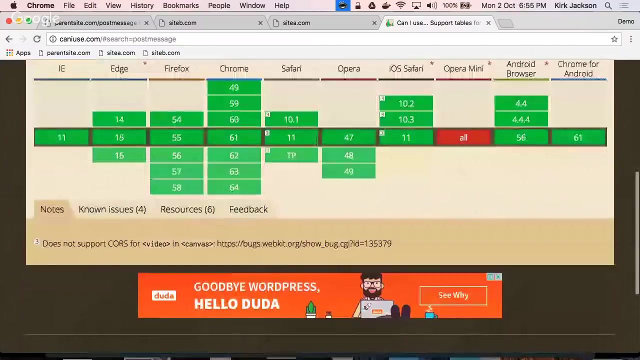 is pretty well supported. uh, let's go. can i use dot com? um post message has been around for a while, so i'm gonna say, yeah, it's pretty much green across the board. and while i'm here, uh cause, which we're going to talk about in a minute, is: 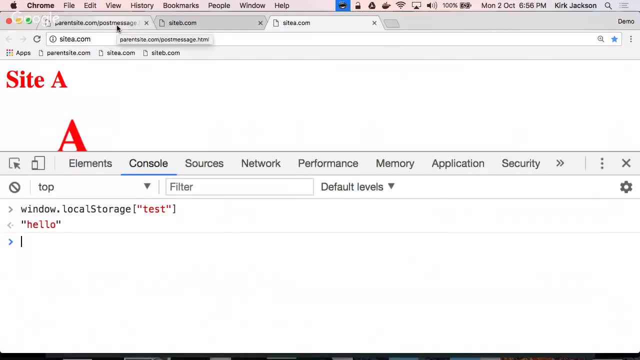 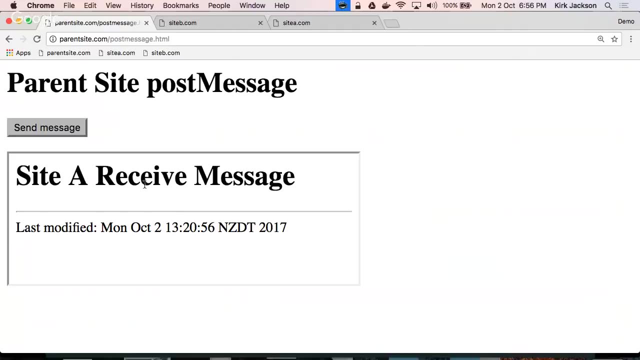 also green: um, across most modern browsers. um, cool. so here we've got a parent frame and it wants to send a message to the child frame. um, the parent frame is parentsitecom and the child frame is siteacom. uh, so just to prove i'm not lying. 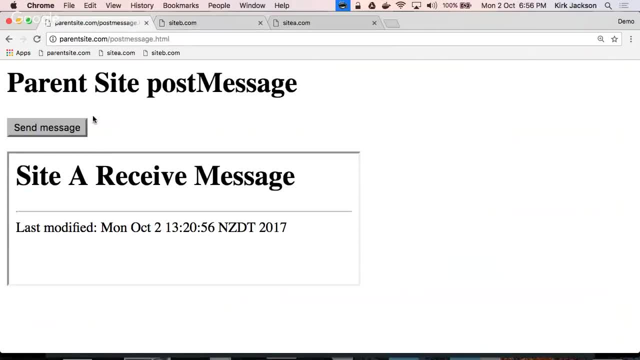 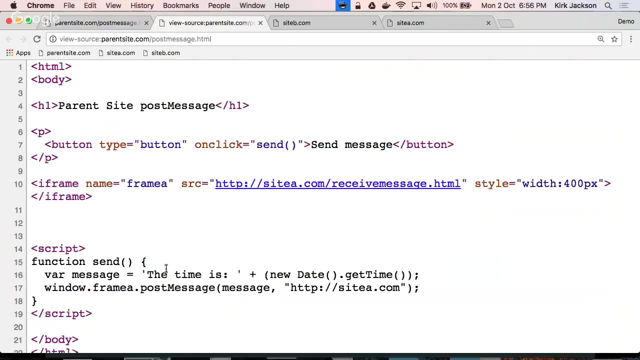 um, siteacom slash receive message. um, so when i click this, um, the parent frame is javascript is sending a message to the child frame with a timestamp and the child frame is displaying it. um, so how that works is, uh, when i click send, it's going post message to. 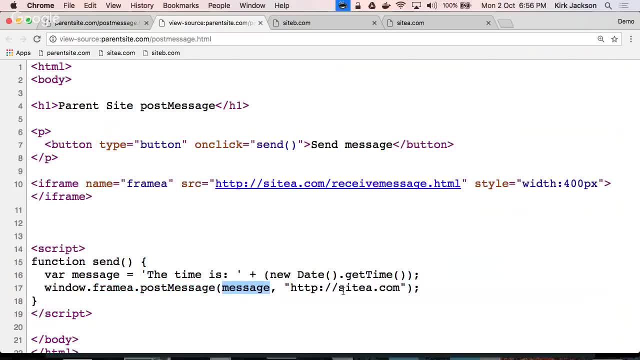 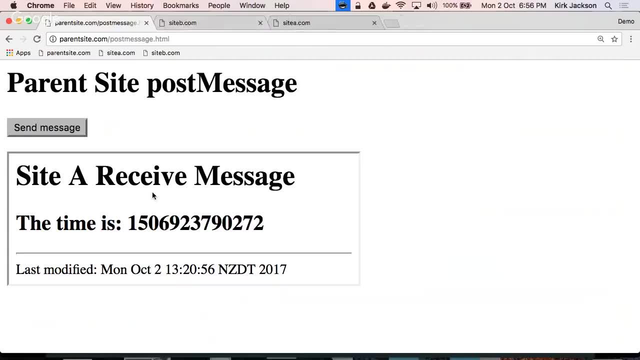 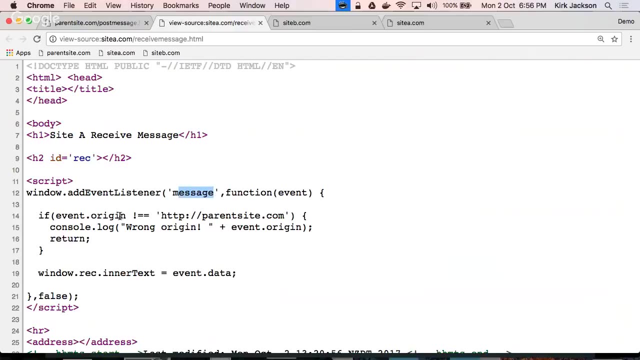 the child frame, passing that time and saying this is the only frame i want to send it to, uh, frames that have the origins siteacom, um. and the child frame um has attached to listen to messages that come in and it's saying i only want to receive messages from parentsite. 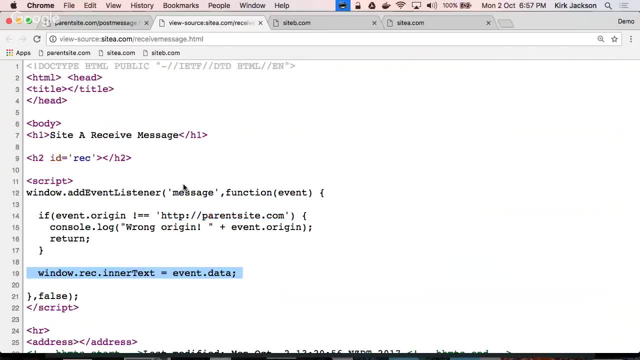 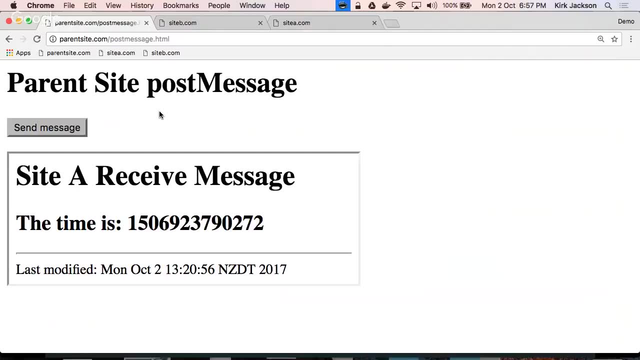 and once it receives them, it's displaying it on the page. um, so i've labored this. uh, you know the origin checks for the sender and the receiver, and i'll just talk about why that is. so say that, um, someone managed to trick siteb to. 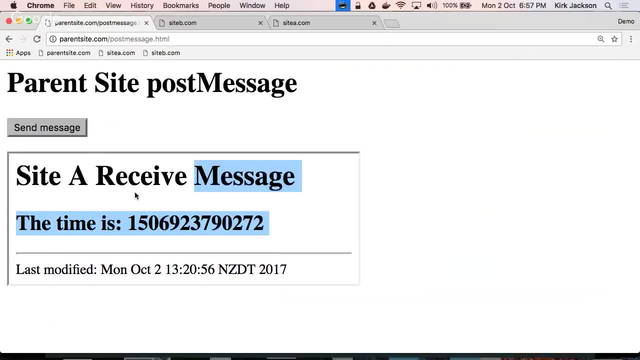 redirect to their own evil site so that they could receive messages from the parent. so say, you had um two frames on your site and they both had sensitive data on it, but one of them had cross site scripting and you're able to change its url or whatever to your. 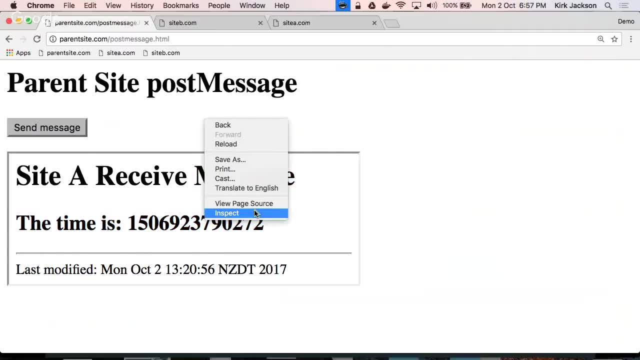 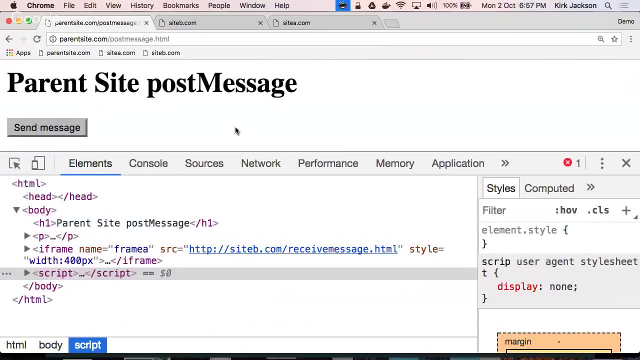 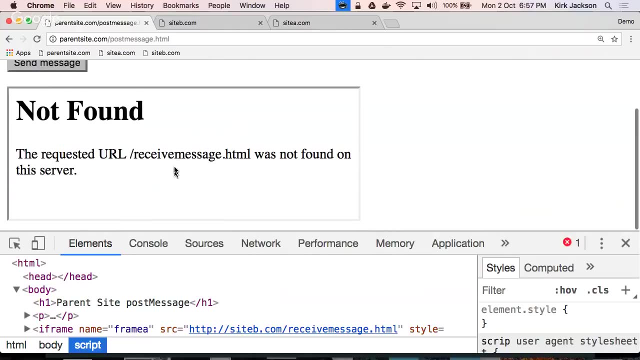 attacker website. um, let's reproduce this scenario by changing the url to siteb of the iframe. oh, that page doesn't exist on siteb, but you kind of get the idea now. um, when sitea tries, when the parent site tries to send the message, the browser, 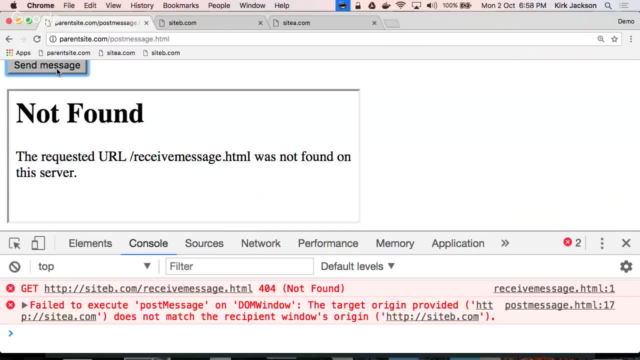 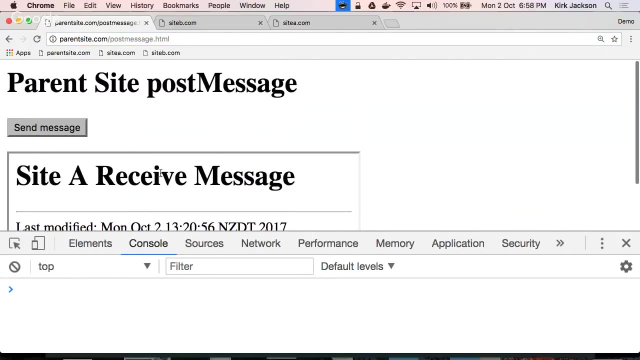 is checking, you know, is the target that you're trying to send to? is it siteacom? and it's giving an error because it isn't, it's sitebcom. so, basically, the browser is enforcing, uh, that um relationship. now it's the same. what if your sensitive? 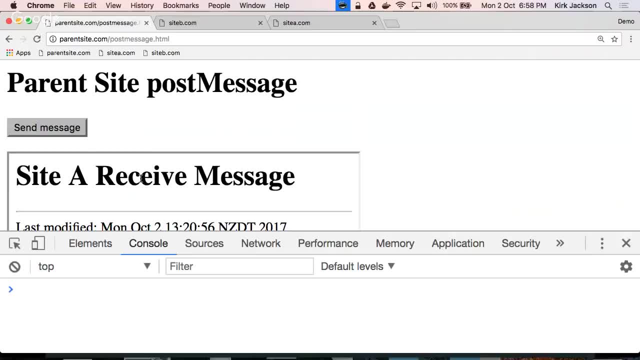 stuff is in sitea and you don't want to receive messages from anyone malicious, so some other site might wrap you in a frame. you don't want them to be able to send messages to you because you might trust it and do something. um, so siteb has. 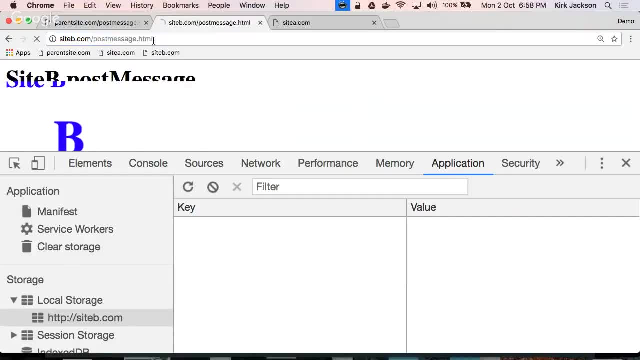 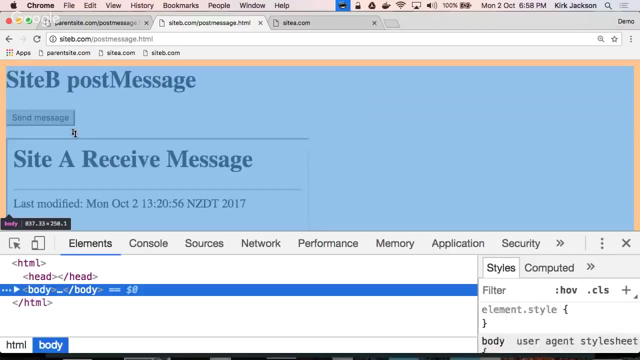 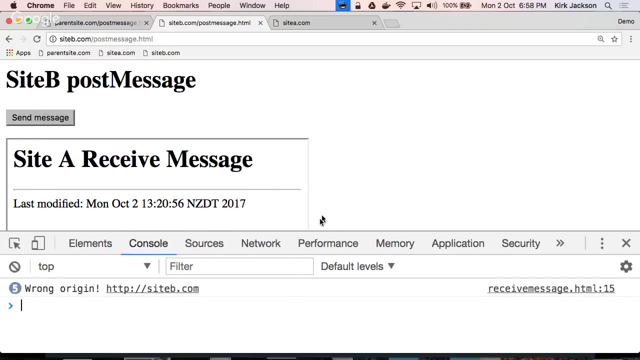 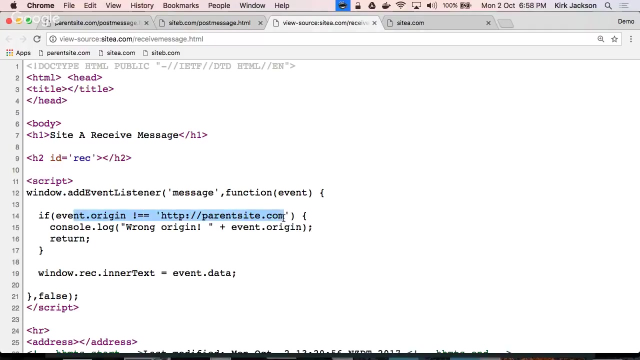 um, a malicious page where it has wrapped sitea um and so siteb is allowed to send the message to site a, but site a is doing that. check that. i showed you frame source um. if the event origin isn't who it expects um, then it's erroring out and you can see. 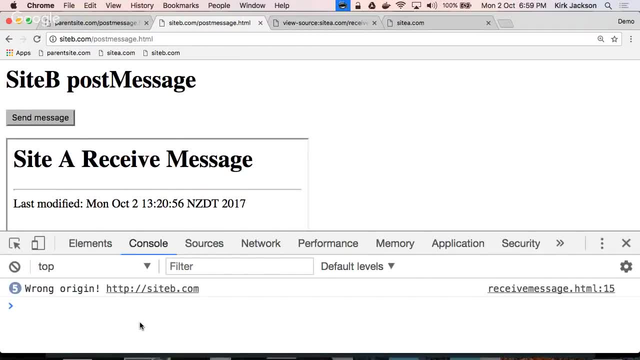 those error messages coming up in the console, um. so likewise, it's able to check who the parent is, that's sending it messages. if you didn't have that check, that means that you would be able to receive messages from anyone that wanted to post them to you. so that's. 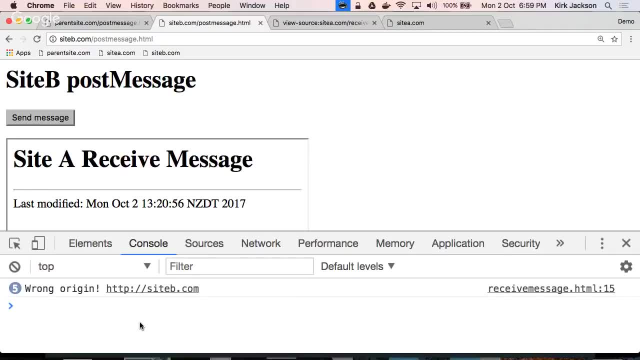 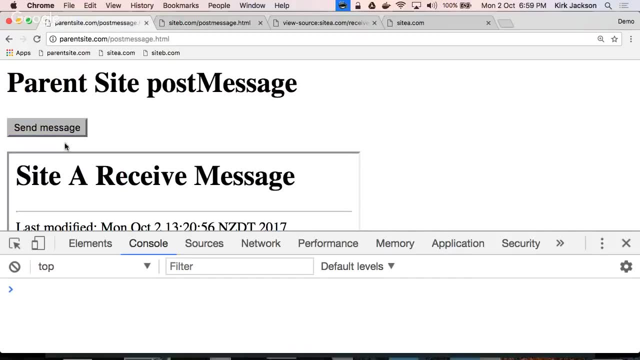 that could be fine, depending on what you're doing with the messages, um, but i guess here sitea is receiving some text- well on the one that works- and just sticking it straight on the screen. so if i was able to send it javascript, it would just display that on the 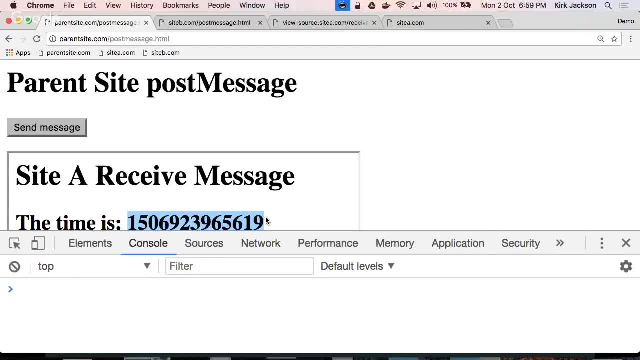 screen. so if someone bad was wrapping my site, they could send malicious content um to me, um. so i want to protect against that and explicitly whitelist. now, when you look into how post message works, there's ways to um. you know whitelist more than just one origin talking to another. 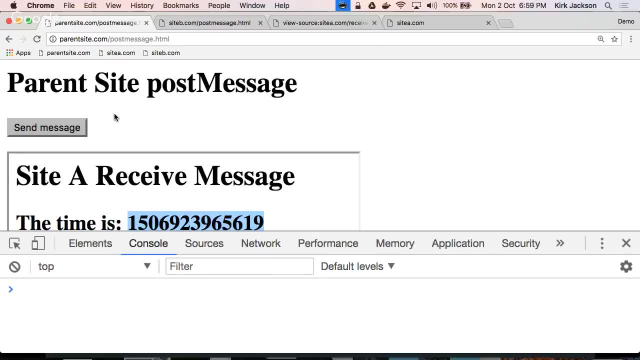 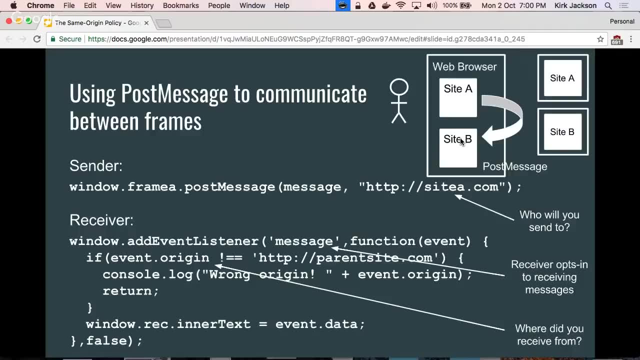 origin so you can look at the docs for how that works. cool, so that's to let you send data from one frame in your browser to one frame, to another frame in your browser. um, so places, i've used this before. um, we had, uh, oh yeah, we had like a help thing which was on a 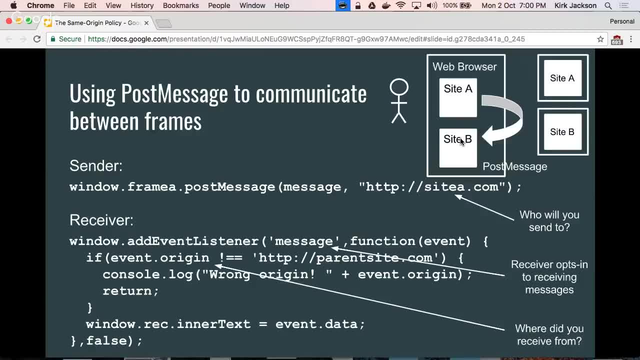 different domain name and when someone typed into a text box we wanted to display search results, um, and they were on different domains. so the way that we passed the search query from one to another was by posting the search string to the other one. um, and we actually had to call. 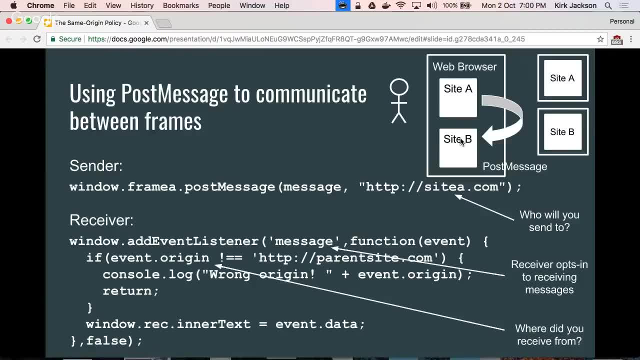 back and forward. so i had another thing where i think the child frame had a button saying expand me, um, and so i had to send the message back to the parent and say can you make my iframe bigger? and then the parent would resize it. and then you click another button to say make me smaller. 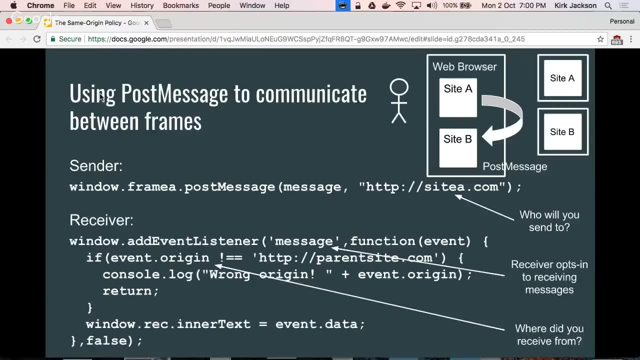 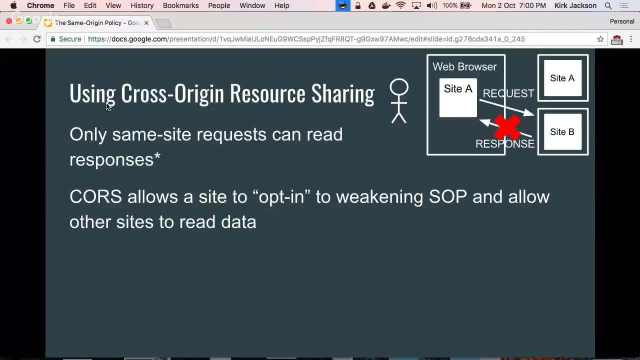 and then the parent would make it smaller again. um, cool, um, and so the the alternate, i guess, just communicating within a frame, within frames- is to actually request data from one server and read the response. um, so this might be. uh, you know, you've got an api that you need to call from your app. 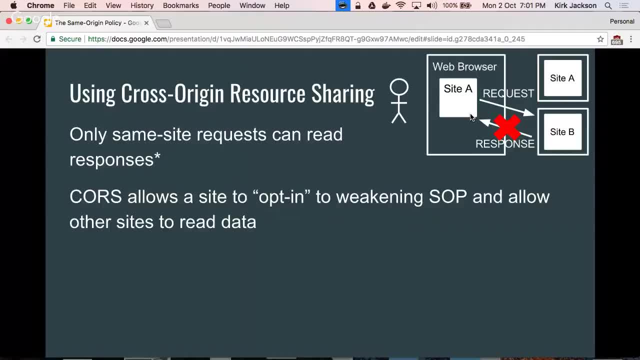 so you might be calling- i don't know- google's latitude to longitude, to location service or something like that. so you need to call an api and you need to be able to receive the response. um, so normally that would be blocked. you could call google server, but you. 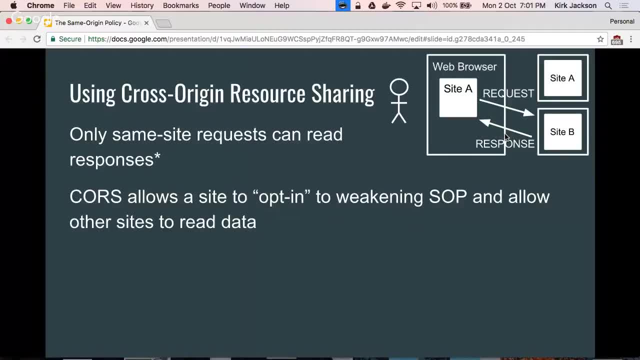 couldn't see the response, um, but we want to turn off that and read the response. so here the onus is on the receiver, the server, site b, to allow people to receive, uh, to send queries and read the response. um, site b is the one that can make the decision based. 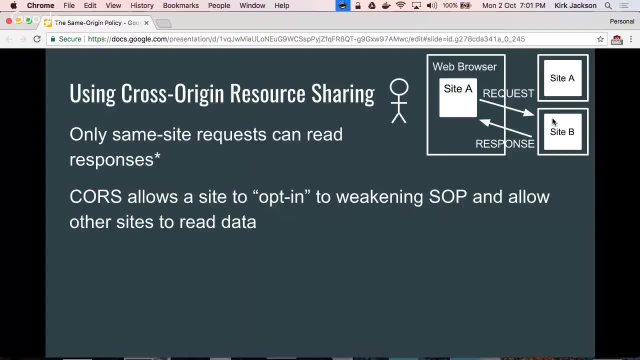 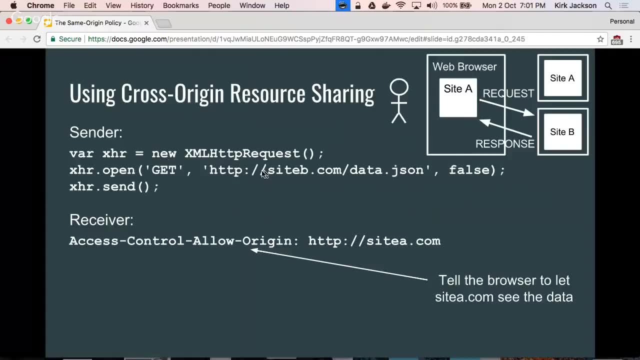 on. you know, is my data secure? will i let people see it um? so how that works is: the sender makes a normal xml http request um asking for some data and the receiver sends a new http header called access control. allow origin, um and its response and the browser looks for that. 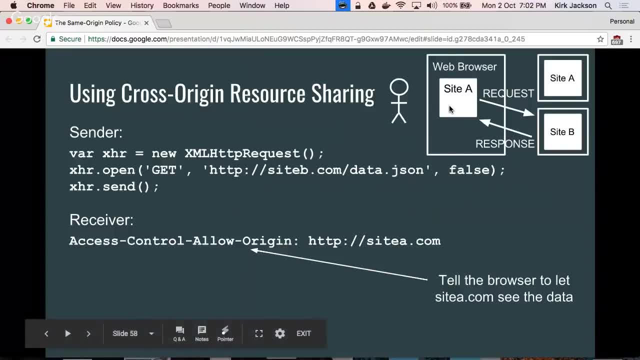 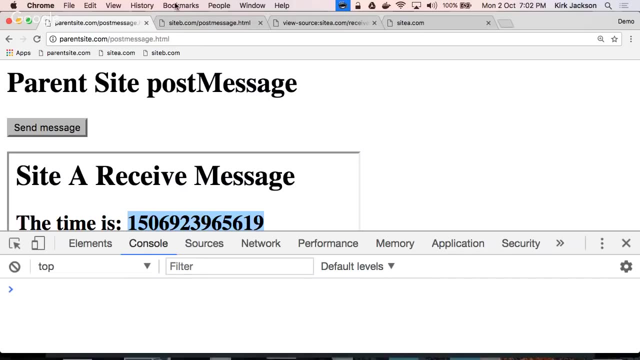 if there's no access control allow origin header, it won't let site a read the response. if there is and it matches site a's origin, it will give the response to site a's javascript. um, so the again the browser is enforcing this. uh, so what does this look like? 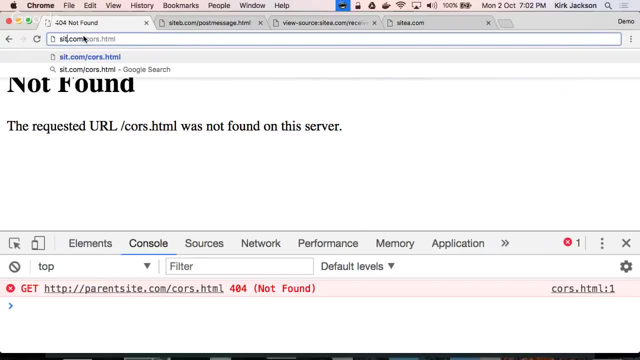 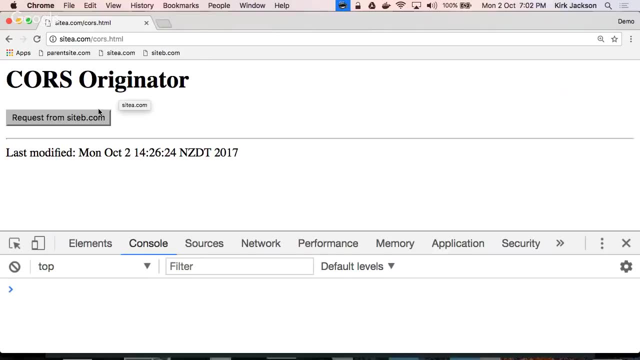 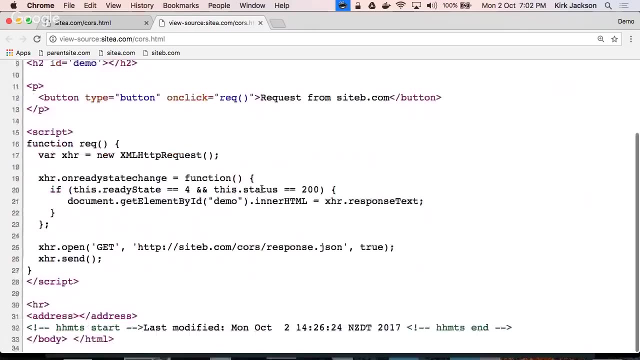 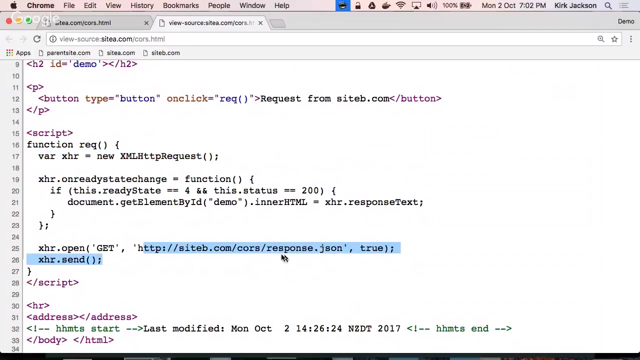 let's call it cause. um so uh, just to look at what this page does, i know this. examples are pretty simple. um, so this just creates an xml http request. object: request: some data from site b? um, when the object gets the data back, it displays it on the page by. 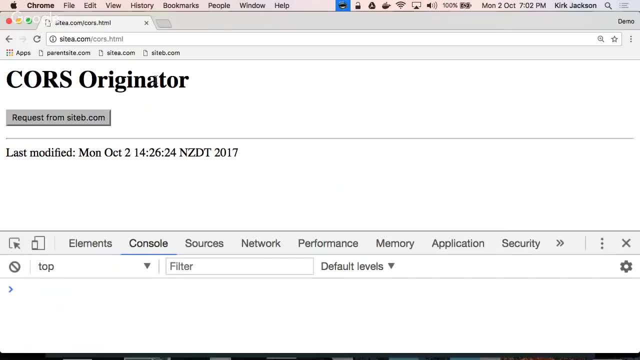 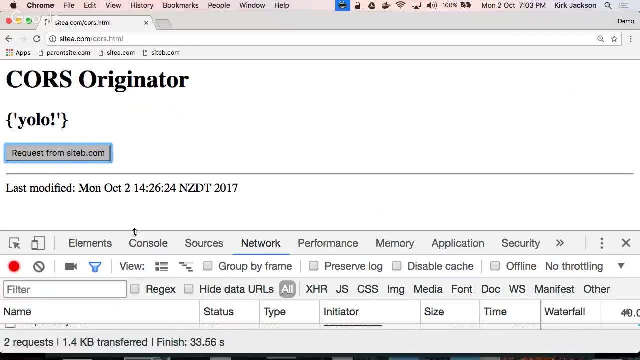 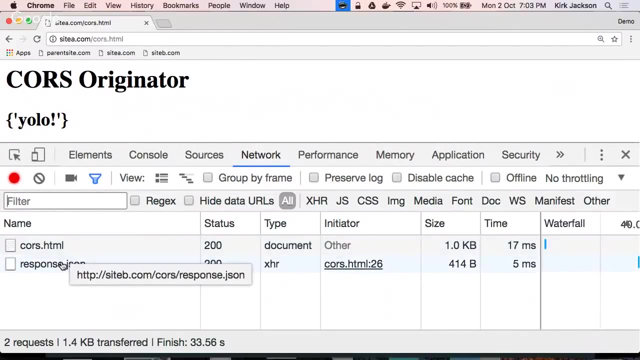 um, doing some janky javascript, um, so just to see what that looks like. um, uh, that requested the data from site b and if we we looked, um, there's site a being loaded, then there's the j, then there's the xml http request where site a is. 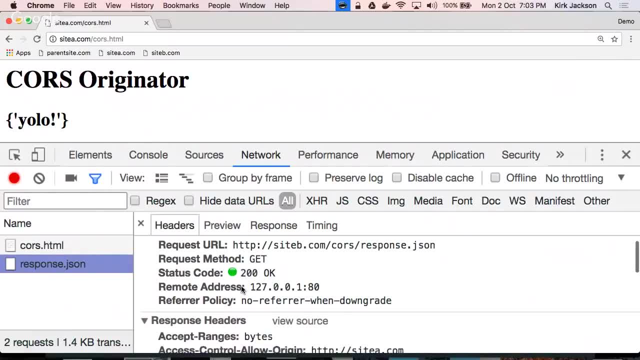 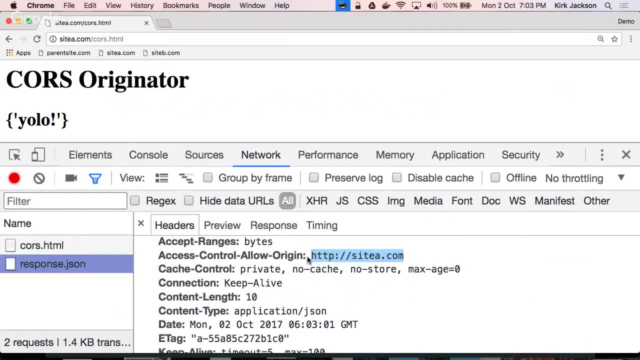 requesting data from site b, um, and site b and its response header is saying: i'll let site a uh receive that data from me, but nobody else, and the browser's enforcing it giving the data back. can that header be wild? can it have a wild? uh, yeah, so the question was: 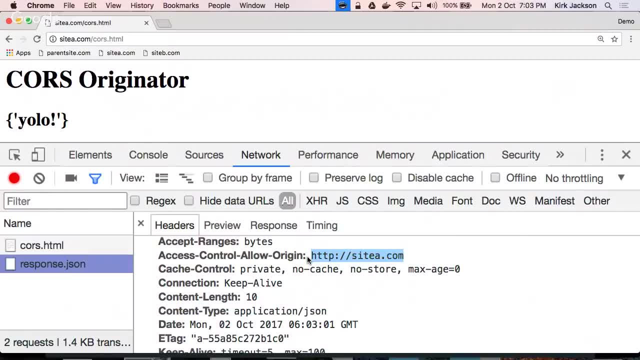 can you have wild cards in there? and yeah, you can. so um check out the documentation. um, if you put a wild card here, that means which is an asterisk? it means any website on the internet can ask for data from your server and get it back. so in some use cases that makes. 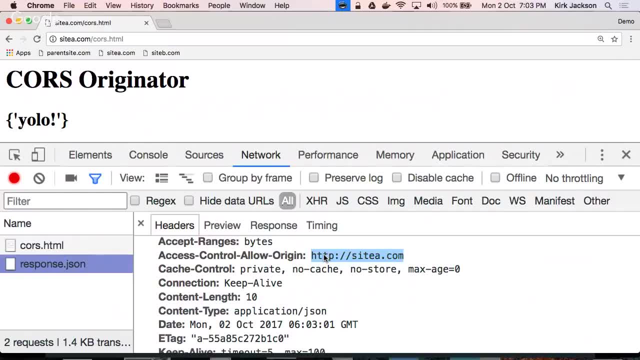 sense. so, like google's latitude and longitude to location service, they might be happy for any website in the world to call that um. but if the request is, you know like, give me my bank balances, you might not want to have an asterisk there, um, another thing that you can do. 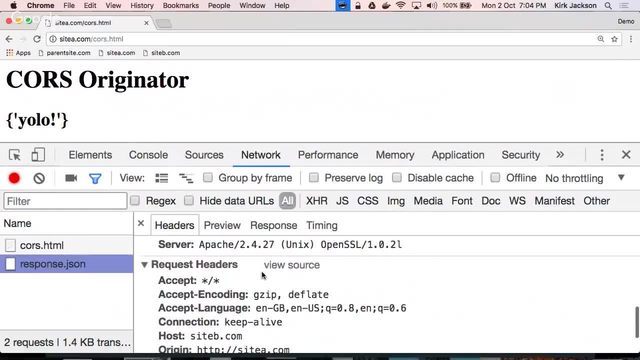 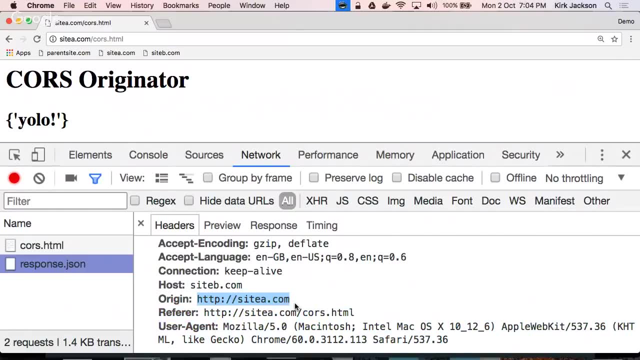 just while we're talking- and this is kind of like extra for experts- is um, when the request is sent to the server, it sends the origin. so the server gets the origin and its request and it can make a decision then as well. so site b can decide do. 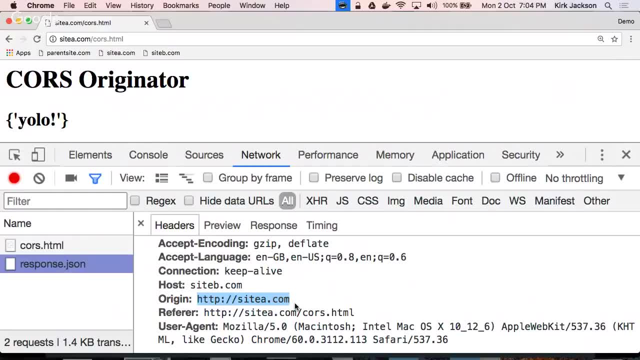 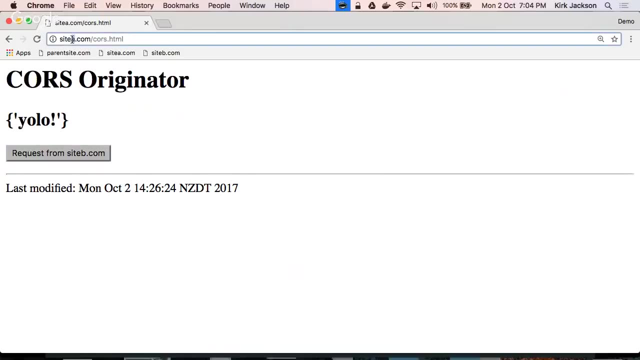 i trust site a who's asked for data? if i do, i'll send it back, um, and so the server can make that decision, or it can send the data back and let the browser make the decision. um, cool. so just just to show what happens when that head is not set. so 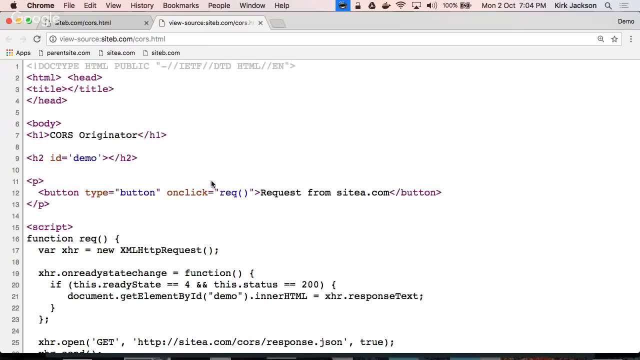 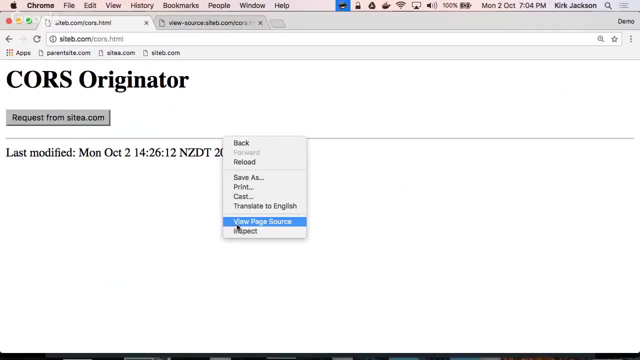 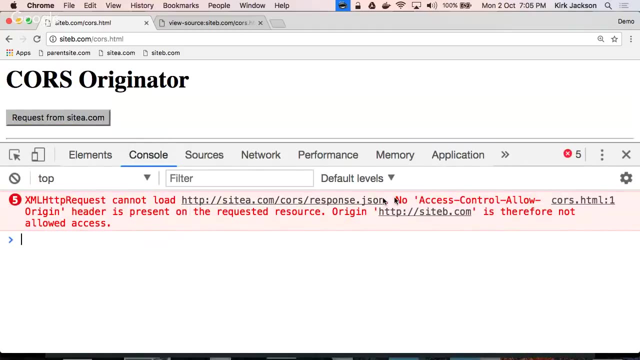 site b is now trying to request data from site a- um. so exactly the same code, except it's trying to call site a- um. that's not working and if we look in our console we'll see that site a doesn't have access control. allow origin header. 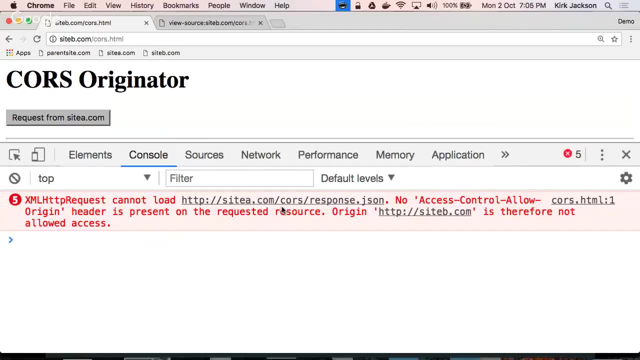 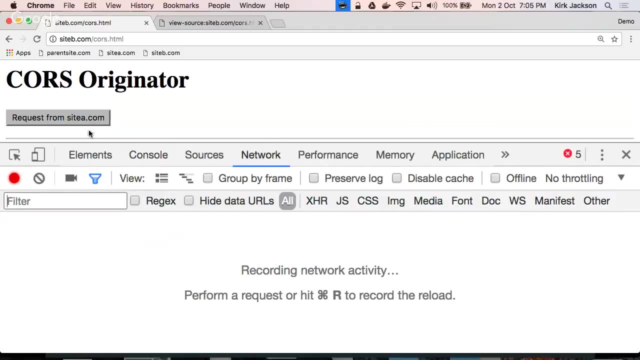 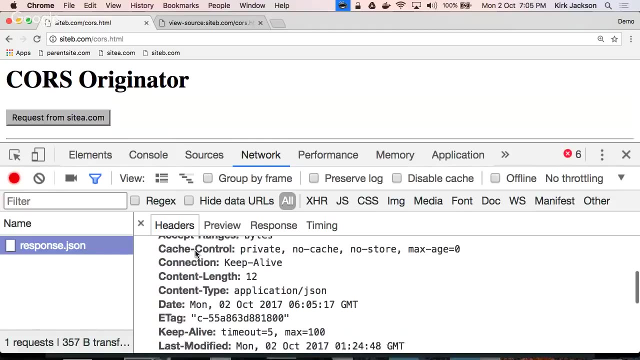 so therefore it's not allowing access. so the same origin policy that we saw earlier on is: what's blocking that and the browser is enforcing it? um, and just to just to double check, you can see that in the response headers there's not, there's not that access control. 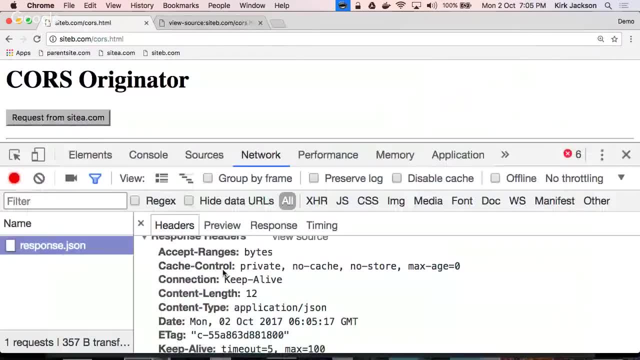 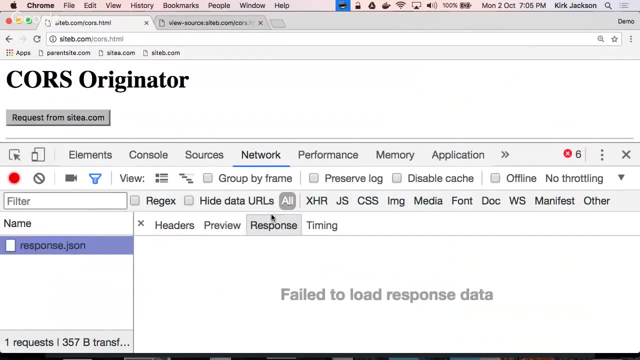 allow origin header. uh, yeah, so the the web server is sending the whole response to the browser and then the browser's not giving it to javascript. um, so you can actually see it in the developer tools. i think it's been thrown away at an early stage, but yeah. 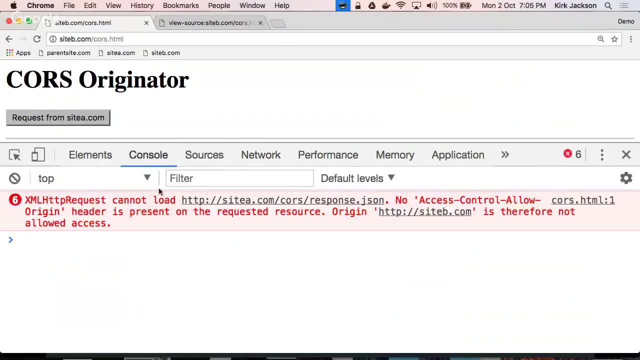 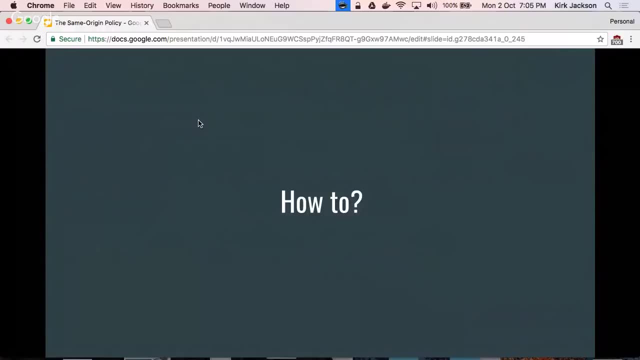 i mean, the response is traveling to the browser. um, cool. so we've seen same origin policy, we've seen how it applies to a bunch of web technologies in a mostly consistent fashion, which is, um, you can't see other people's data, but you can send things to them. you just can't. 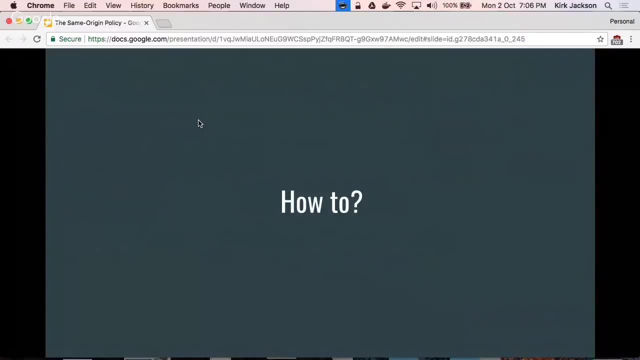 see the reply. um, we've seen two extensions to html five or an html5 that allow you to send data between frames and send data to other servers, receive data from other servers. um, and this last section is a bit of how to's. so a couple of scenarios like 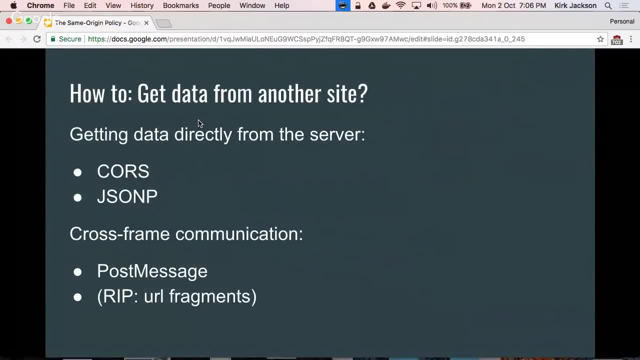 if you want to get data from another site, how do you do it? uh, we'll discuss both those ways, um xml, http requests with cause plus origin and jsonp and post message. if it's between frames. um, i put a little footnote there. there used to be a way of doing it with url. 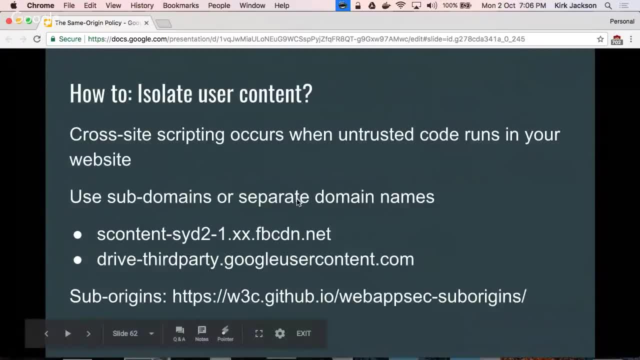 fragments, but i don't recommend you do that. um next scenario you might want to do is take some something that users have entered and put it on your web server in a safe way and, as we've seen, like if there's two pages on the same origin. 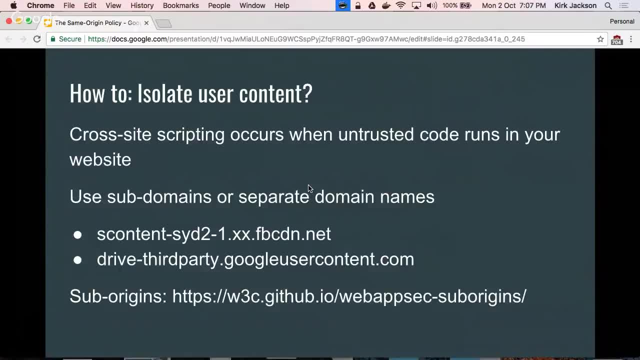 there's two pages on site a. then they can actually access each other's data um. so if you gonna take user information and put it on your website, you really don't want it to be on site a, because you shouldn't be trusting their html um or their pdfs or whatever. 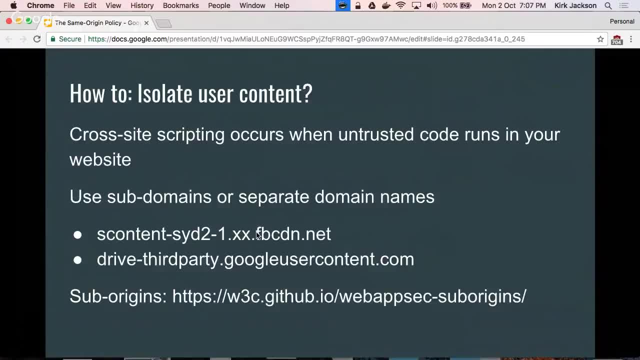 um, so what you normally do is have separate sub domains for user content. so here's what facebook and- uh, google do: they'll have different domains that they'll put user content on, and so when the users html loads or their pdf loads, it is in a different origin than facebook. 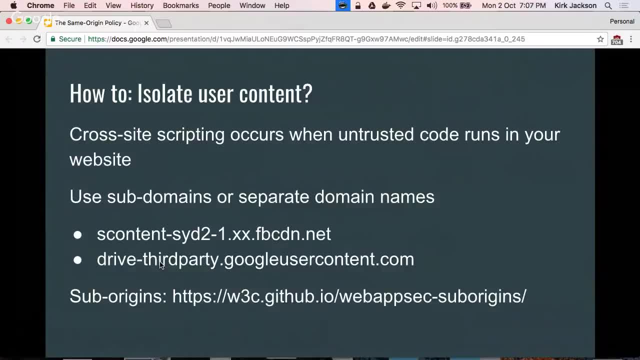 or google, so it can't access the data. um, there's an extra for experts here. there's a new spec called sub origins, which is going to let you, instead of having different domain names, have different parts of your site that can't communicate with each other. um. 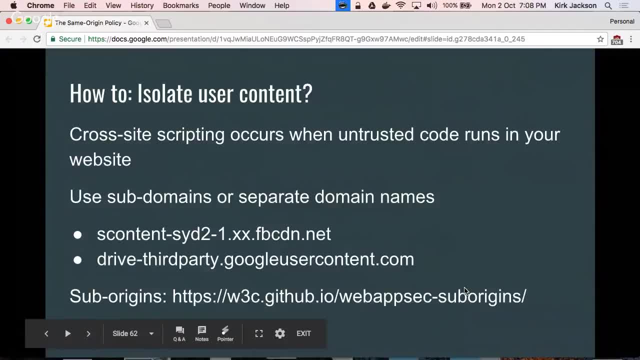 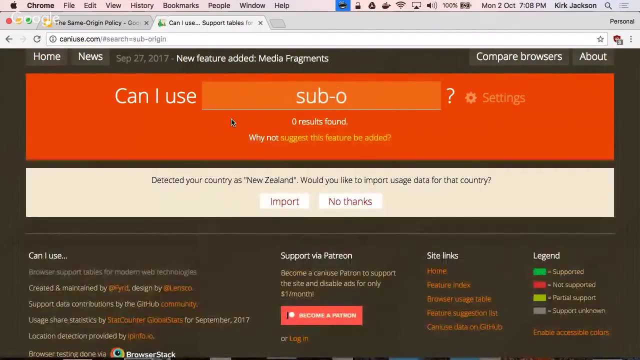 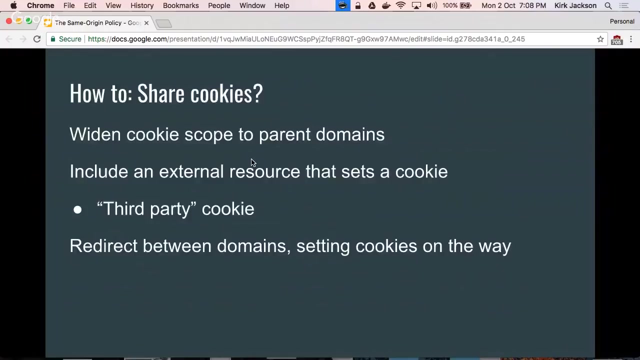 so this is sort of an extension to the same origin policy. and have a look at um. at the moment, it's only supported in chrome or firefox. um, only supported in one browser. yeah, whatever, not even on there. um cool. um, how do you share cookies between sites? um well, there's two ways. 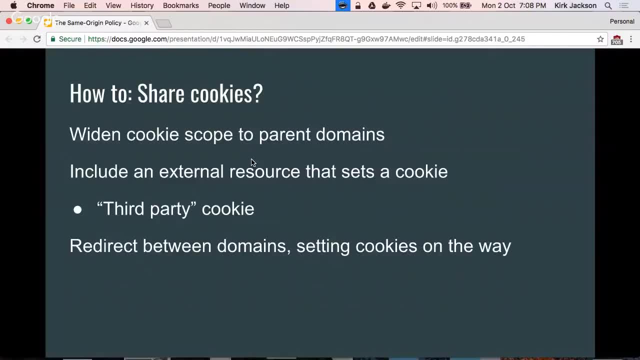 you can um widen the cookie. so instead of being mysitegooglecom, you can see the cookie for googlecom and then all the sub domains of google see the same cookie. um, you can do what ad networks do and actually set the cookie um in multiple places. so 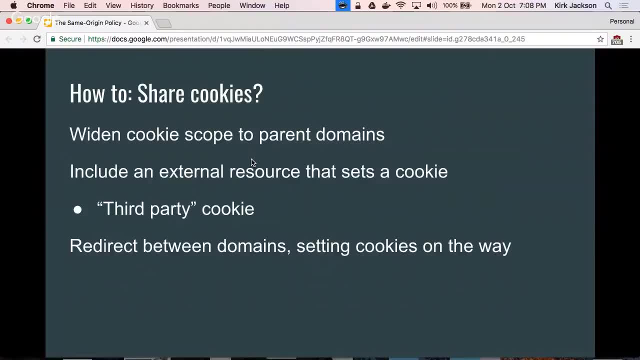 they'll like, um get you to embed some javascript which sets cookies on your own server as well as um, as well as other cookies, uh, so those are called third party cookies. pretty much evil, um, but and uh, safari in particular doesn't build in very nicely, um, or you can do what google login. 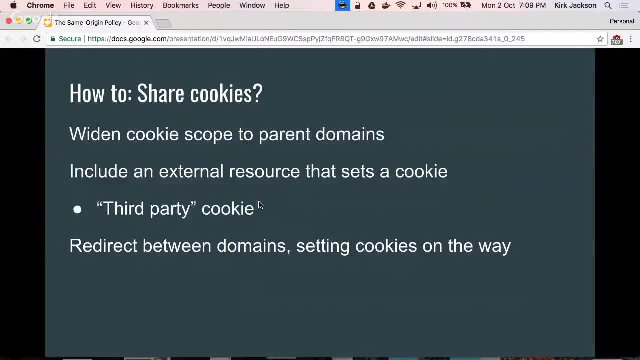 does so. when you log into google, it needs to log you into googlecom and youtubecom and bloggercom and whatever else they own um. so it'll actually bounce you through different domain names by redirecting the browser and setting cookies on the way, and when you log out it'll bounce. 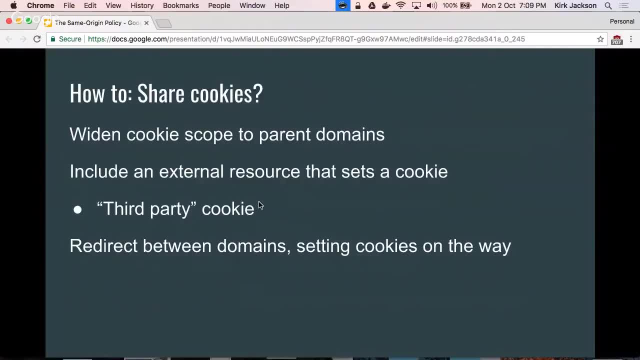 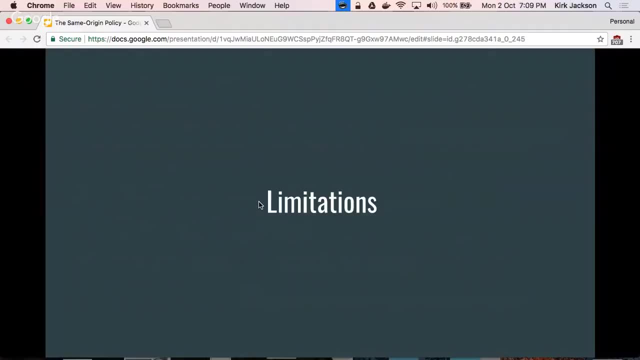 you through different domain names. uh, clearing cookies, um, so that's kind of how they share cookies. they set multiple cookies, okay, so there's a few scenarios that you can dig into. okay, so, limitations of the same origin policy. i have alluded to this heavily, so i don't 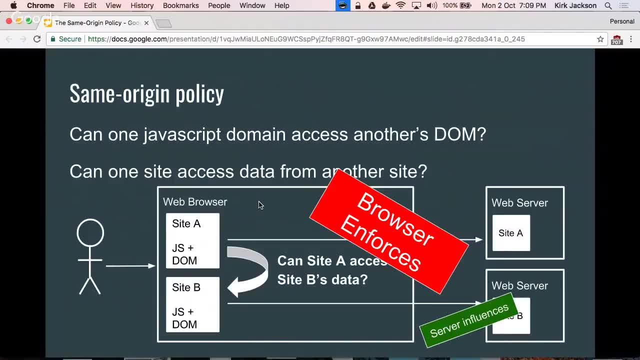 think it's a surprise that it's the browser that enforces same origin policy. um, not not really your web server that enforces it. your web server doesn't really know that the person asking for data is a web browser. um, it just has to trust the browser is going to do a good job. 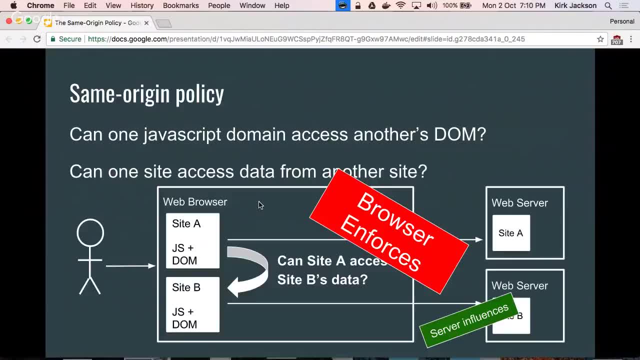 um. so where this really comes into play is if you're making an api and um, you want to have that on a different domain name from the rest of your site and you want to allow cross origin requests. you're like, well, if this is running in the browser. 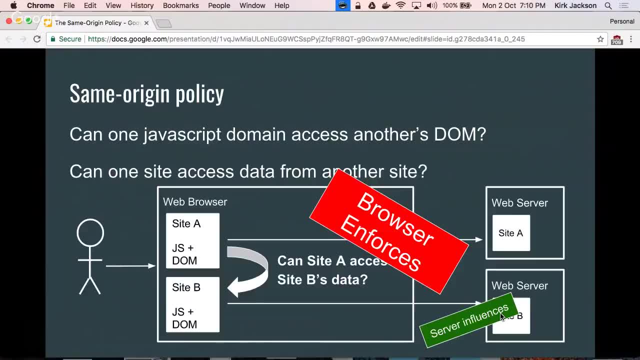 my javascript code is the only code that can access my api. but you've just put a server on the internet that'll receive requests and give data back. anyone can abuse your api by just calling it from their own server site code. they just can't call it from. 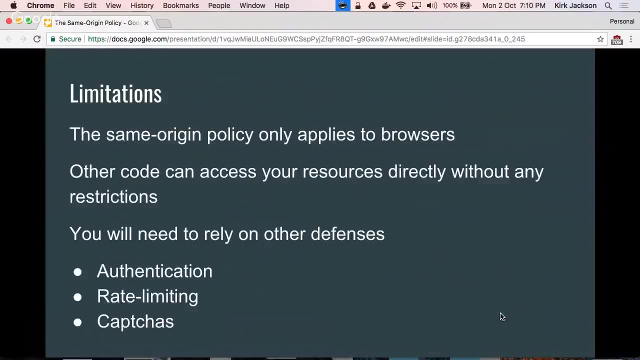 javascript. um, so, um, yeah, so basically, this stuff only applies to code running in the browser. um, if you're exposing an api or you're worried about abuse, um same origin policy doesn't protect you, um, and so you need to do things like you know, making it authenticated or rate. 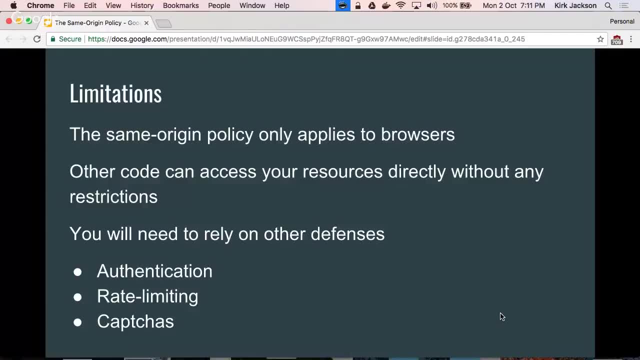 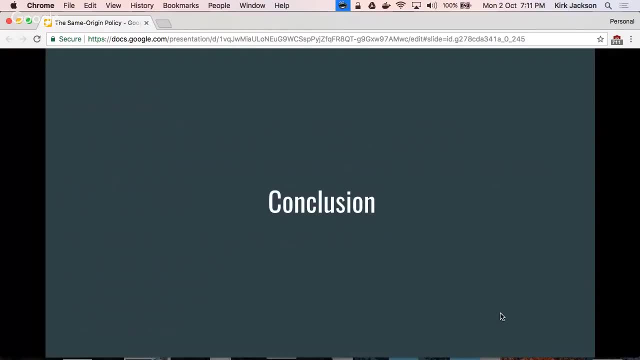 limiting or detecting bots or sticking up a capture or any of those other things that you'd normally do to try and protect an api. um cool. so, in conclusion, today we learned about the same origin policy and it's kind of like the basic underpinning of everything. 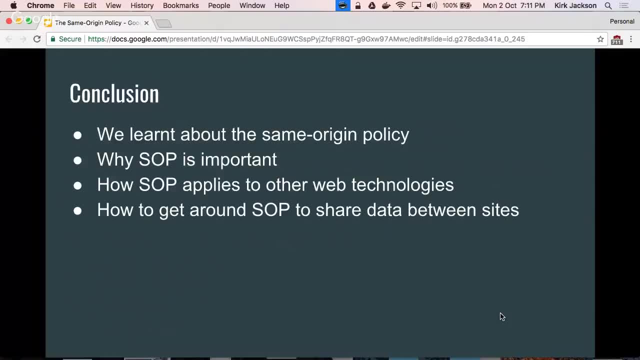 when you go and look at cross-site scripting, you'll see that cross-site scripting is kind of an abuse of the same origin policy to try and run javascript in someone else's origin. when you look at cross-site request forgery, that's an abuse of of cookies and how. 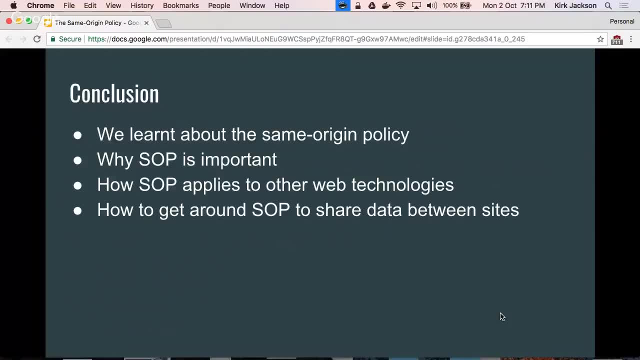 they work. so same origin policy kind of underpins everything um a lot of the web attacks that have happened, like browser flaws where browsers weren't enforcing the same origin policy correctly, or where people's websites you know where they haven't opted into some of these features. 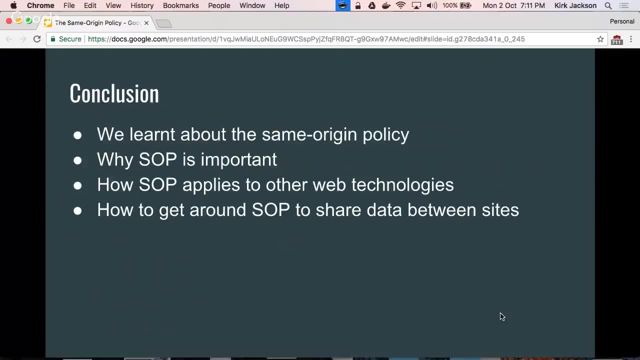 um, it all kind of boils down to the same origin policy. uh, we looked at how it applies to other web technologies, um, and how to get around it. when you actually want to share data between your sites, cool, so that's, that's the talk, um, if you 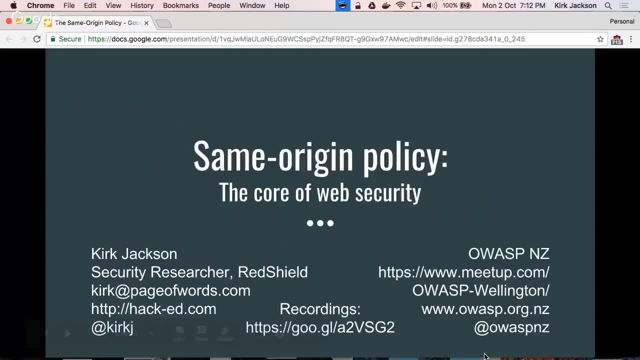 would like to uh watch recordings of other talks we've done at the oas meetup. um, there's the url down there, um, which is now obscured. um, or you can go to the meetupcom oas wellington and look there. um, drop me an email, or i've got some of my previous talks.